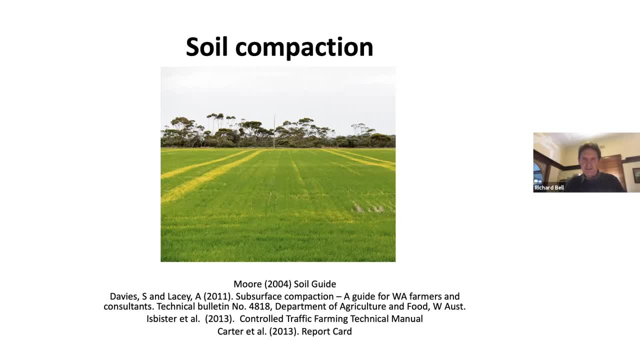 I'm going to use it, but we can go through it as fast or as slow as you like. The photograph is quite telling. This is a crop that's come up in the wheatbelt and you can see these strips where the crop is quite yellow and that corresponds with wheel tracks. So that's a really 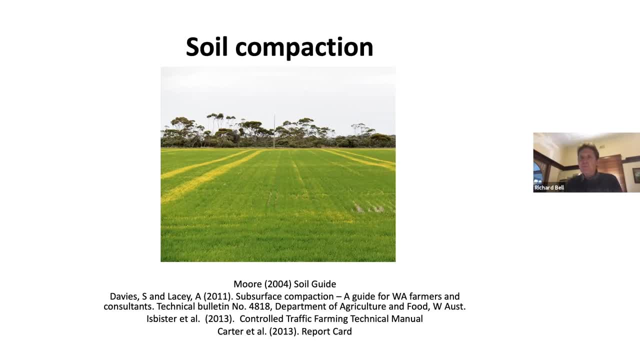 good illustration of a compaction issue in the soil and presumably where the soil is compacted under the wheel tracks. the rainfall is not infiltrating and you're getting some temporary water logging and that's what causes the crop to yellow off. That doesn't always. 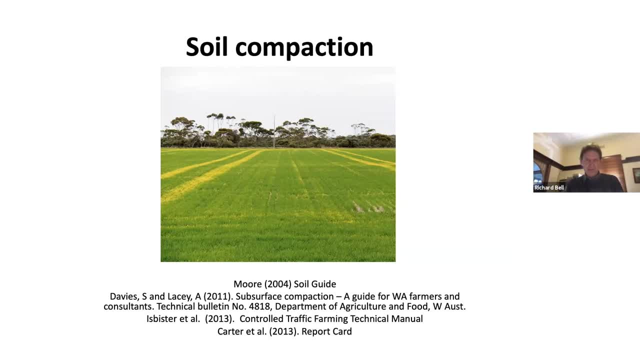 show up quite as neatly as that, but that's a visual indication of the sort of problem, that of compaction Locally. there's quite a bit of good material that is available to read up on and learn some more. There's the soil guide, which is available from DPIRD. Jeff Moore was the 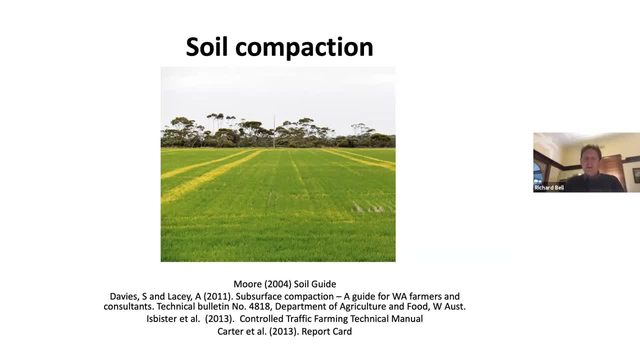 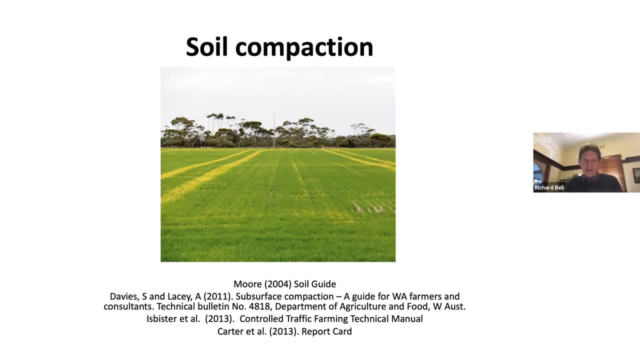 Secondly, Steve Davies and colleagues a little bit later put out a bulletin from DPIRD on subsurface compaction, so that's a bit more up-to-date. Also relevant is ISVista 2013 on the controlled traffic farming technical manual. that obviously deals a bit with subsoil compaction and DPIRD had 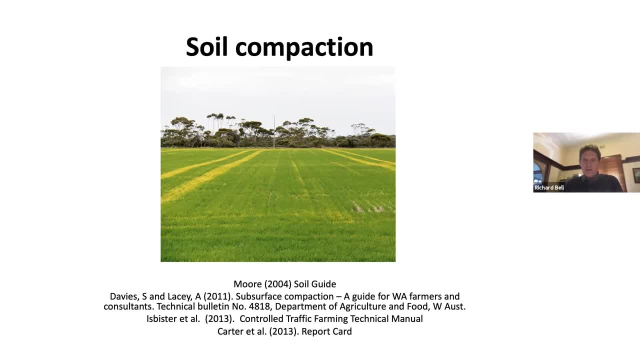 a publication called the report card in 2013, where they put together what we know about the different land degradation issues in Western Australia where they occur, how severe they are, and there's an article in that on subsoil compaction, led by Dan Carter. 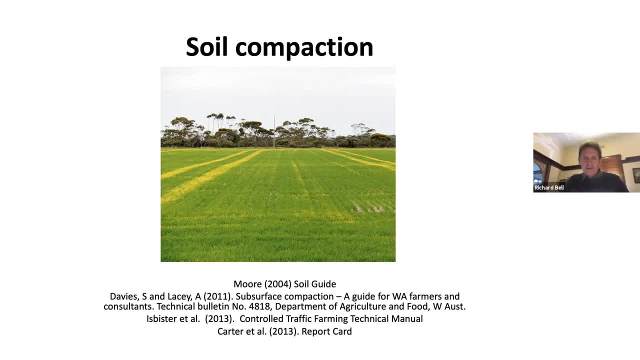 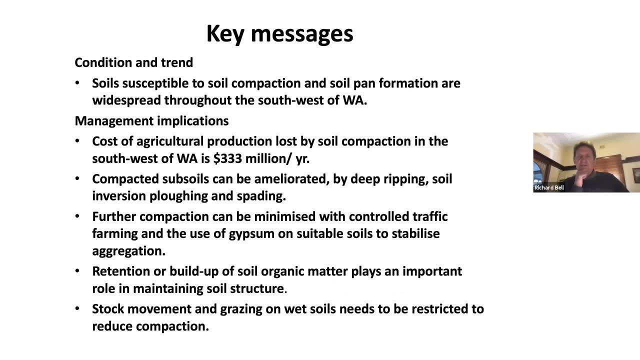 So what I'm going to present draws from that, those sources. So the key messages is that in the West we do have soils that are quite susceptible to soil compaction and to pan formation, And it's been an issue around for the last 30 years or more that we've been aware of. 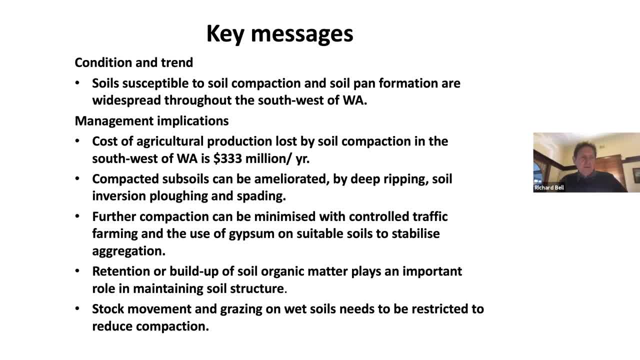 And it is important Because the estimated loss of crop production is in the order of 330 million dollars per year from that. But there are technologies that have been developed: Deep ripping has been around for quite a long time and more recently the inversion plowing. 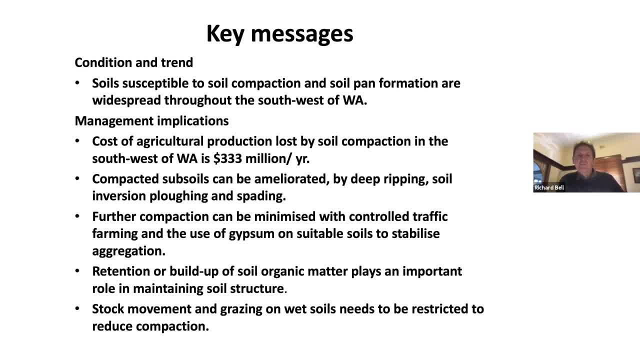 technologies have become popular as well as spading. So they're engineering Treatments to try and overcome compaction and they're obviously reasonably expensive. Importantly, with the spread of controlled traffic, we now have technologies to minimize the recompaction, Because without controlled traffic recompaction is going to occur within the space of another. 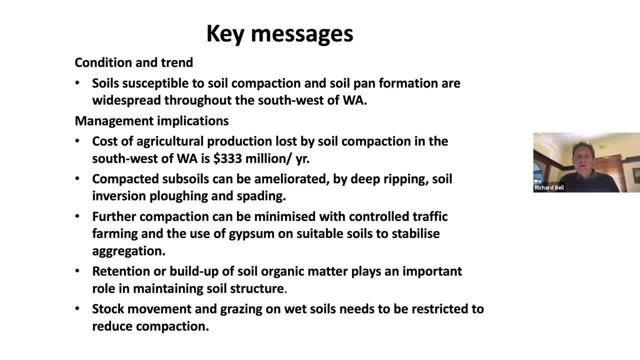 two, three, four years. So it's not a permanent solution, It's only a temporary solution. On clay soils there may also be some role for gypsum in trying to improve and stabilize soil aggregation, But soil structure and compaction is a process that damages soil structure. 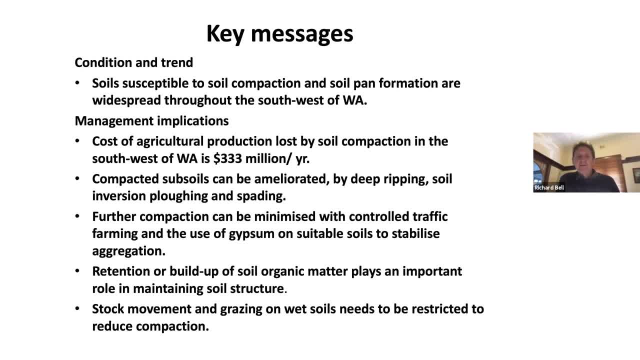 Soil structure is very dependent on organic matter. So whatever we can do that helps to build up organic matter And the soil retain organic matter in the soil plays an important long term role in resisting the effect of soil compaction that is, making the soil resilient to that. those forces causing 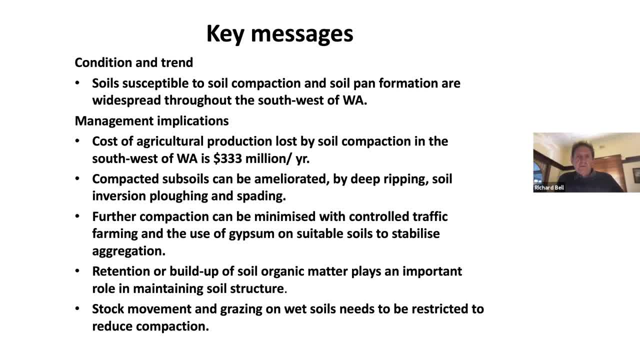 compaction, and a lot of what we deal with in relation to compaction is on cropping soils, But of course it is an issue in horticulture as well, In livestock farms or in mixed farms where you got stock movement and grazing and particularly 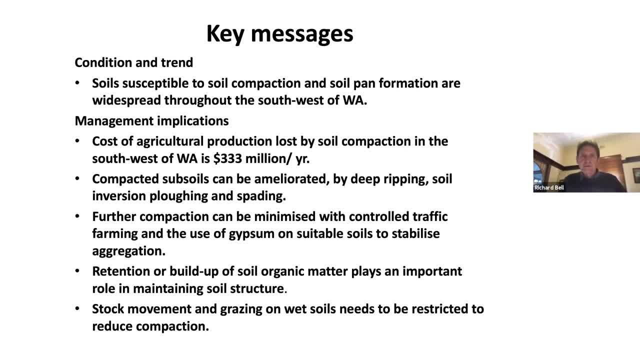 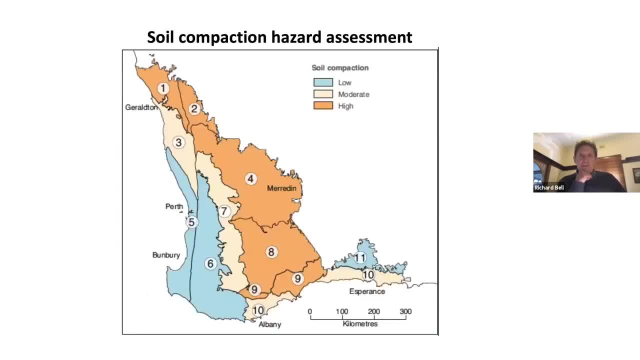 in the winter That can also be a significant factor causing compaction, because the soils are wet From Deep Herd. they have put out this hazard assessment for compaction and what it shows is that in the No No No Northeastern, eastern, southeastern wheat belts are the areas where large proportions of the landscape are susceptible to compaction. 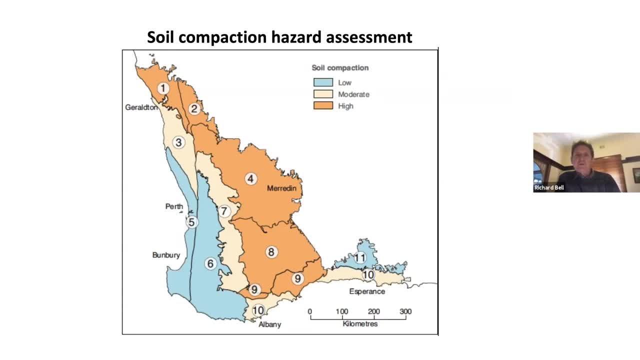 Other parts of the southwest which have moderate or low hazard. it doesn't mean that compaction is not of any concern. It just means a smaller proportion of the landscape is likely to be affected, as opposed to the areas that have high hazard. 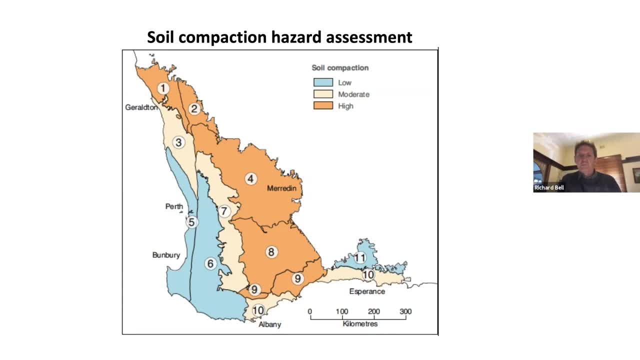 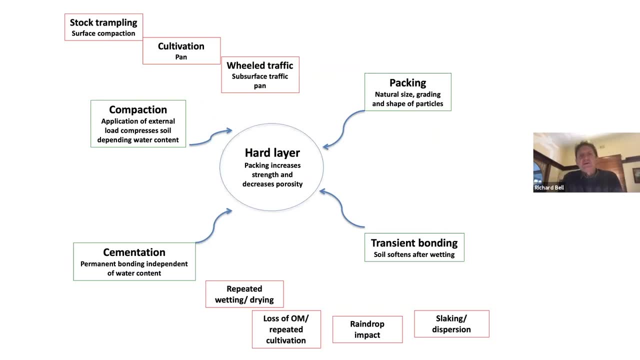 And that's just related to landform. When we talk about compaction, it is broadly within the context of hard layers in soils, And that's a bigger topic than just compaction, because we know that lots of soils, even under native vegetation, can be quite hard. 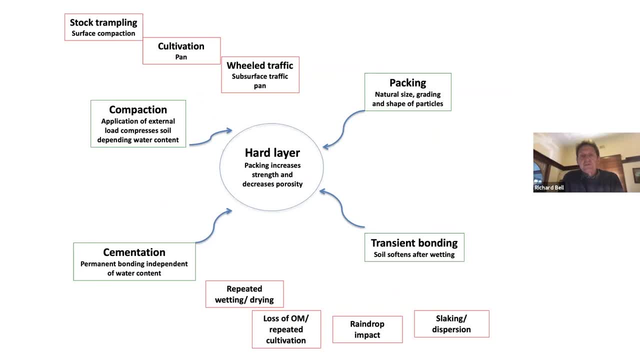 So lots of native soils have very dense subsoils with extremely high bulk densities in the subsoil. So, putting this into context of hard layers, hardness comes from packing, So just the way in which the sand, silt and clay packs together. 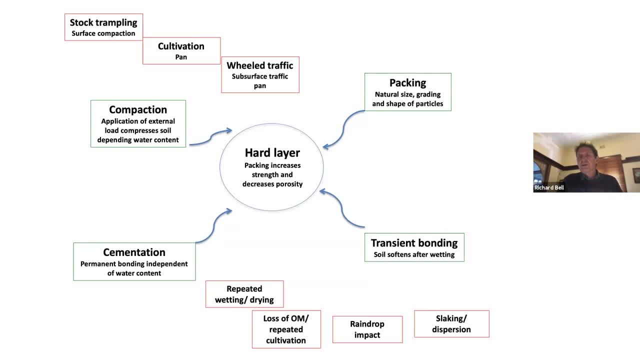 So if you've got the right combination of sand and then silt that fits into the pores between the sand and then clay that fits in the smaller pores, then it can all bind together into a hard packing or hard setting type of condition. 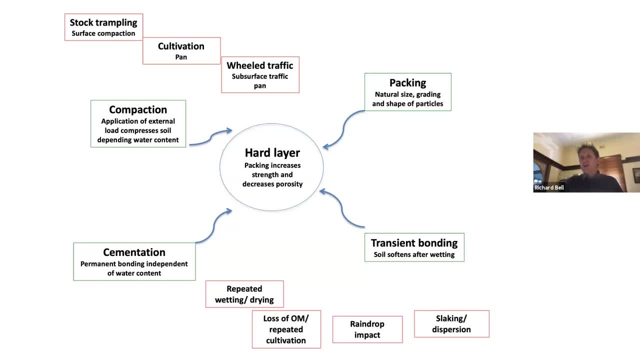 That can be exacerbated by transient bonding. So when the clay, sand and silt pack together, they tend to bond together. But some of that is reversible. when the soil rewets It softens again And I think most of us who have worked out in West Australian Wheatbelt have seen soils like that. 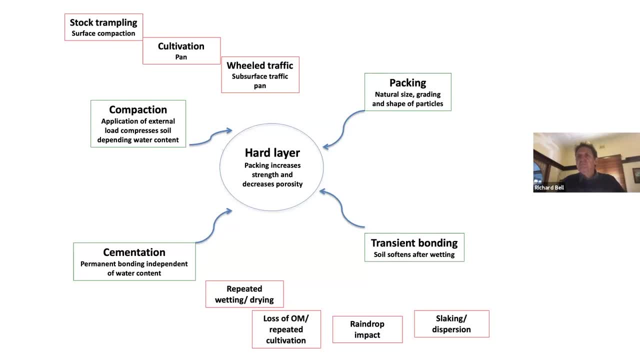 and probably also in Victoria. Soils that are rock hard in summer when they're dry, And then as soon as they wet up they start to soften. There's also cementation, So this is where the sand, silt and clay are more permanently bonded. 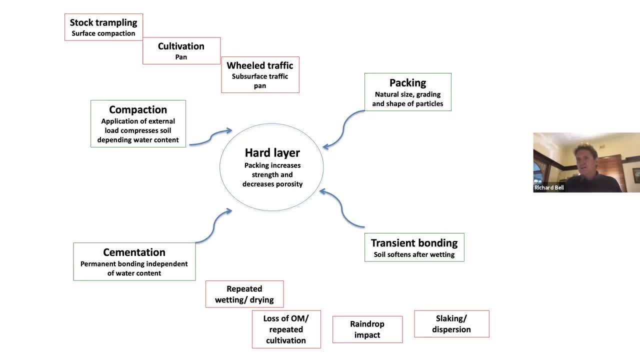 They're bonded together through compounds like iron oxides, aluminium oxides and silica, And that might be expressed in a silcrete pan, for example, which you often find in duplex soils Just at the top layer of the duplex B horizon. 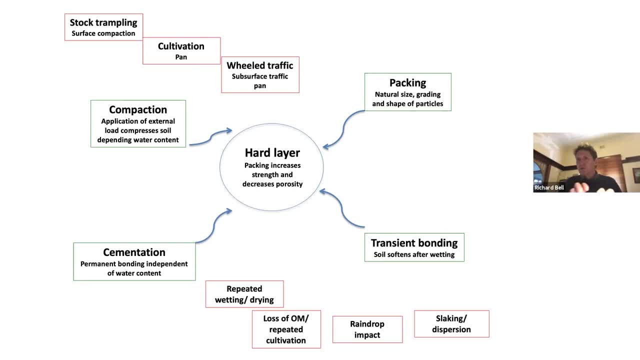 You often get quite a hard layer there from silcrete that is bonded together, the clay particles. So that type of permanent bonding is there, regardless of whether the soil is wet or dry. So those are natural features. Also we've got other natural processes that cause hardening of the surface. 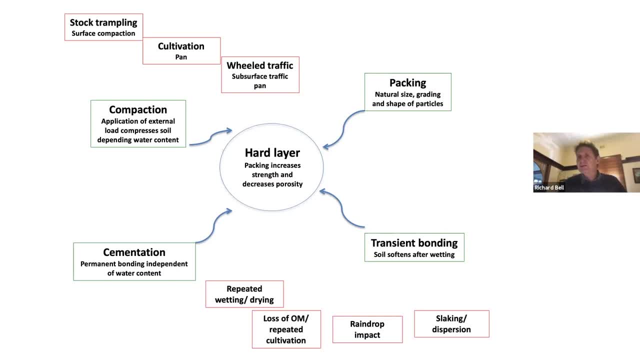 There's what we call slaking and dispersion. Slaking is a tendency of all soils when they wet up, Because when you've got a dry soil and water falls on the surface and it starts to soak in, water starts to penetrate into the peds. 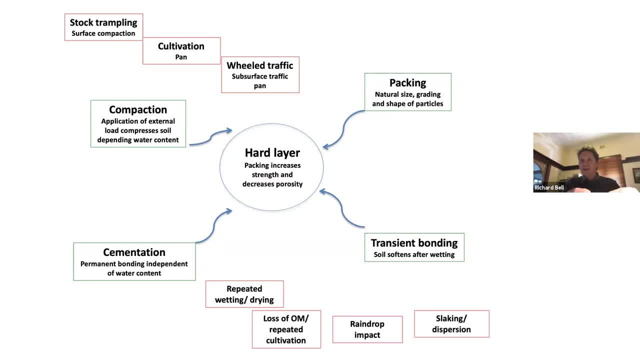 And if there's any air trapped in those peds. as the water soaks further and further into the ped, it compresses the air that's trapped inside it And, in some non-resilient soils, eventually the ped explodes. The force of the pressure of the air that builds up within the ped is so strong that it just causes the the ped to collapse completely. 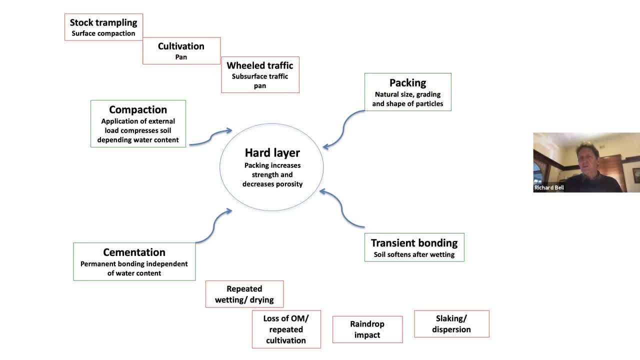 And that's what's called slaking. So that commonly happens on soils when they wet up with the first winter rains, And that's often expressed in a layer that's perhaps a few millimetres, five or six millimetres thick. So that's often expressed in a layer that's perhaps a few millimetres, five or six millimetres thick. So that's often expressed in a layer that's perhaps a few millimetres, five or six millimetres thick. 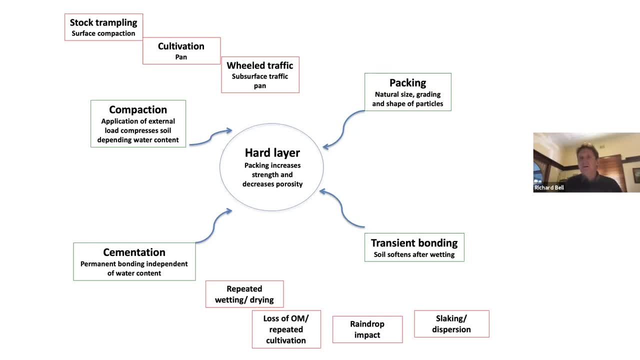 Which, when it dries, forms a hard crust on the surface, Which, when it dries, forms a hard crust on the surface, Which, when it dries, forms a hard crust on the surface. Dispersion is a bit different. that's related to sodicity in the soil. 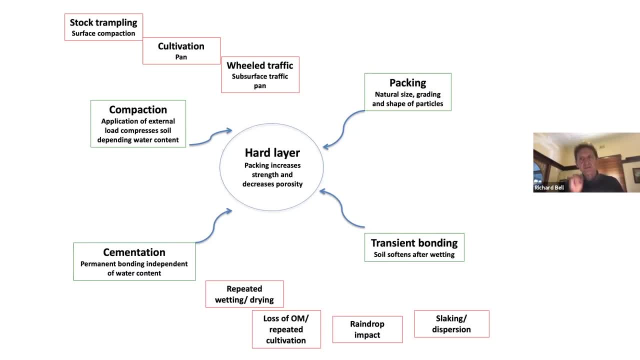 Dispersion is a bit different. that's related to sodicity in the soil. Dispersion is a bit different. that's related to sodicity in the soil. So those soils, when they wet, they tend to disperse because of the influence of the sodium. 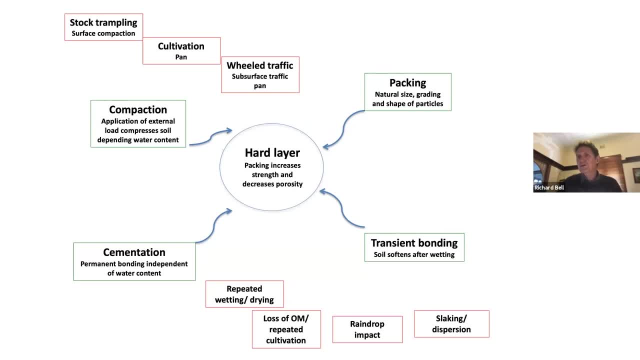 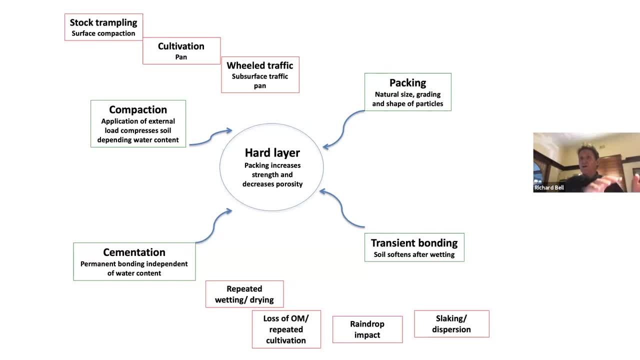 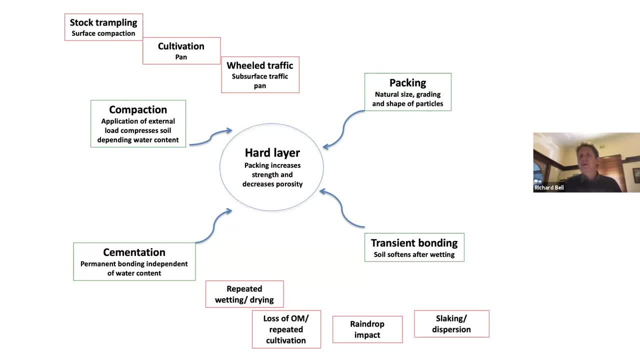 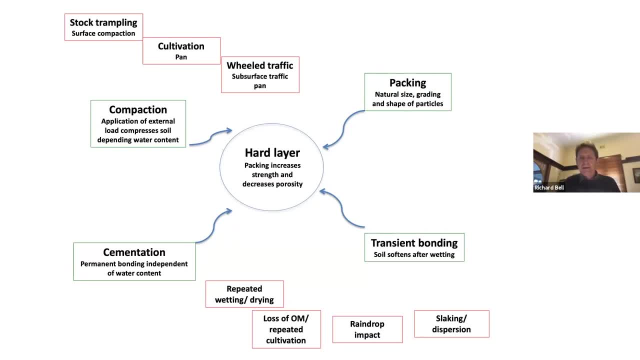 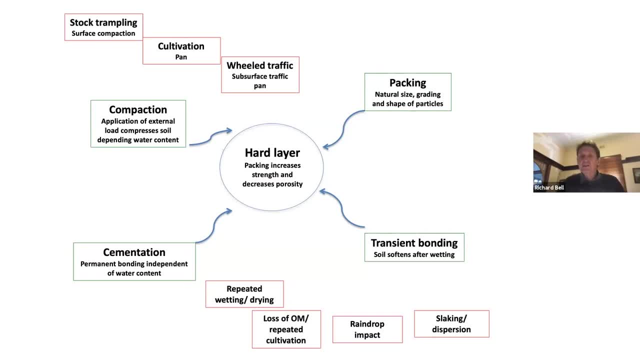 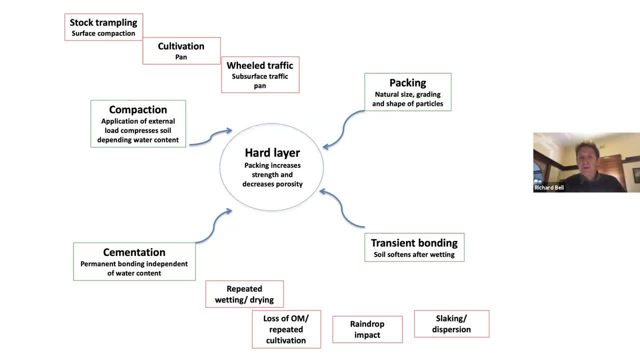 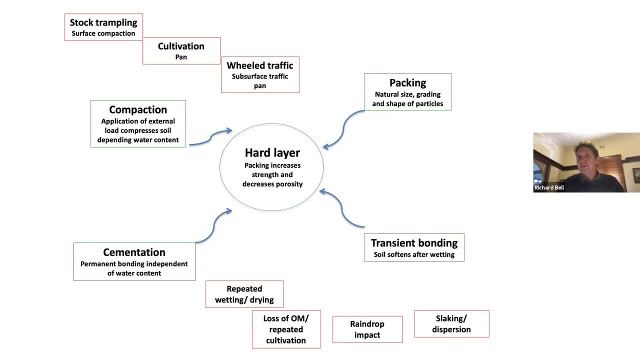 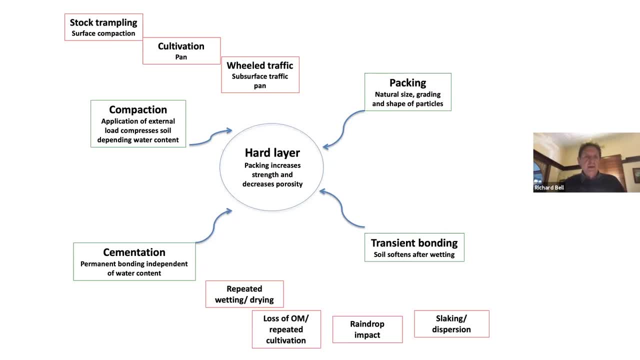 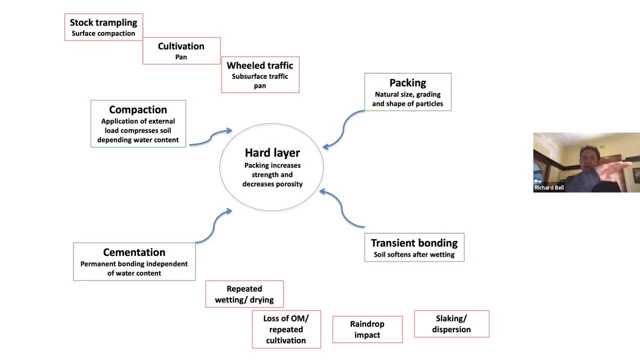 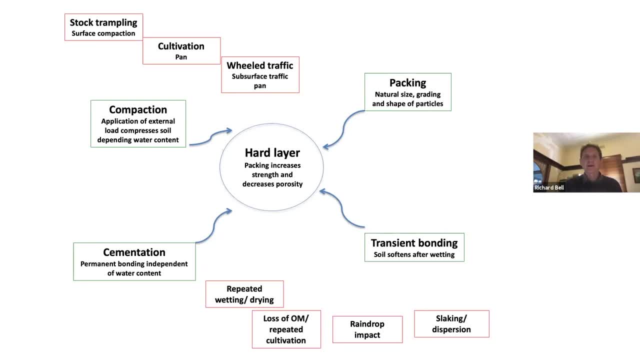 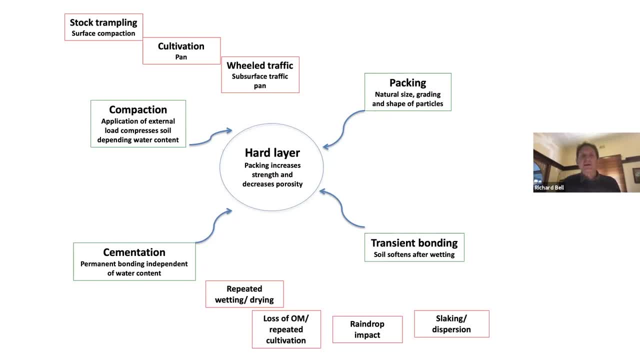 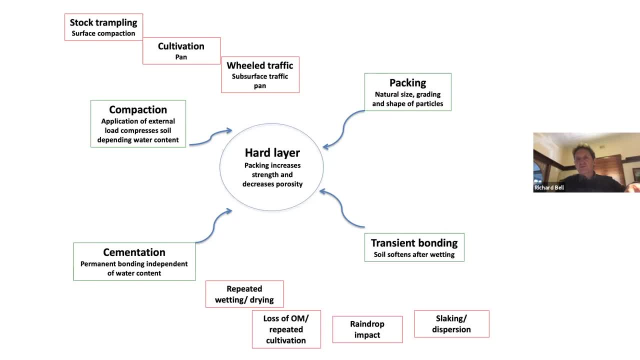 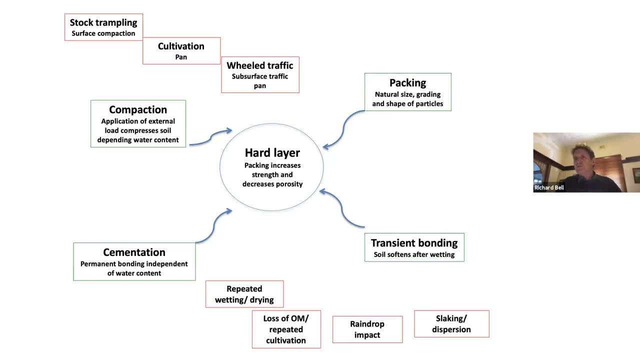 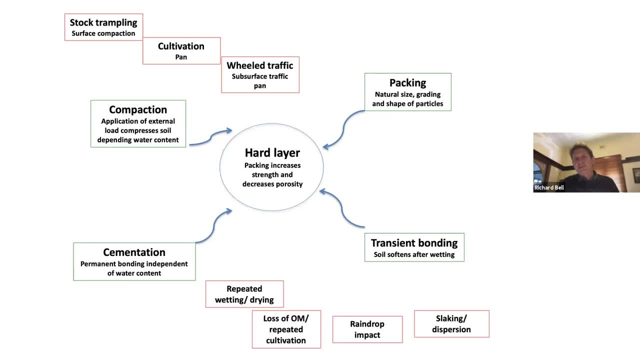 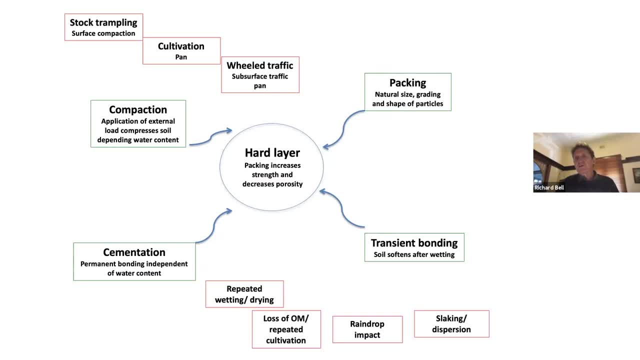 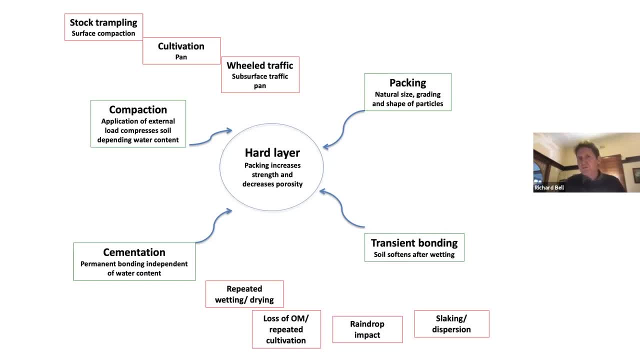 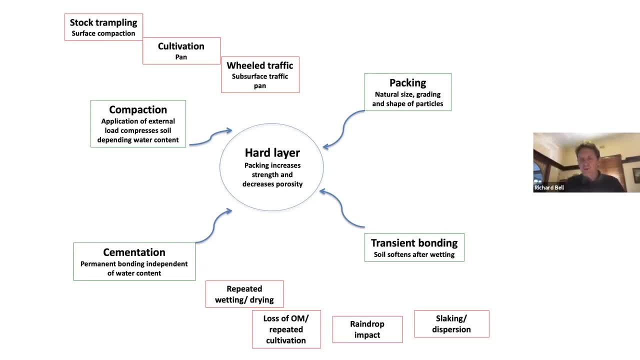 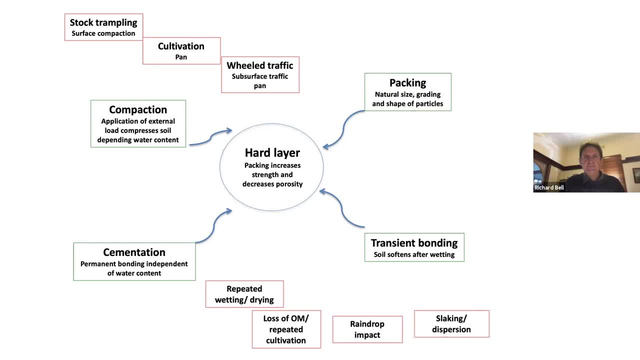 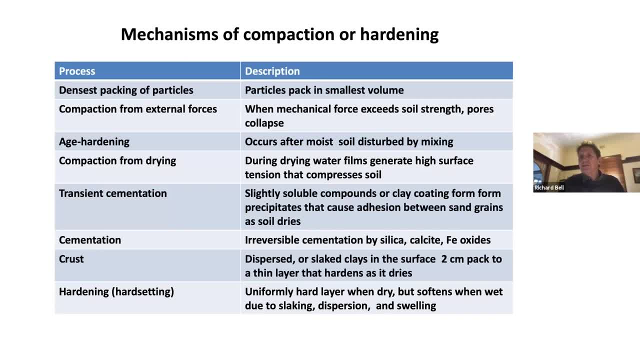 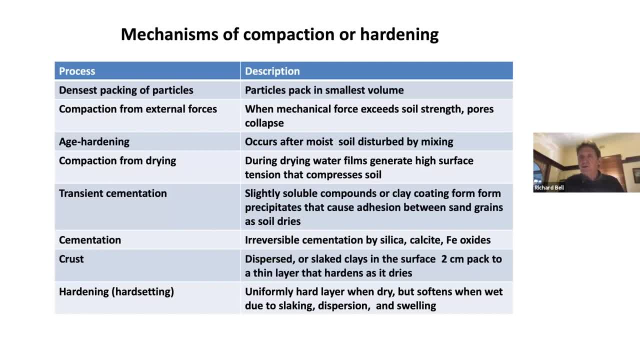 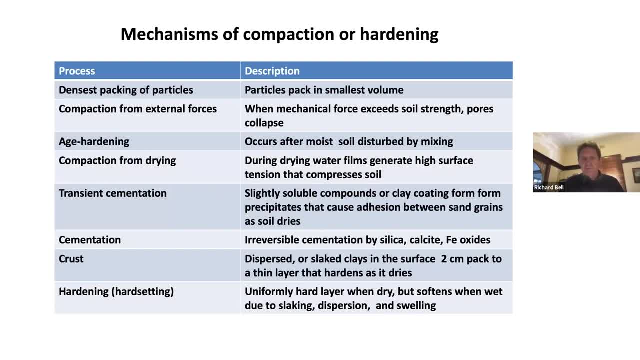 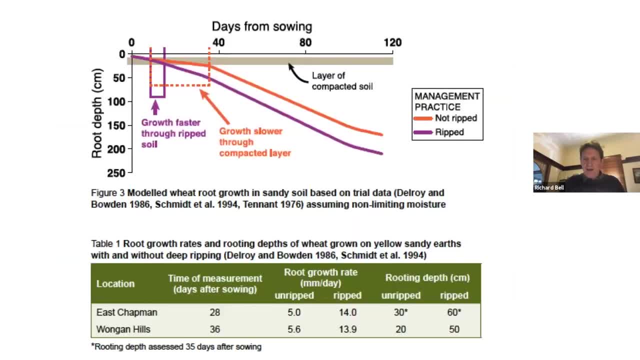 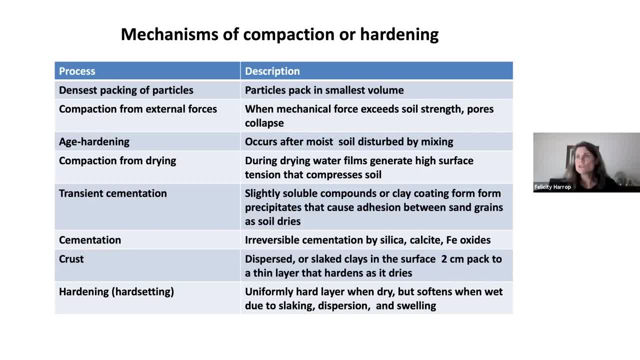 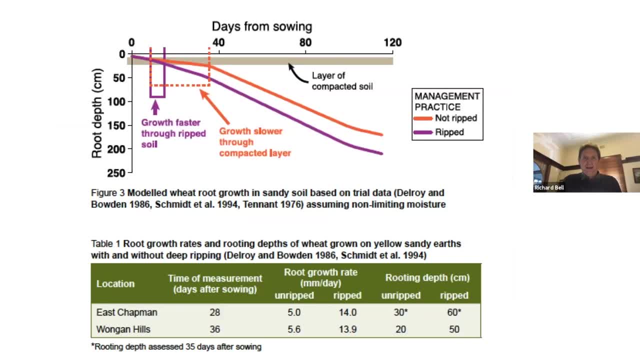 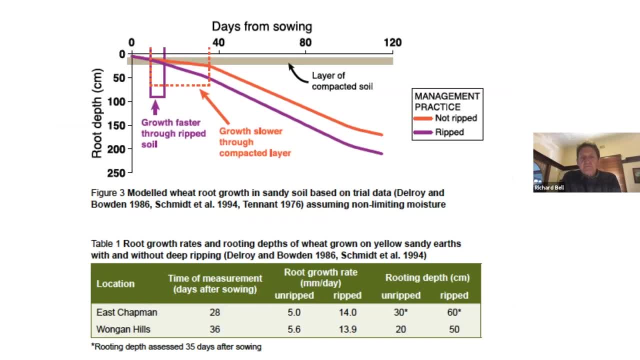 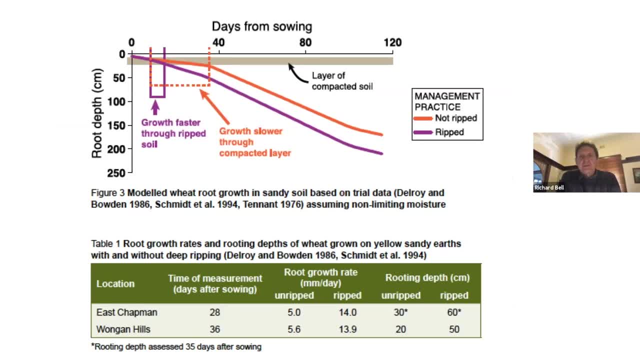 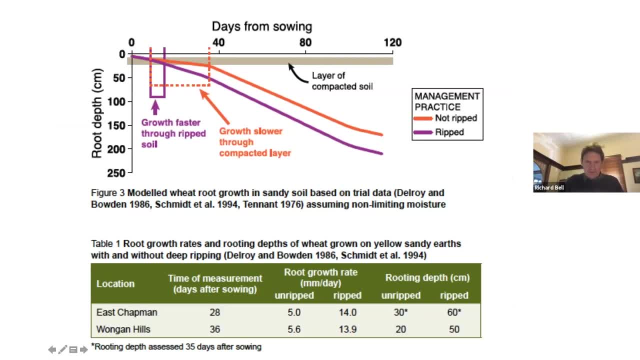 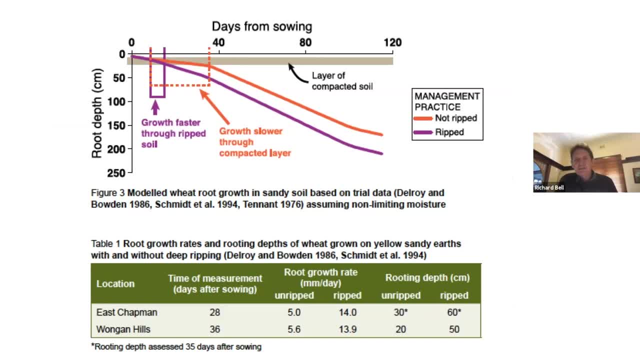 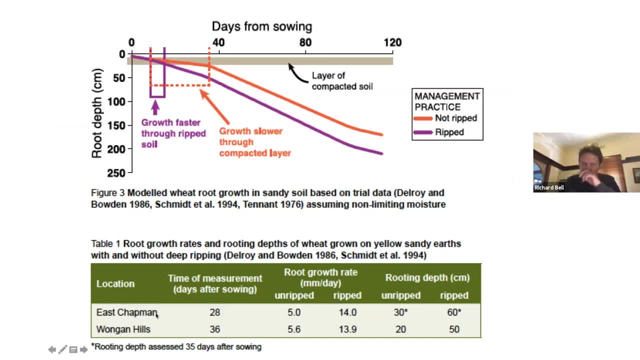 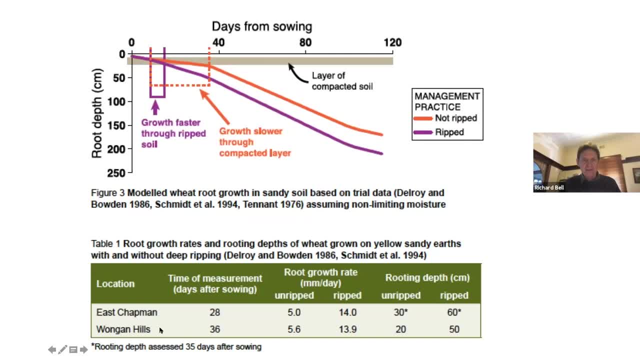 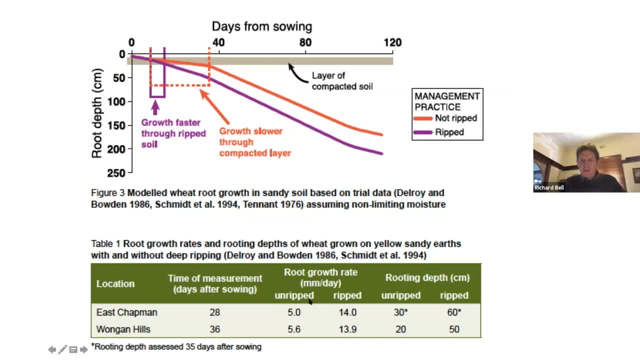 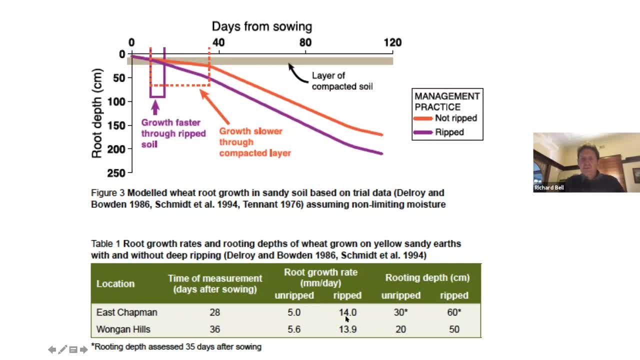 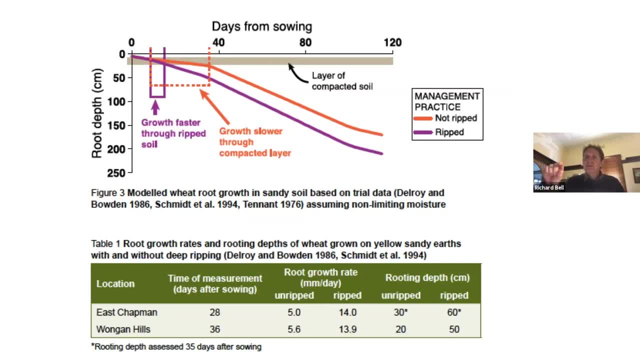 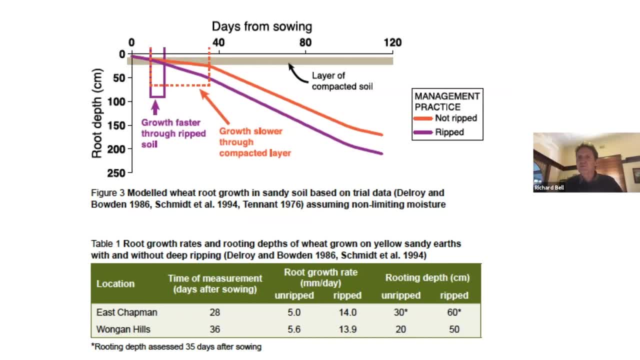 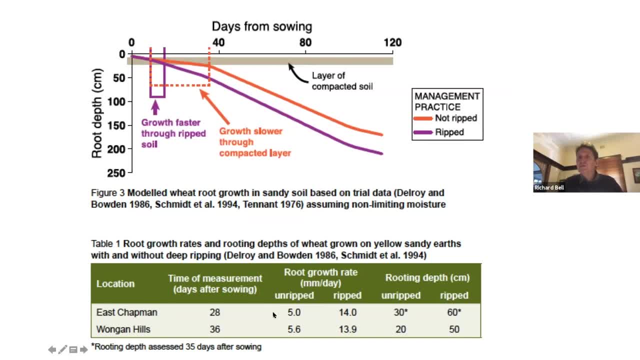 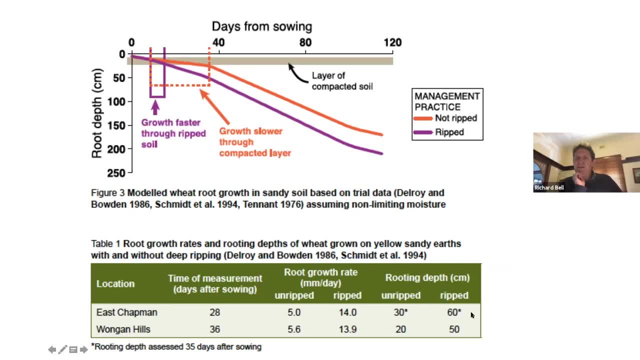 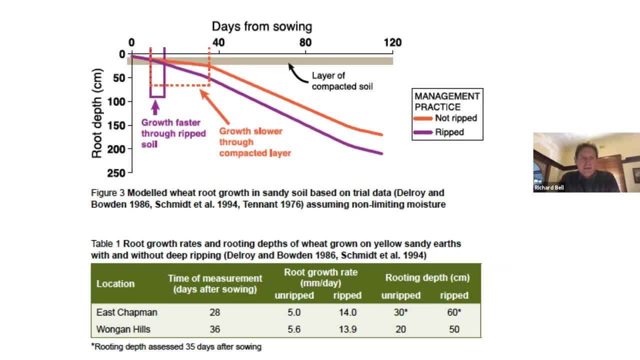 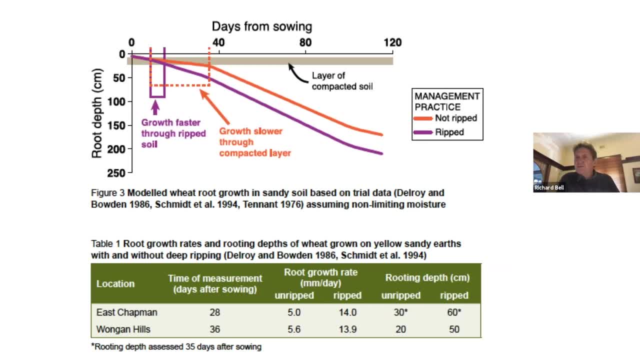 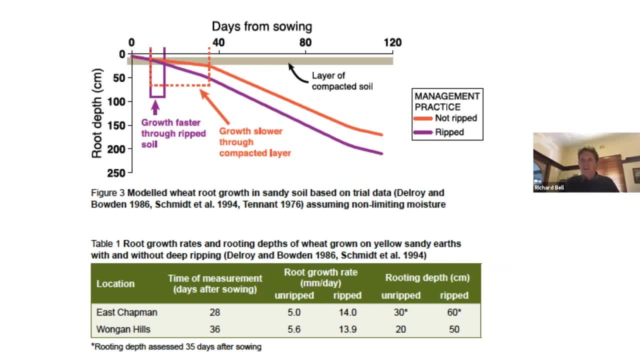 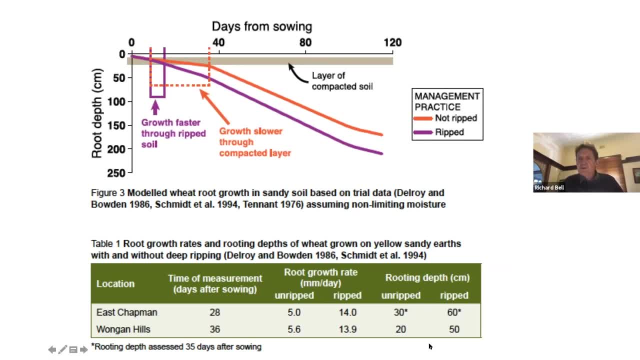 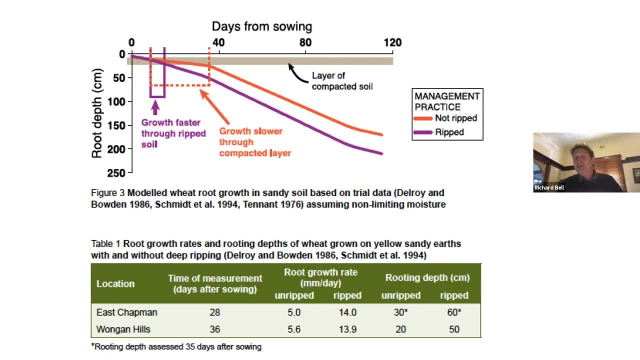 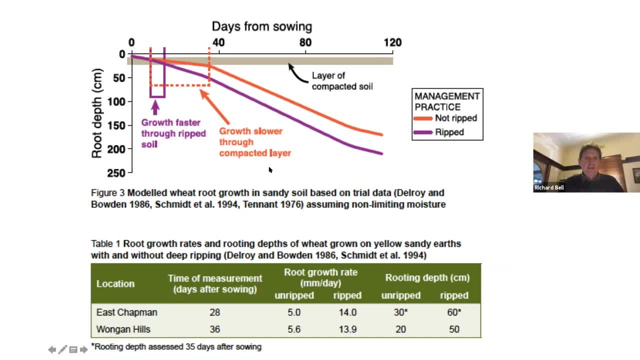 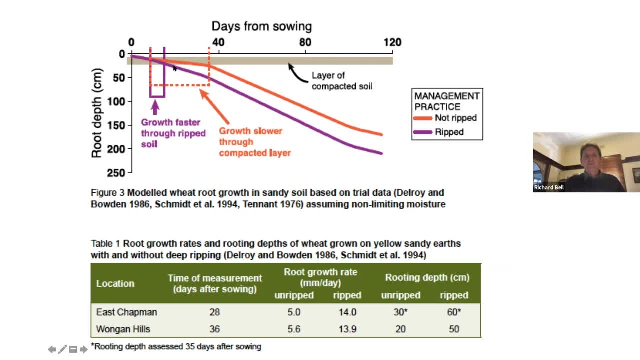 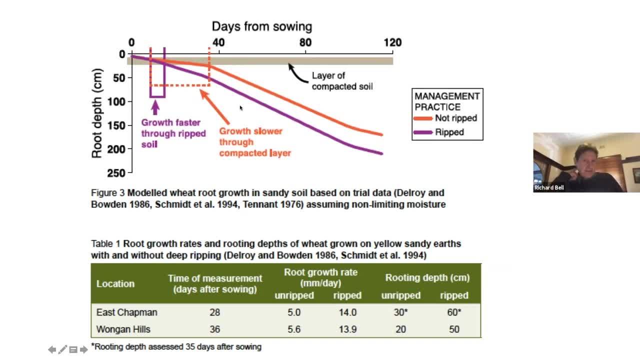 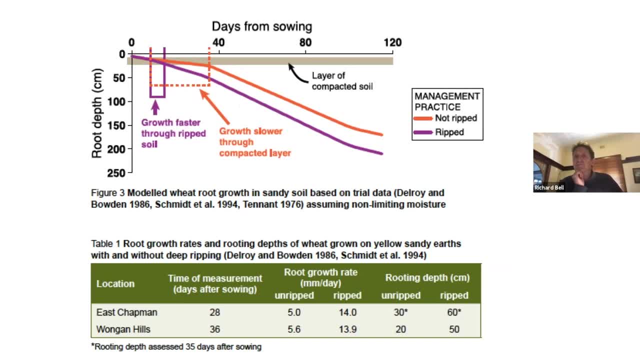 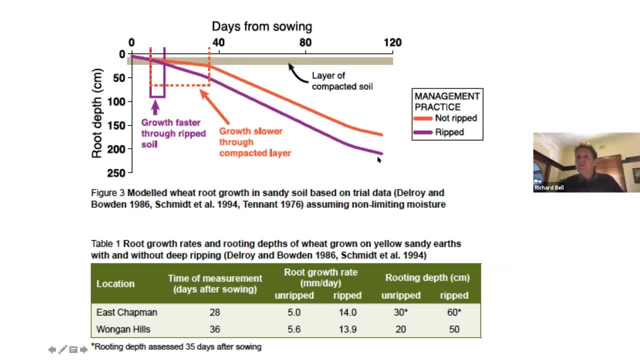 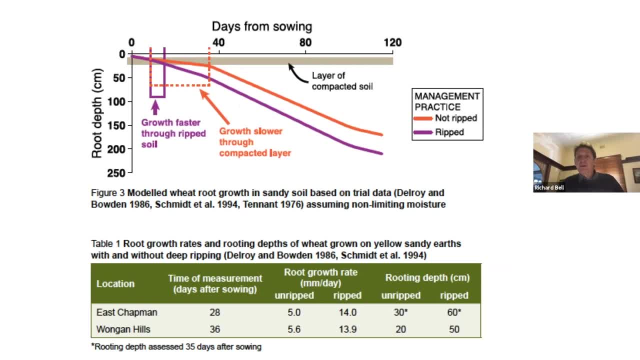 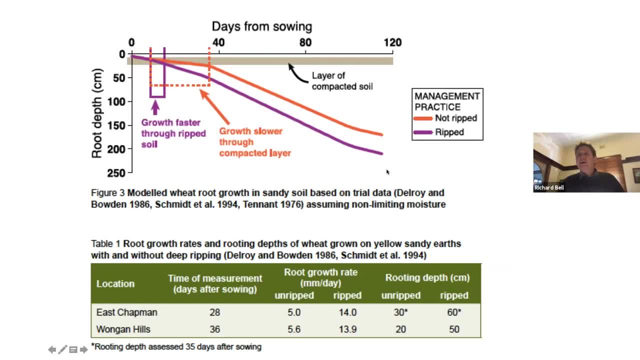 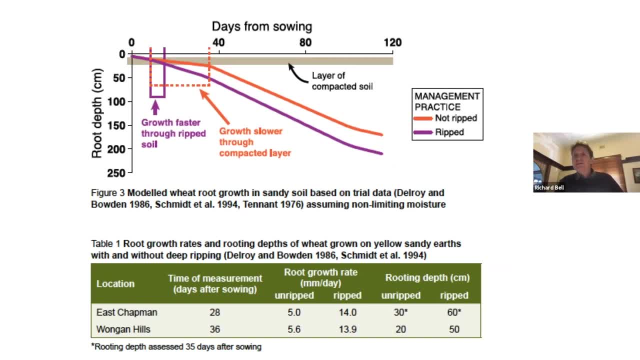 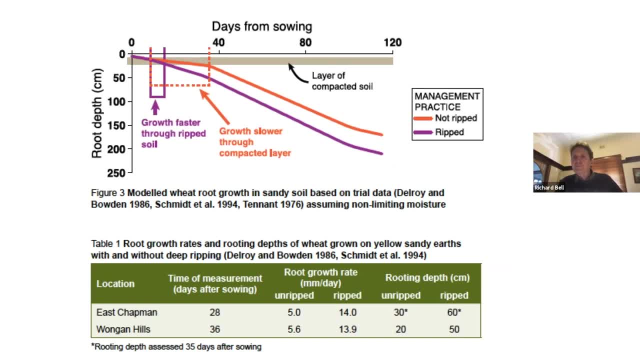 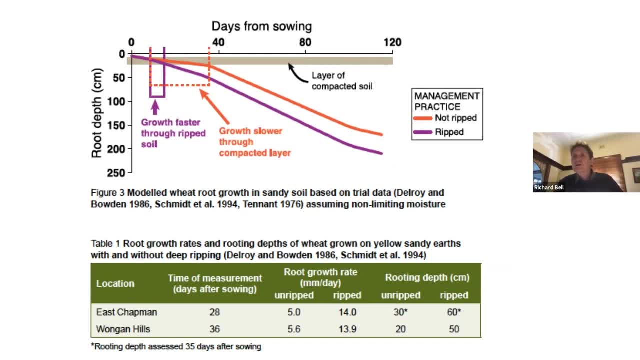 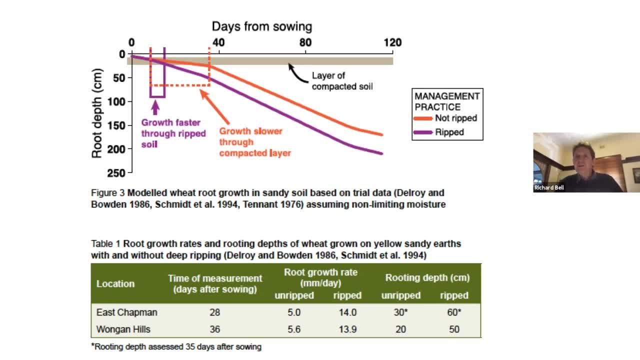 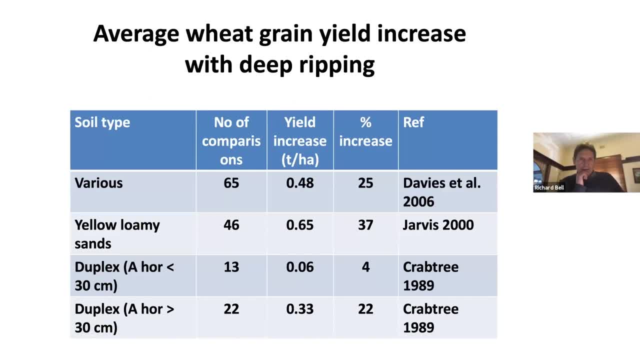 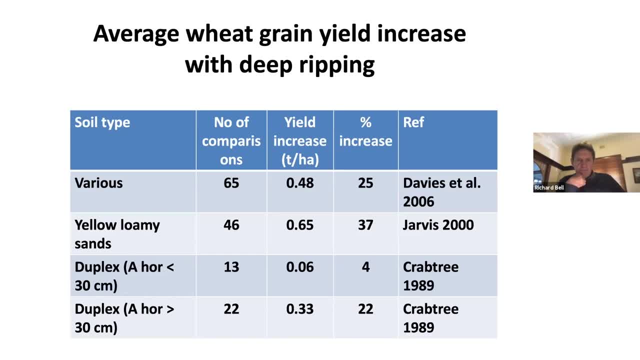 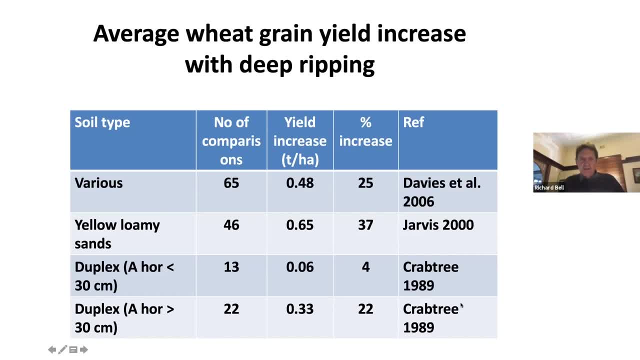 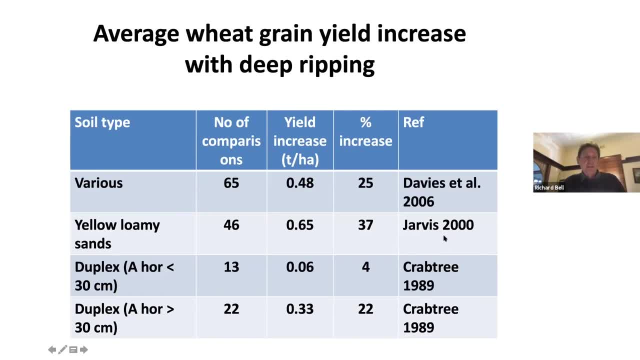 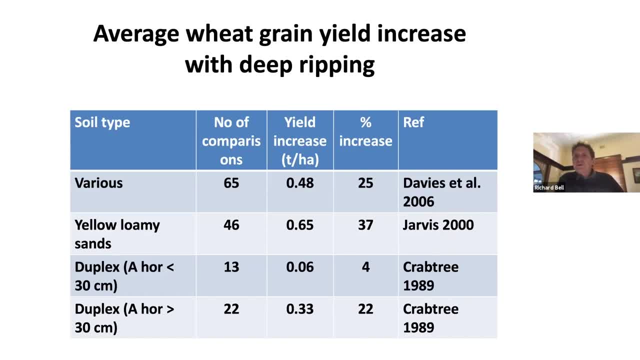 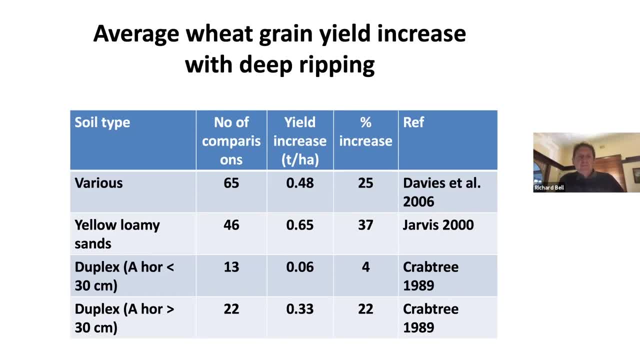 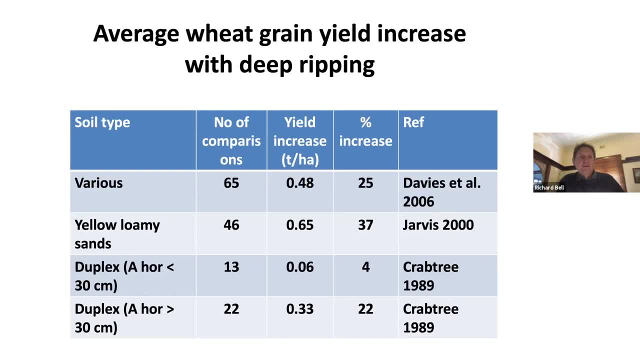 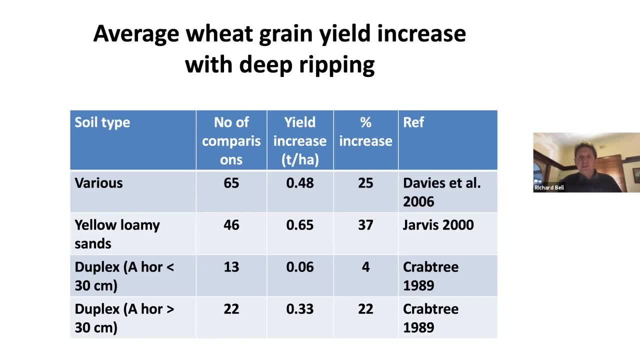 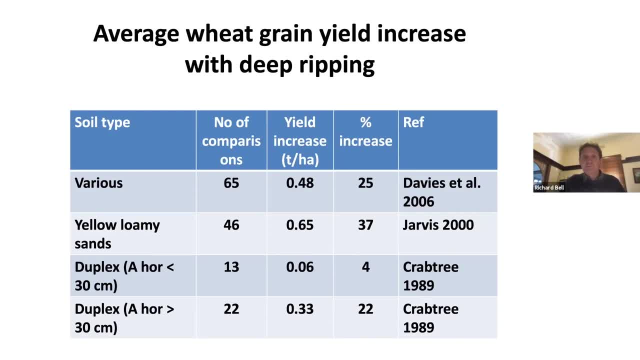 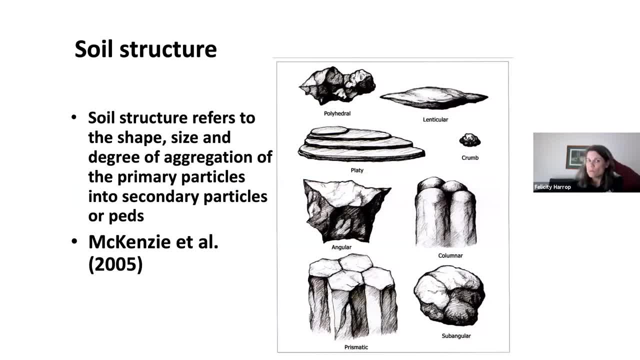 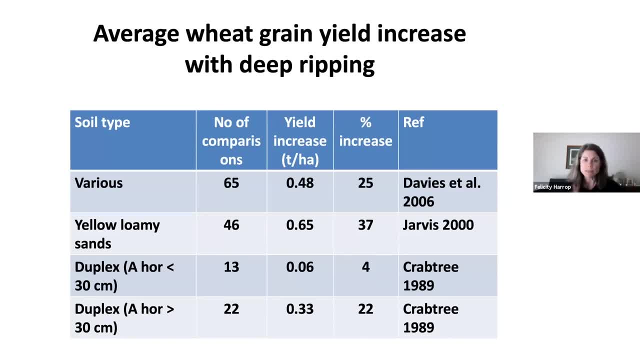 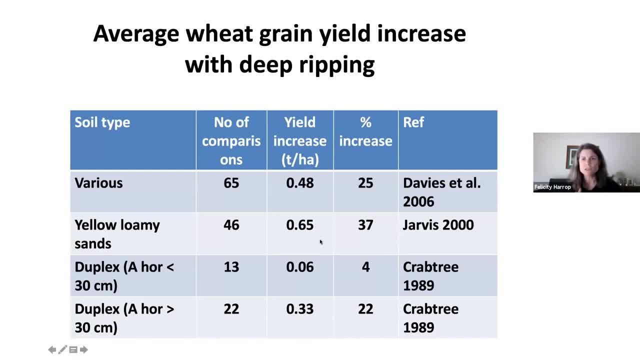 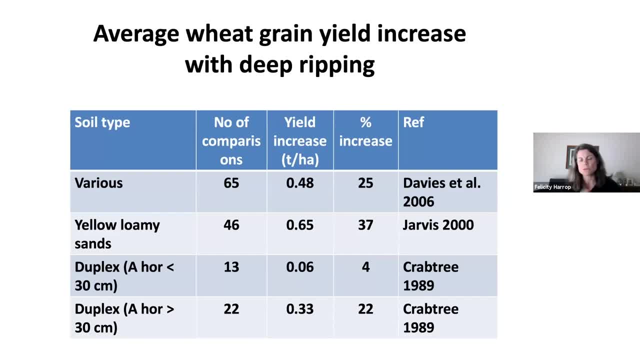 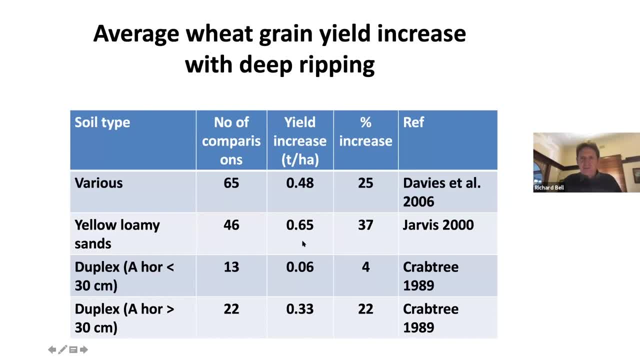 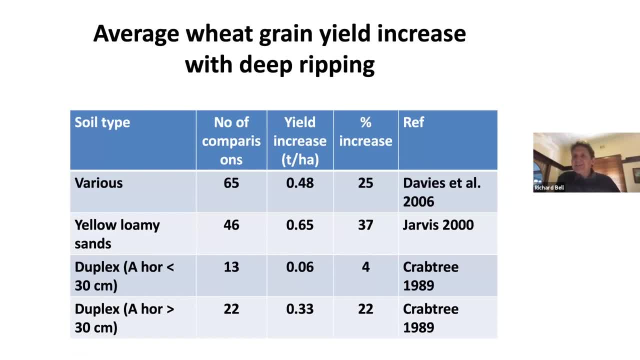 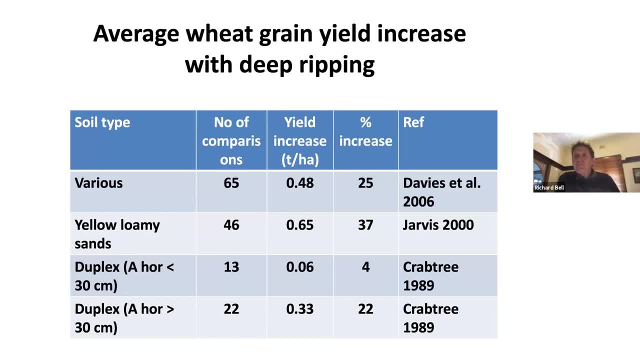 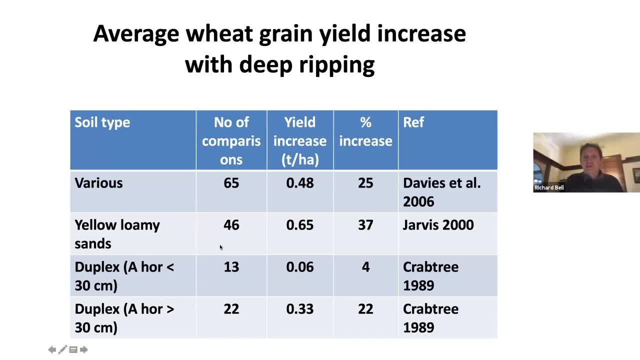 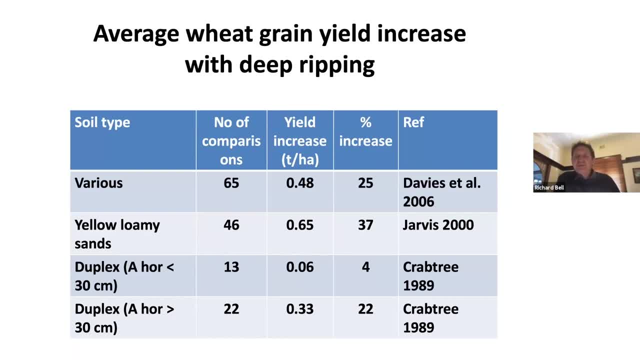 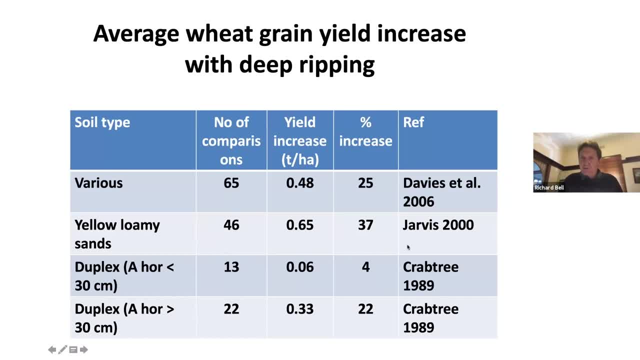 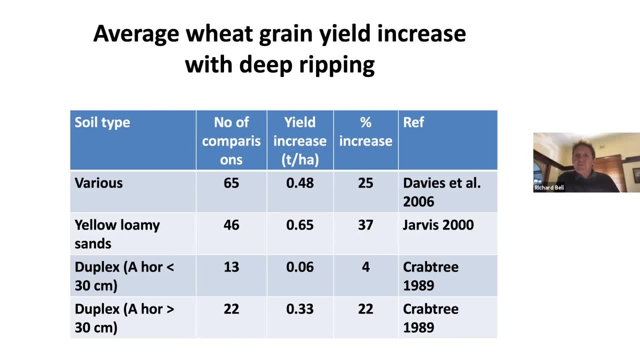 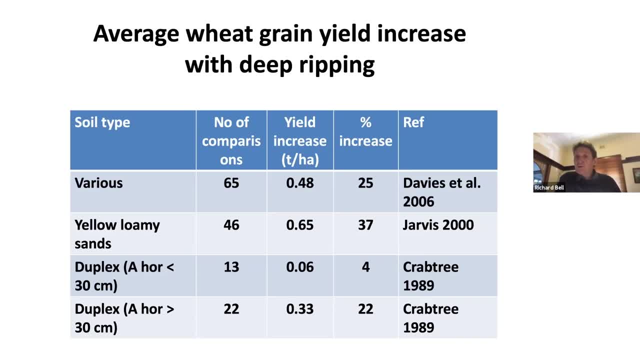 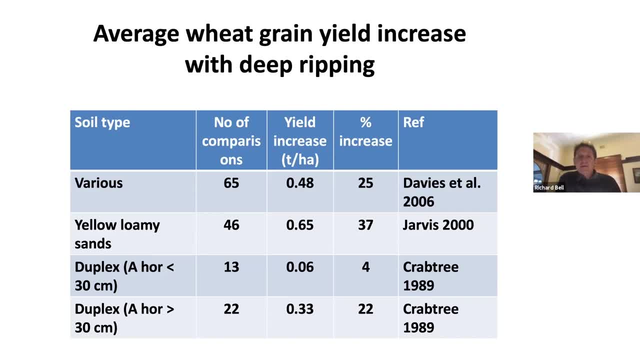 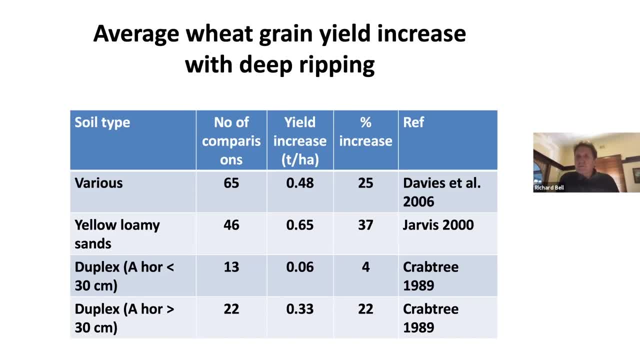 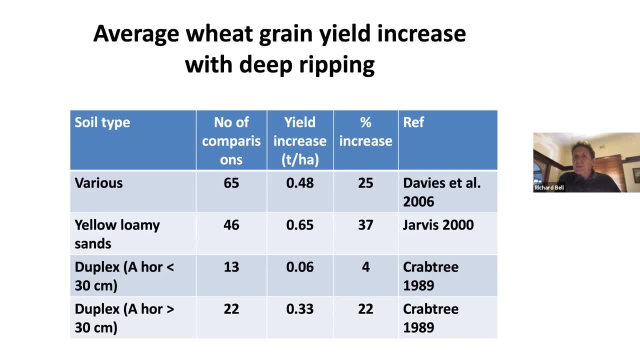 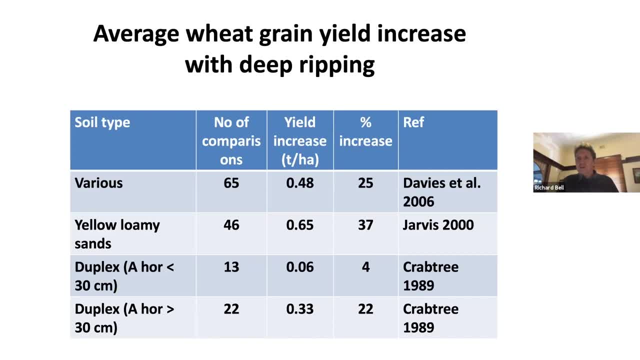 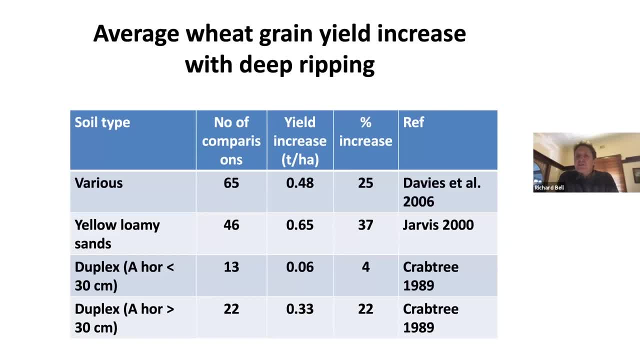 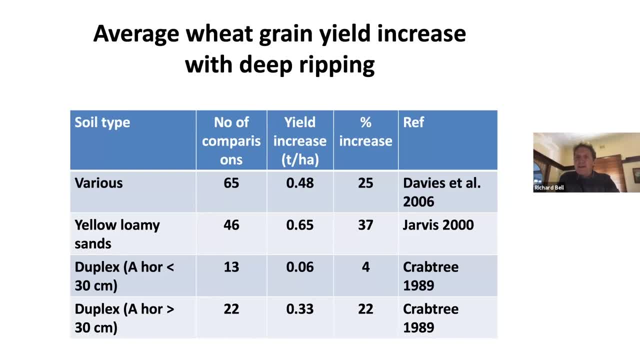 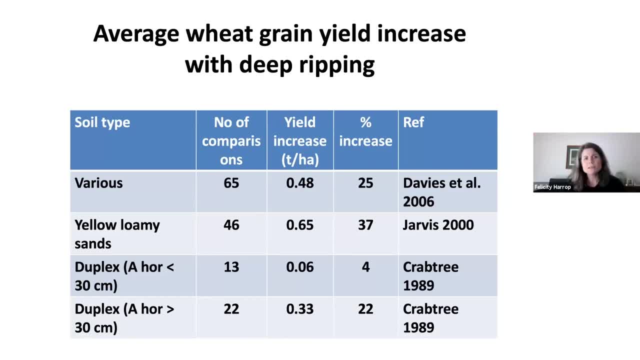 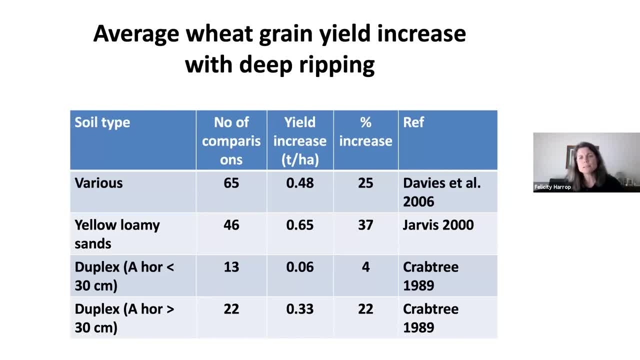 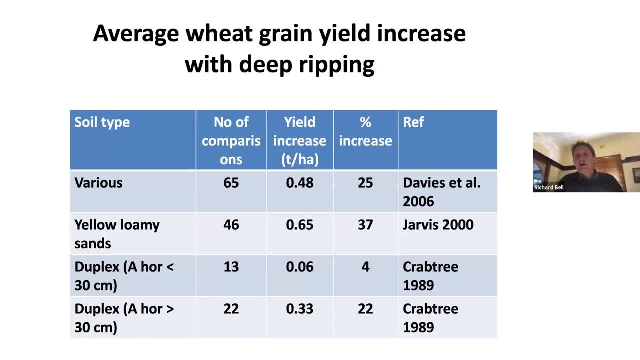 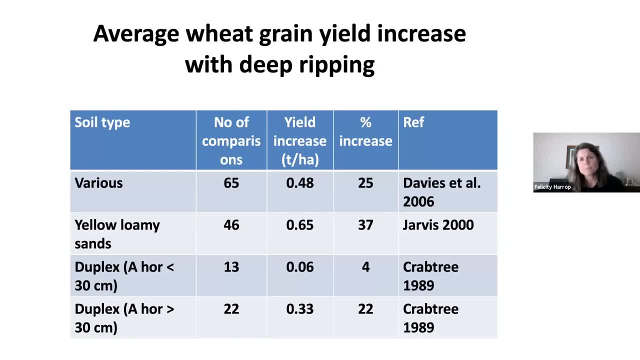 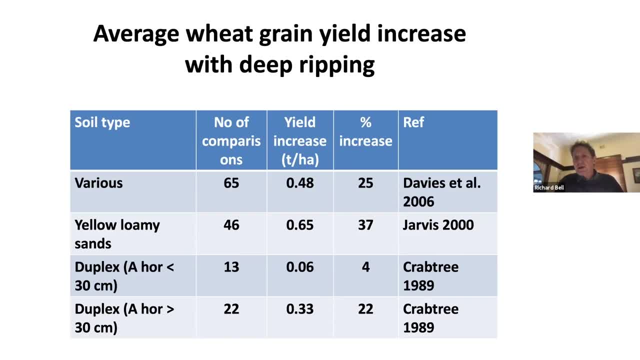 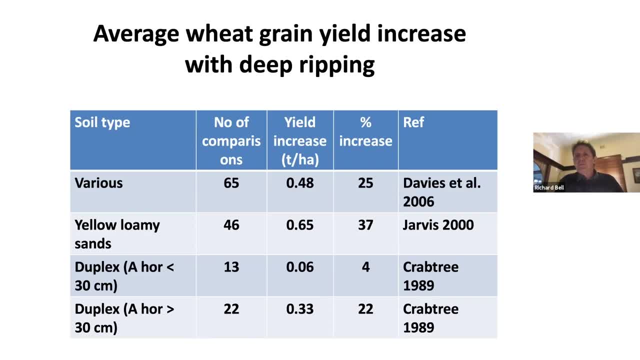 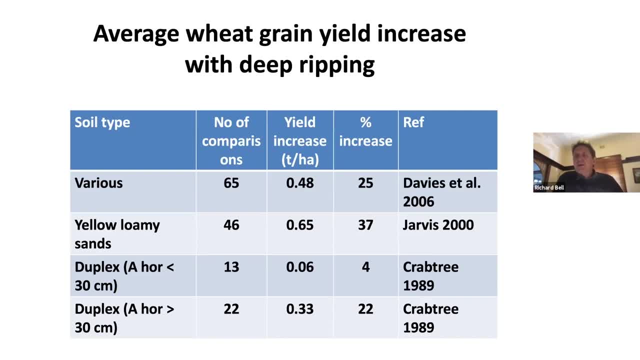 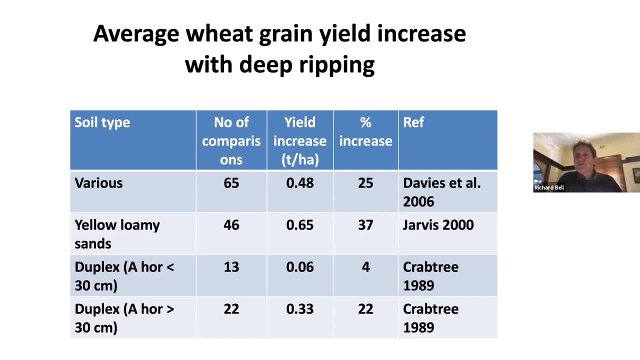 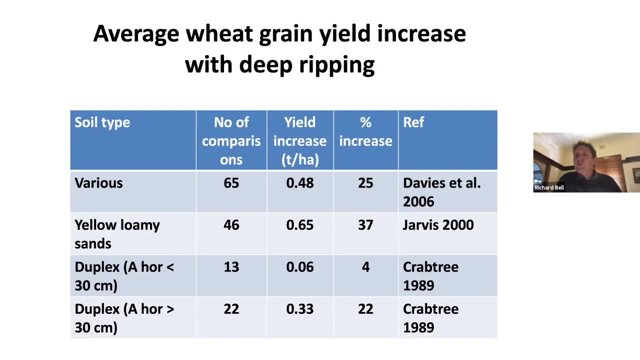 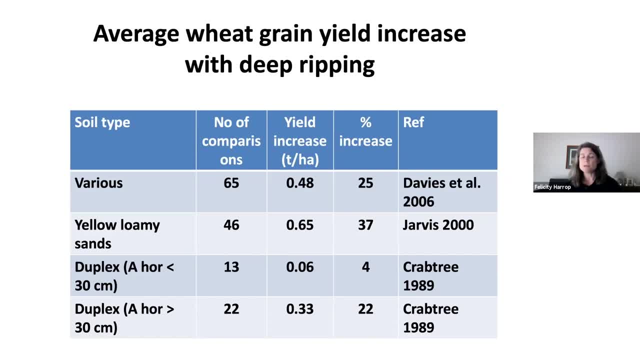 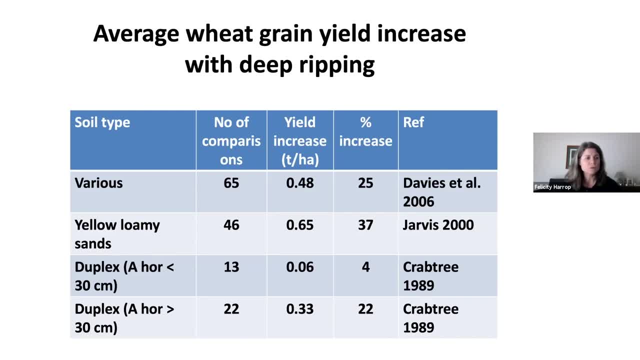 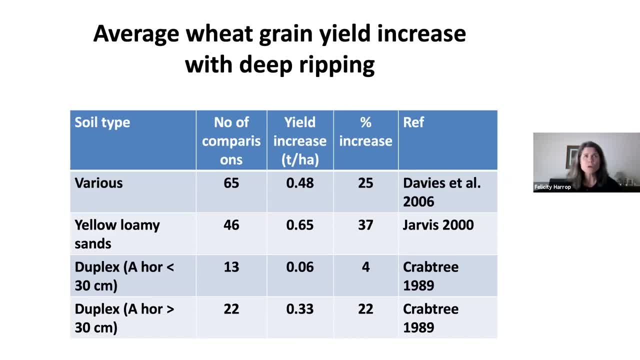 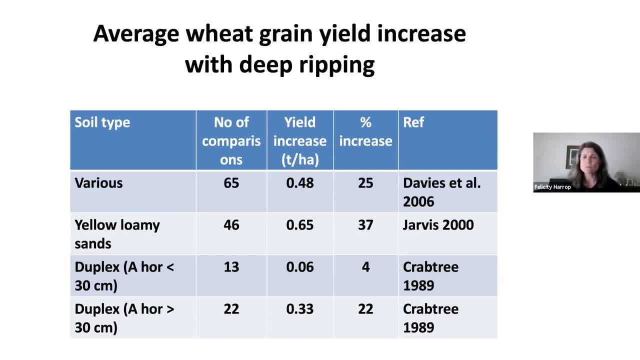 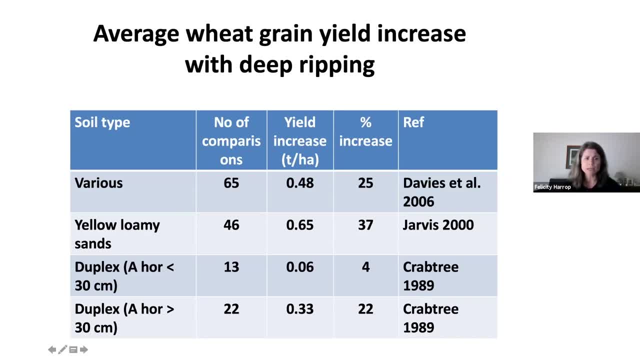 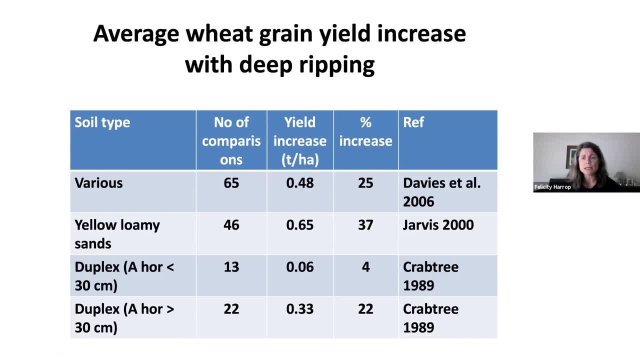 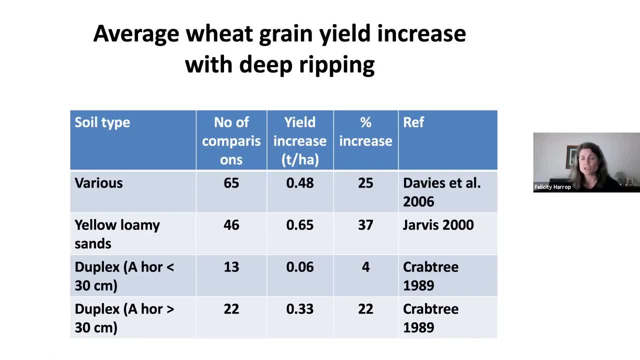 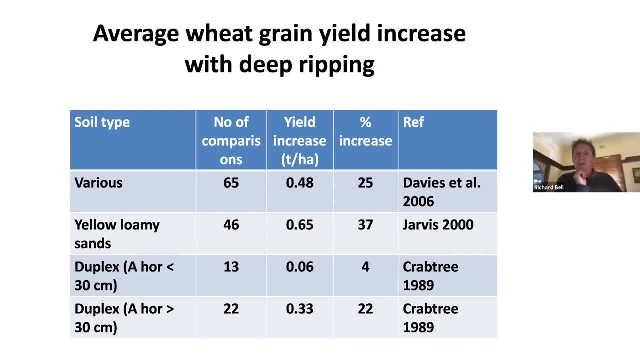 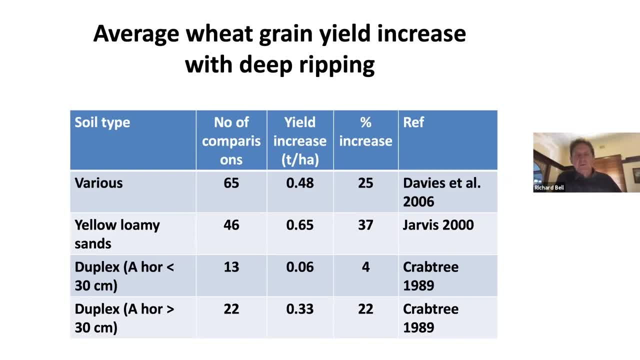 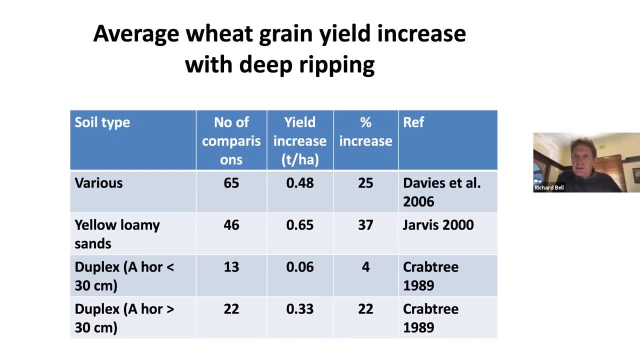 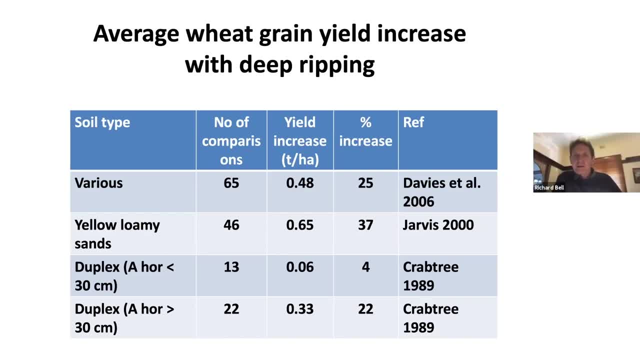 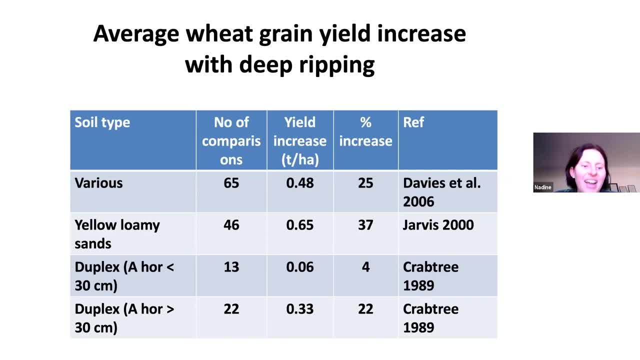 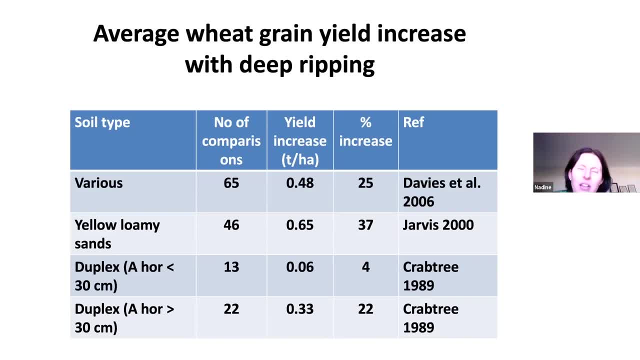 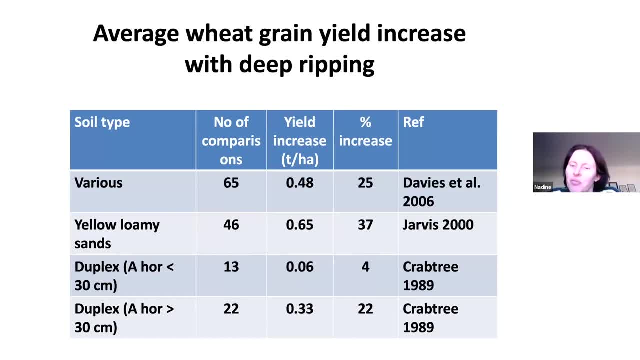 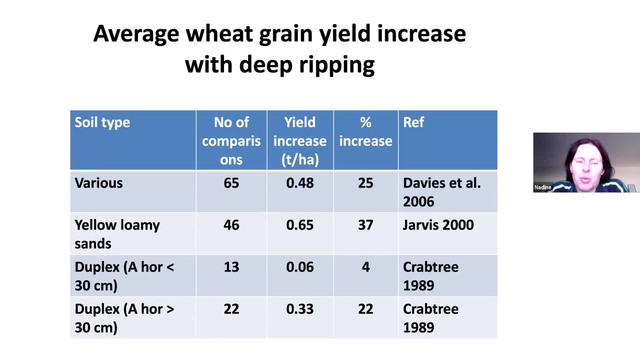 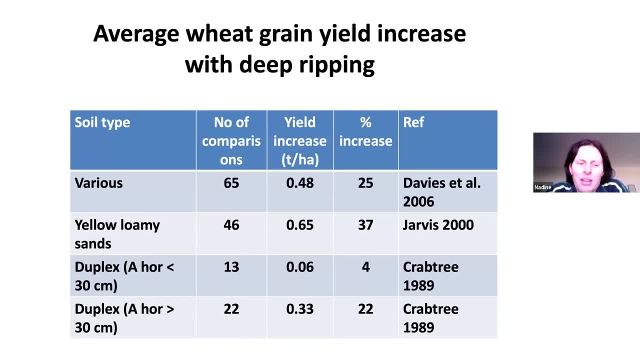 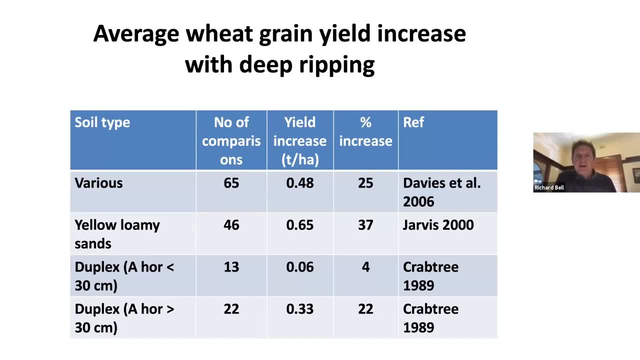 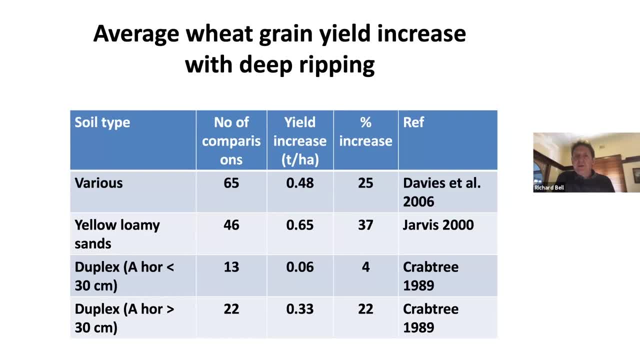 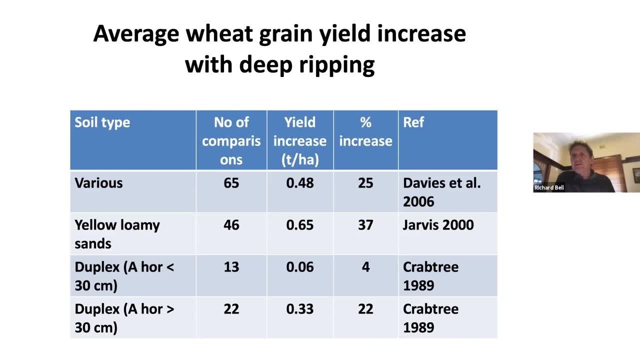 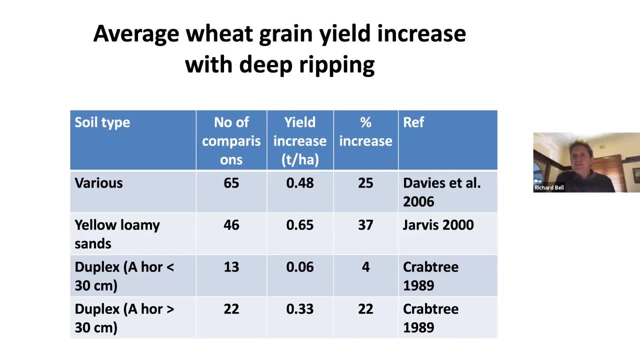 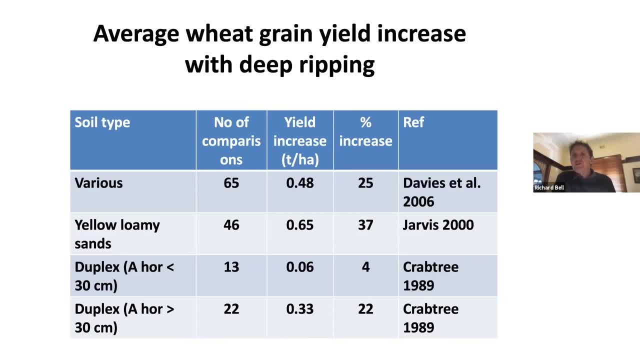 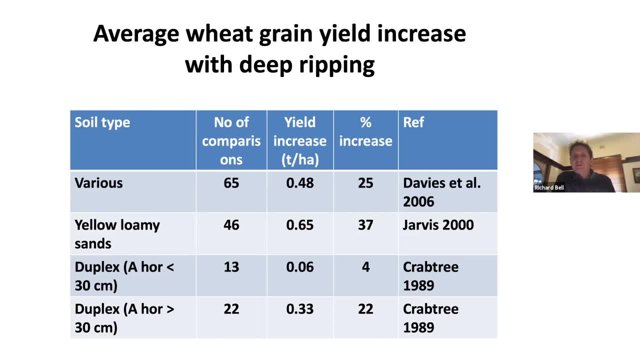 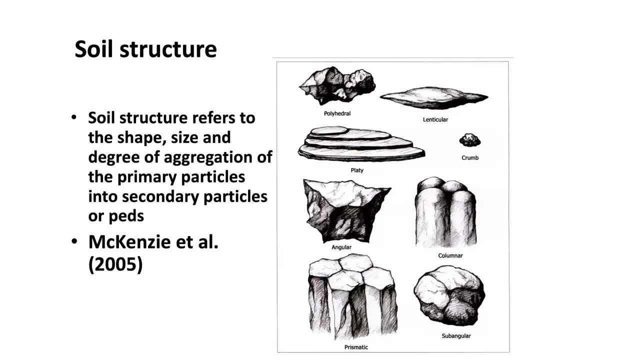 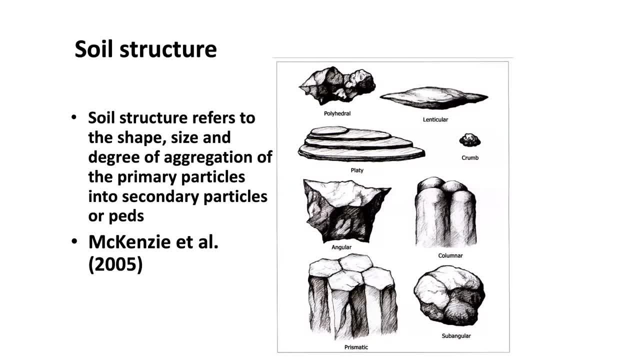 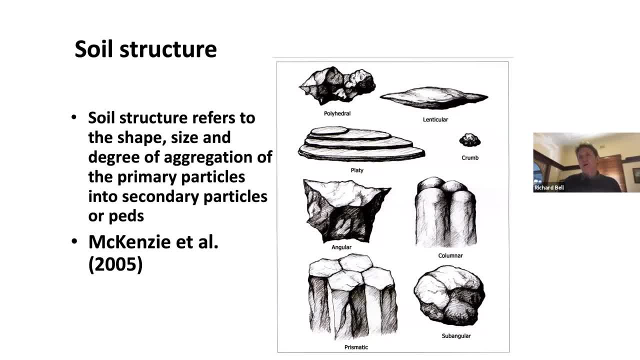 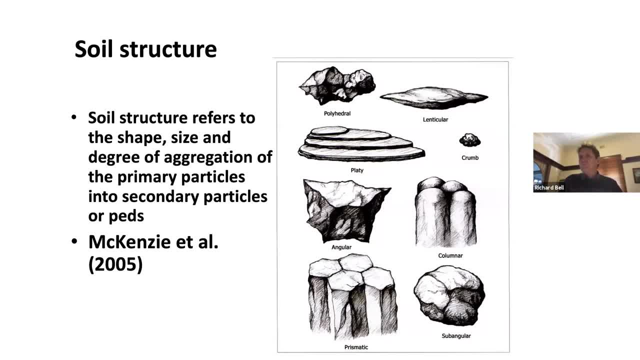 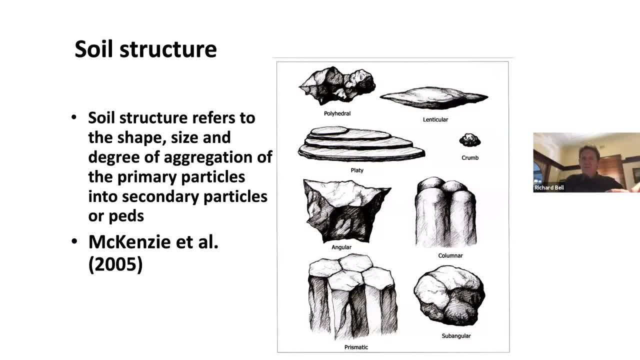 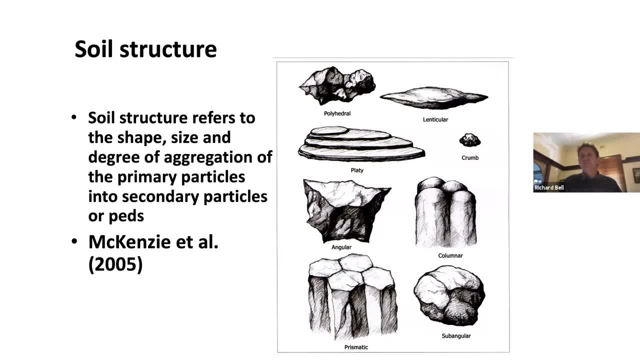 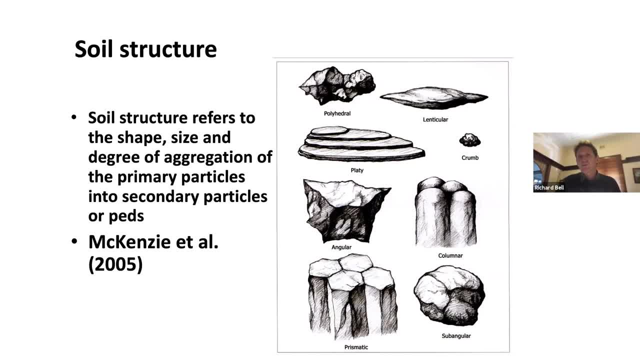 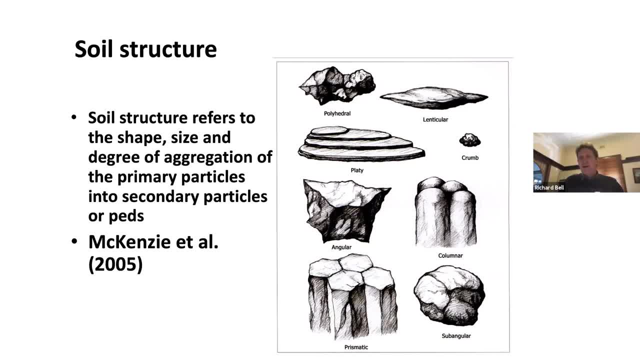 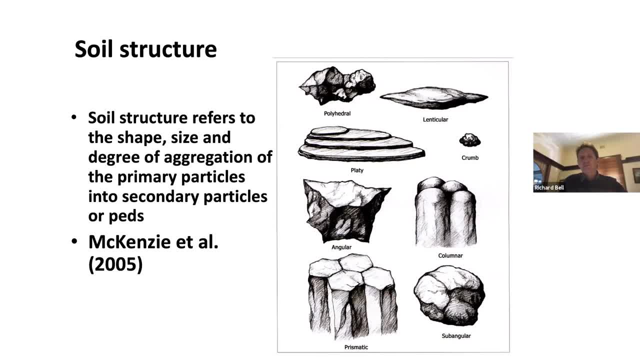 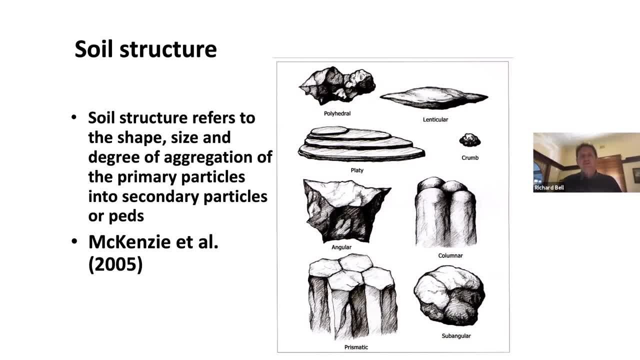 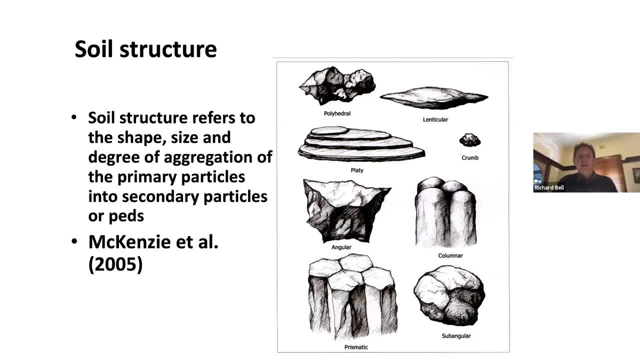 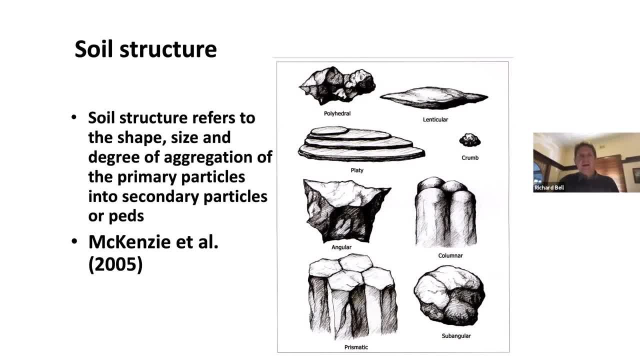 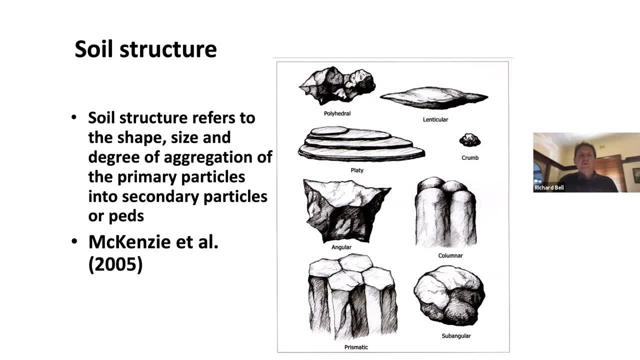 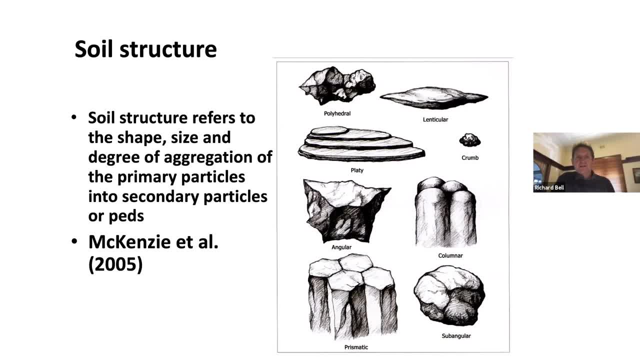 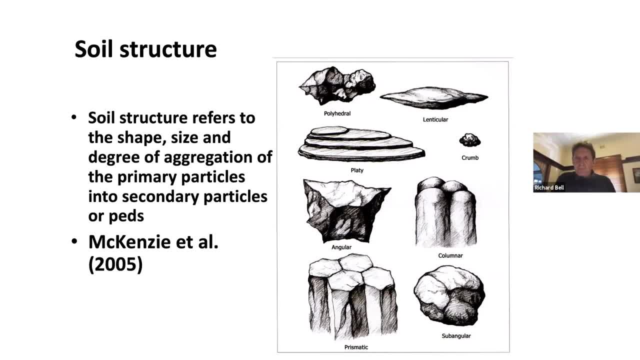 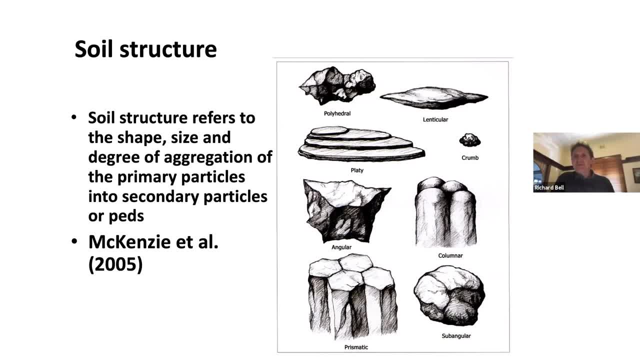 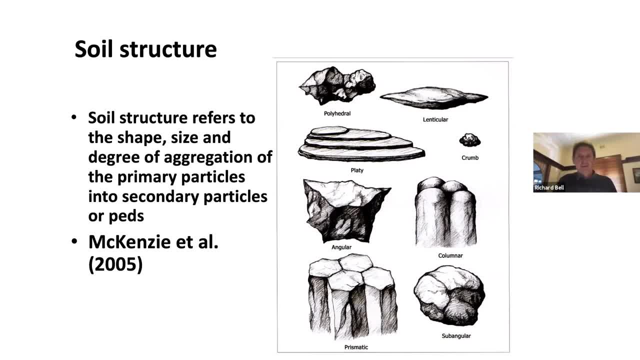 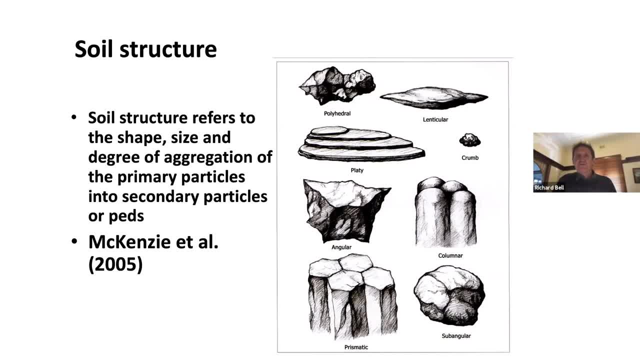 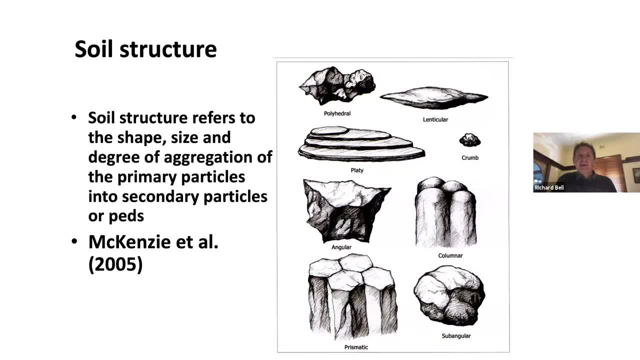 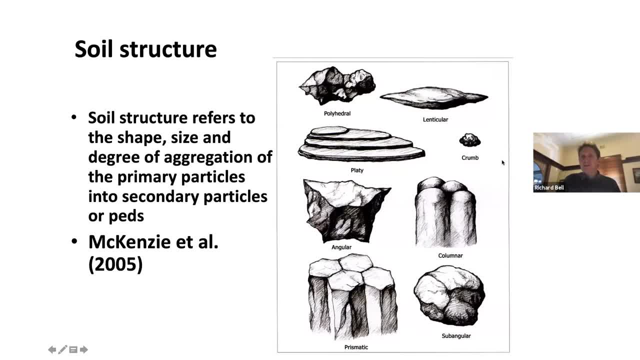 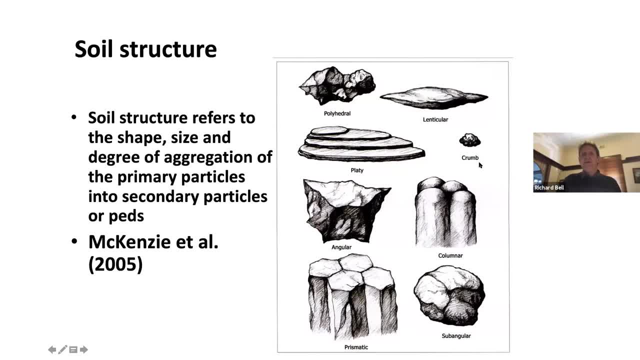 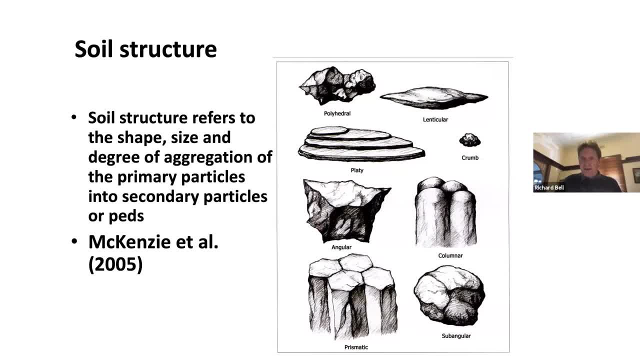 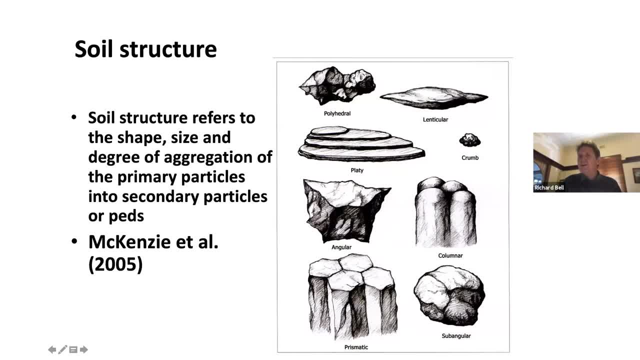 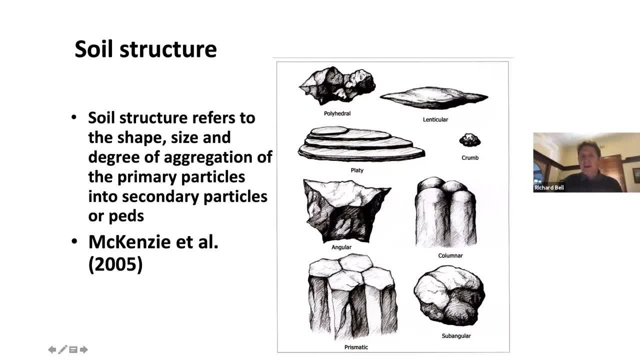 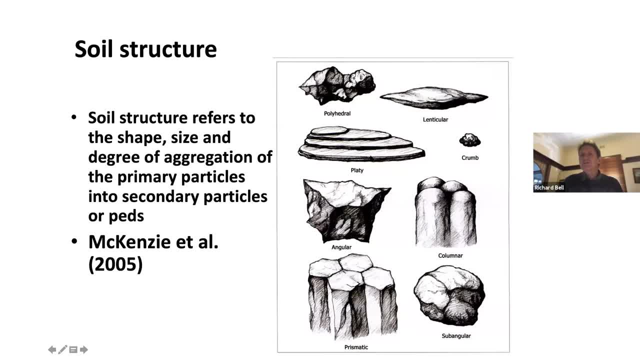 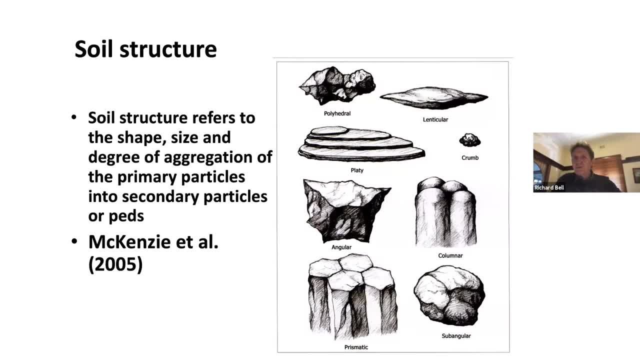 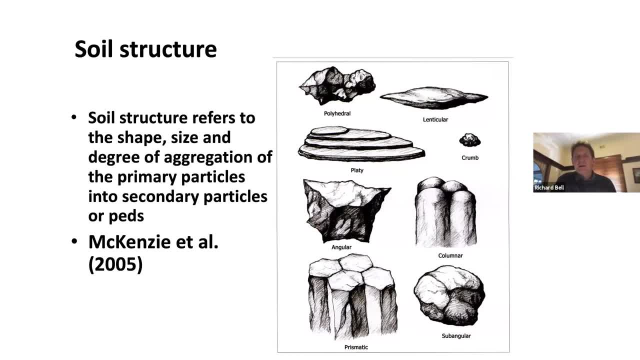 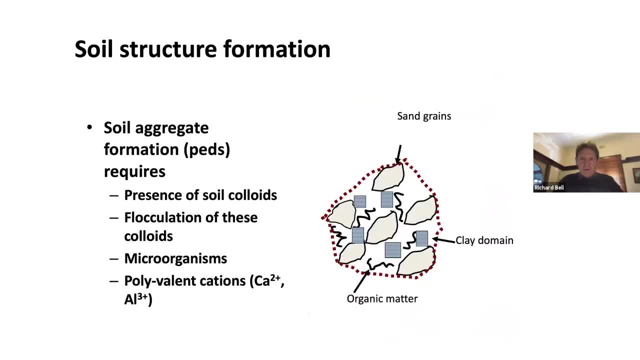 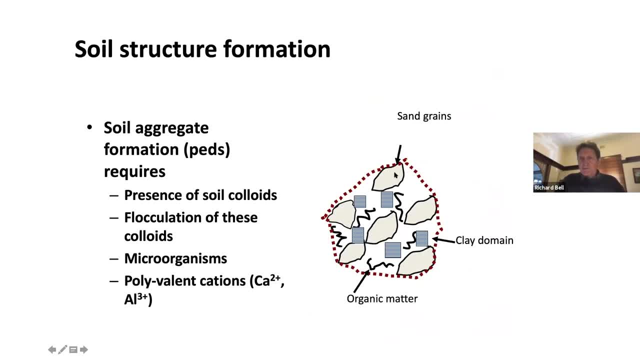 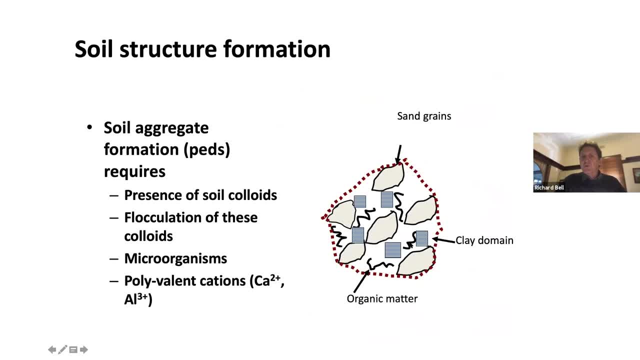 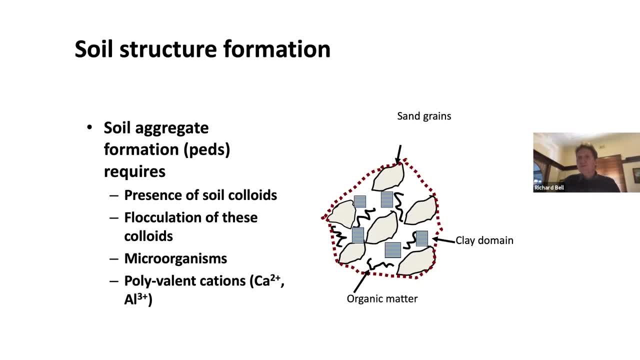 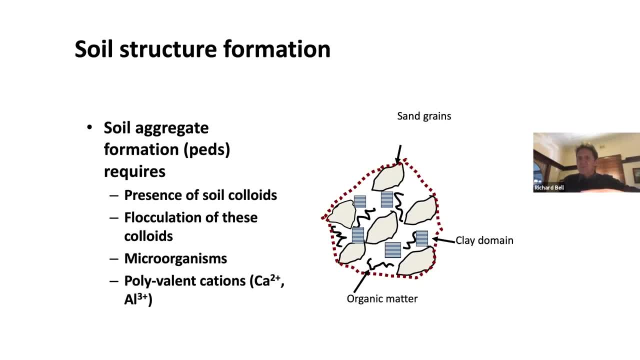 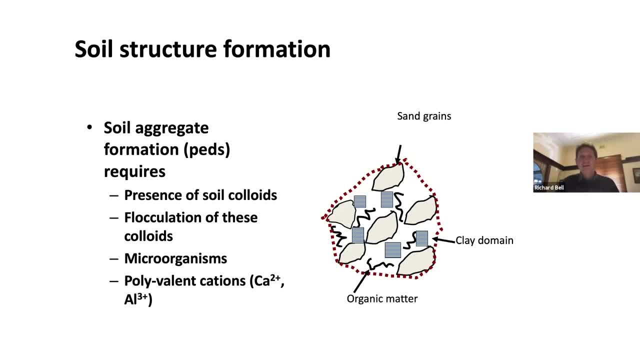 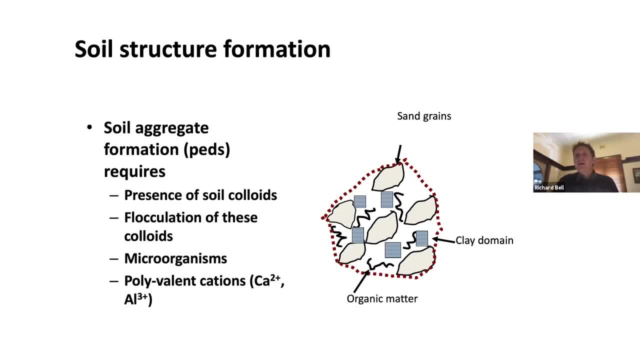 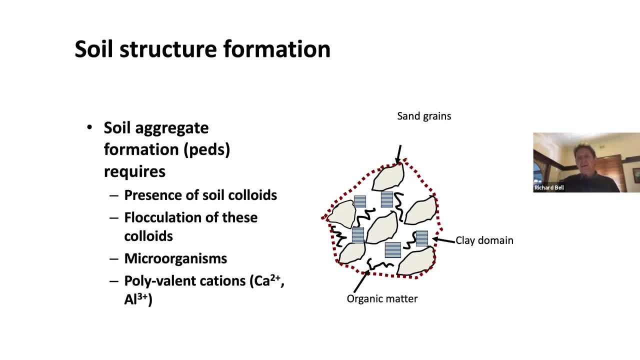 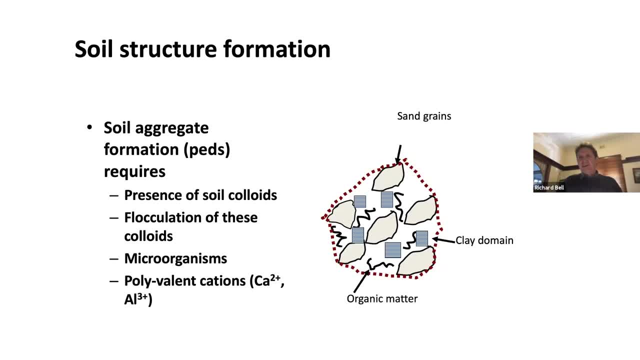 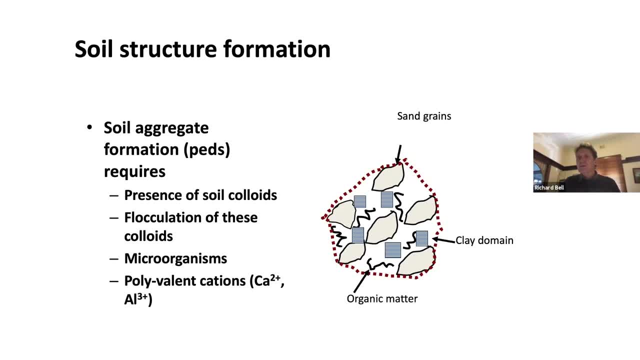 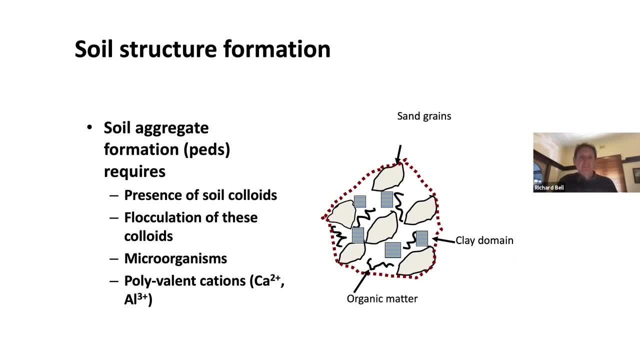 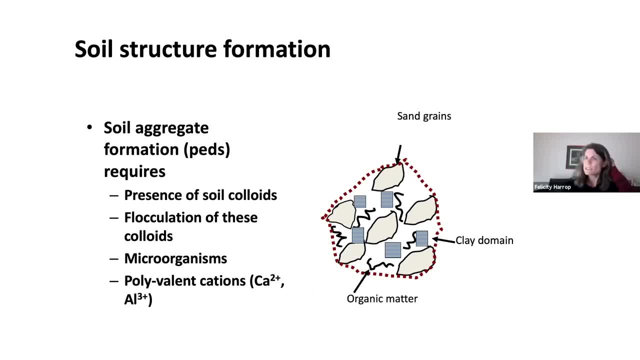 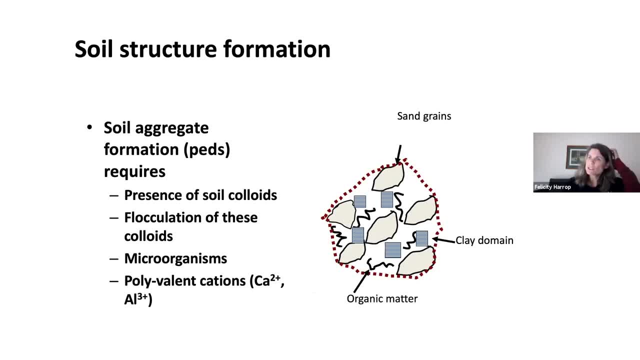 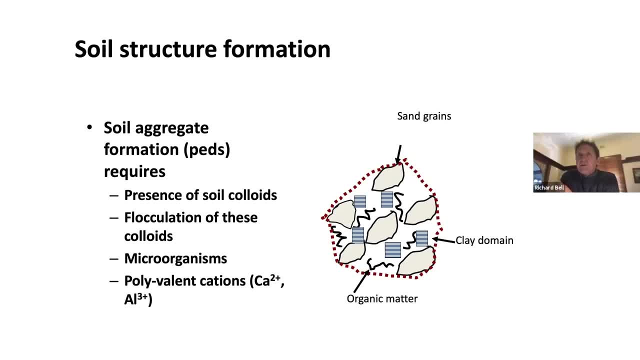 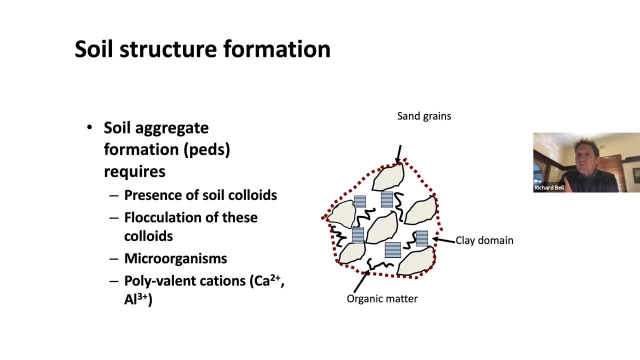 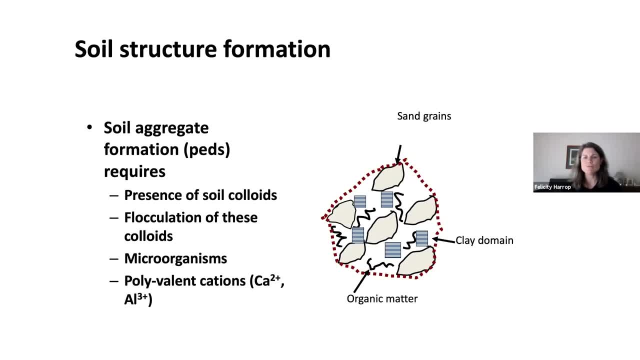 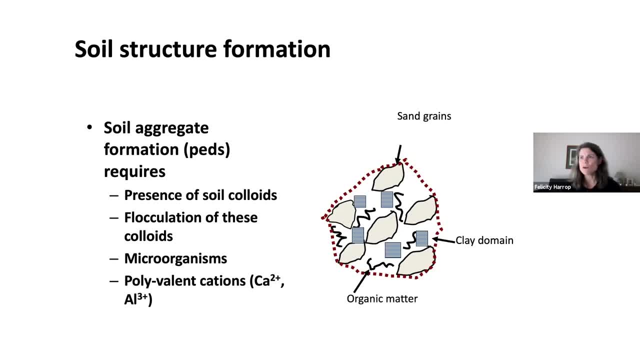 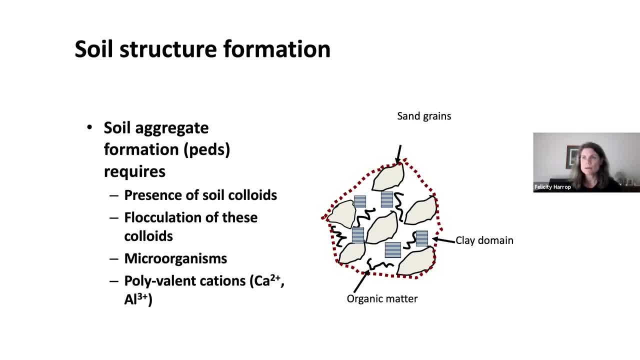 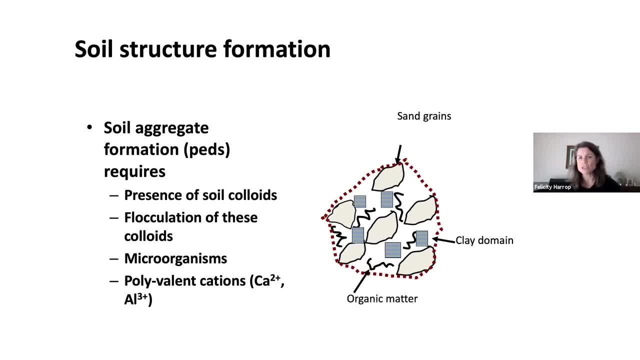 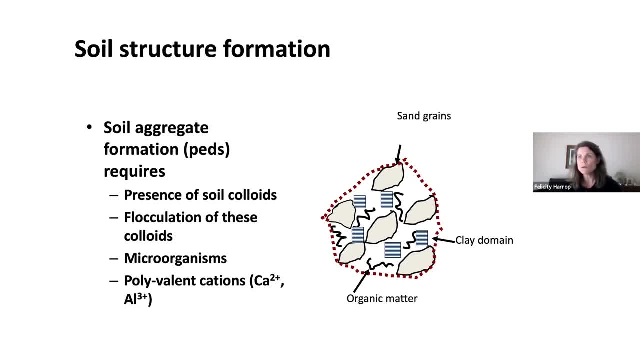 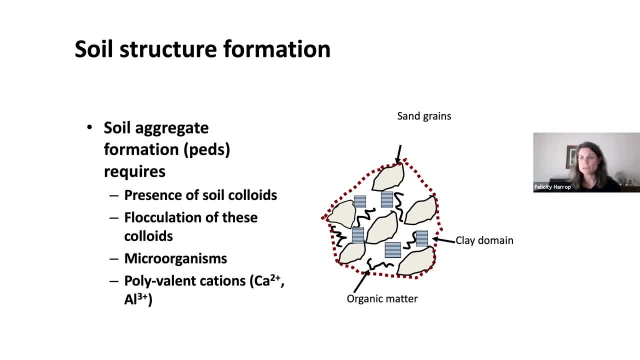 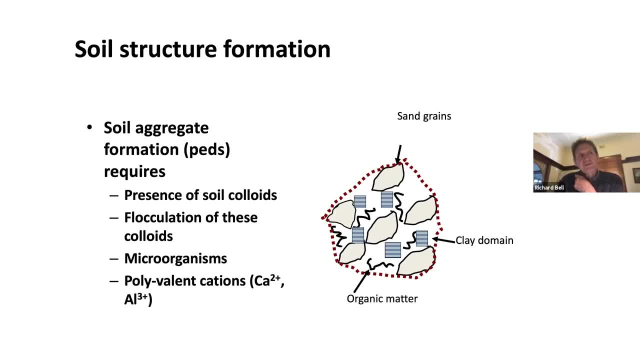 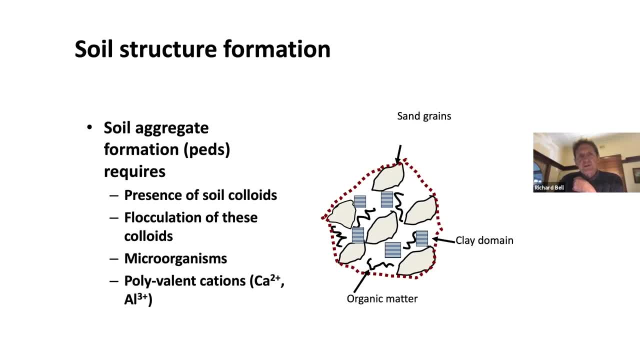 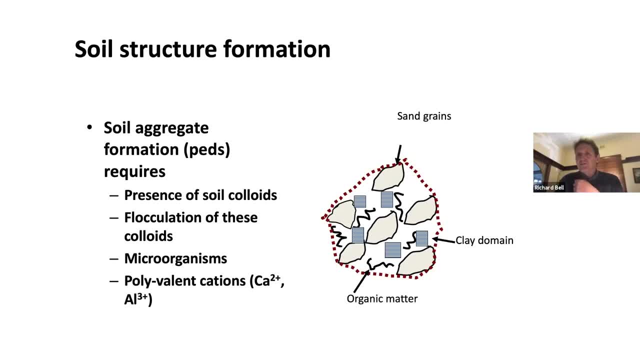 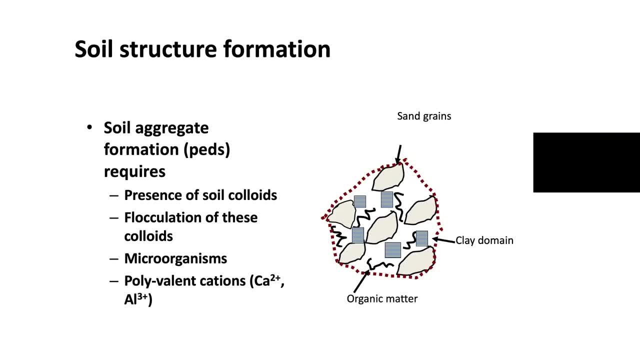 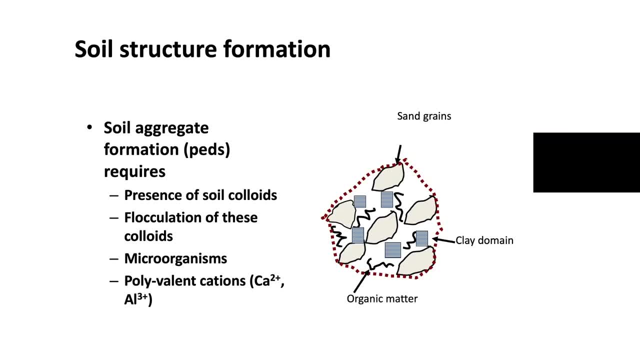 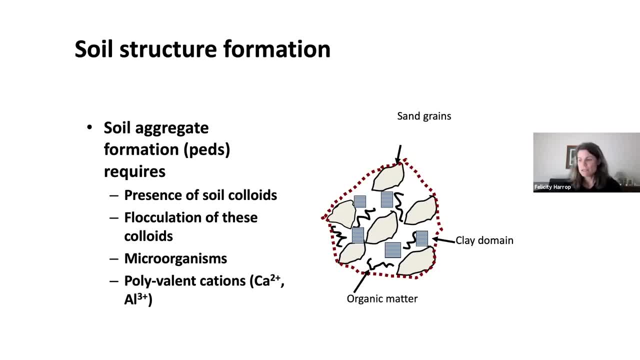 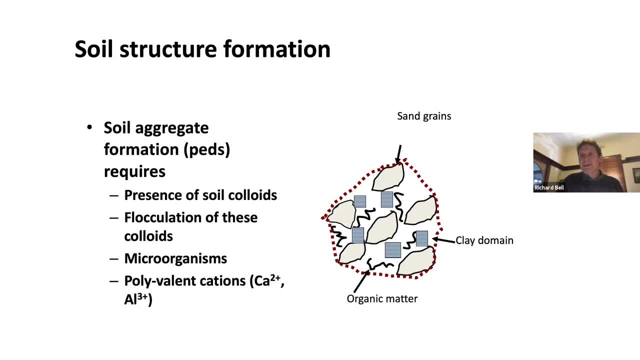 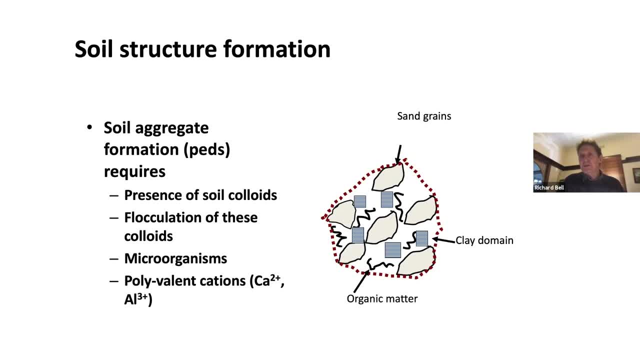 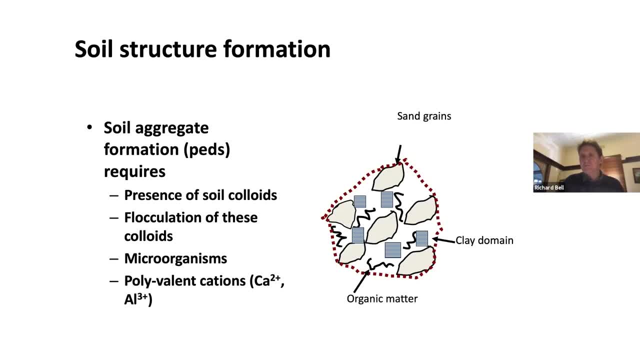 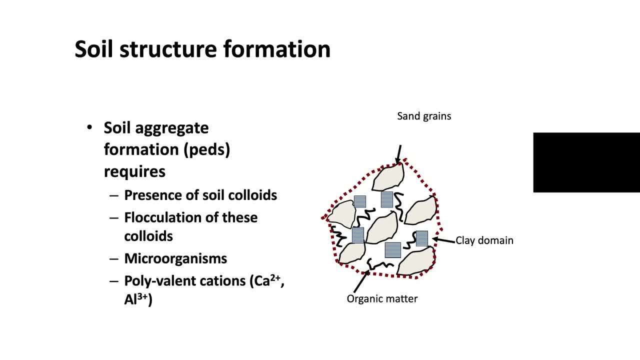 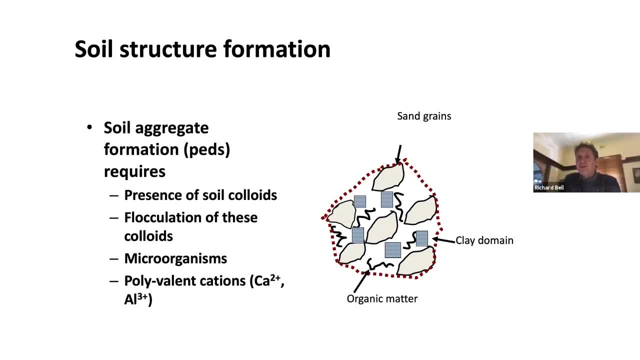 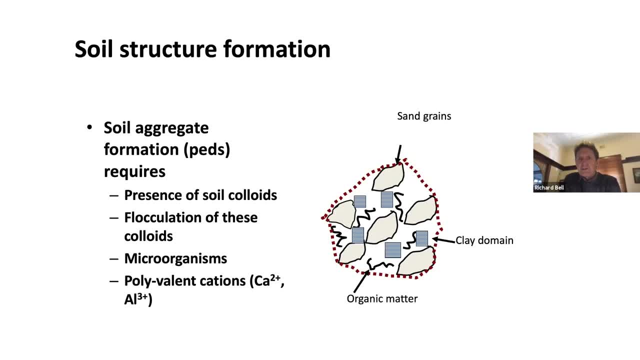 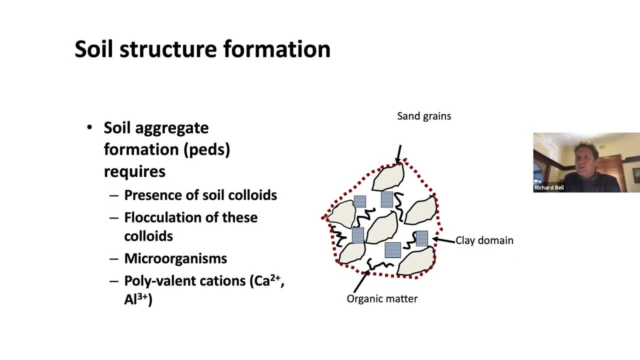 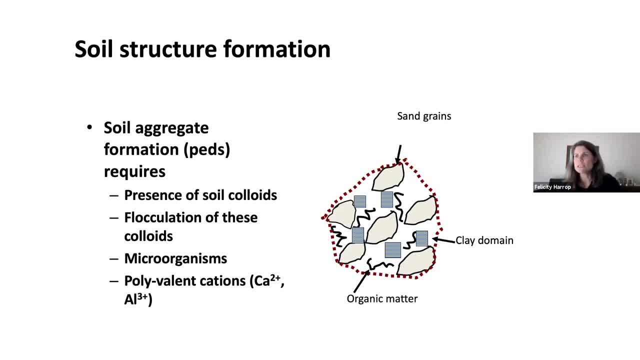 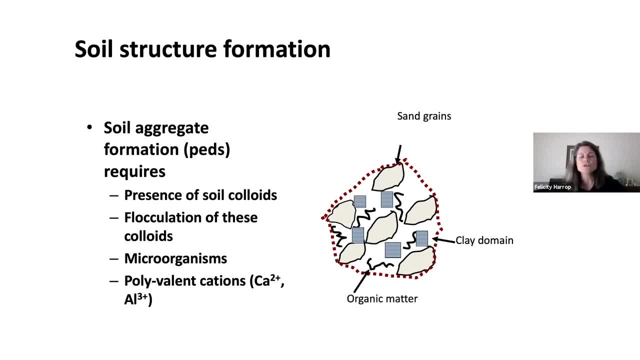 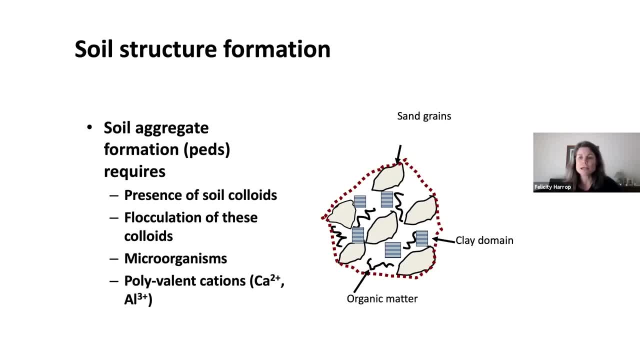 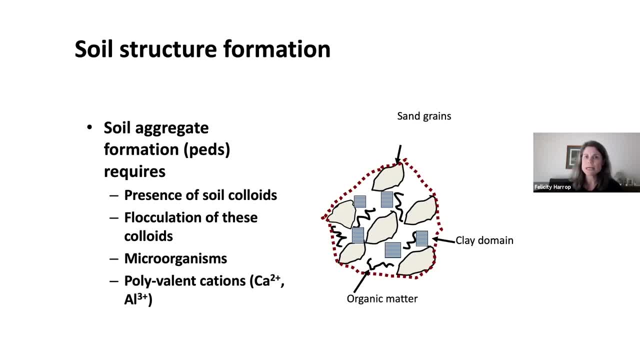 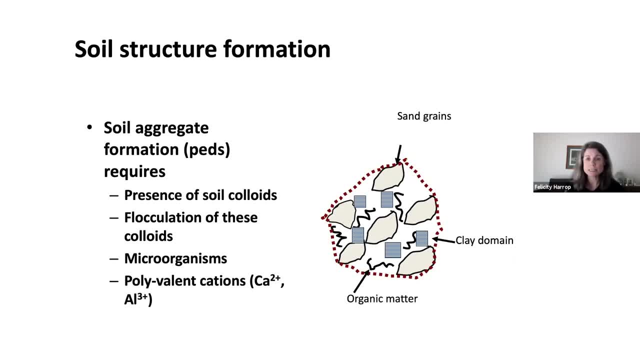 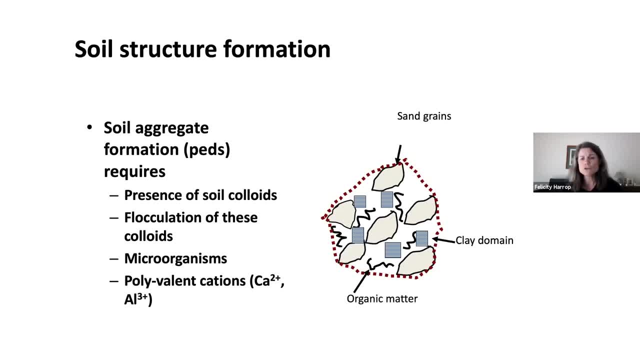 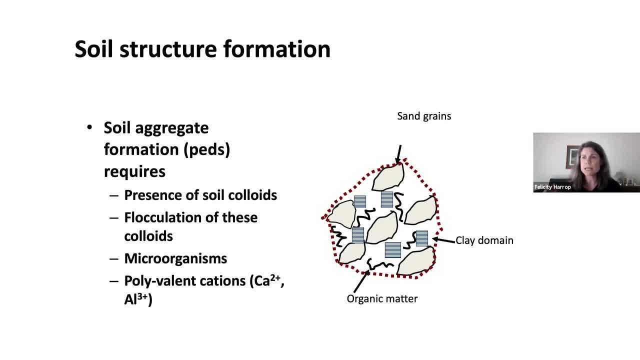 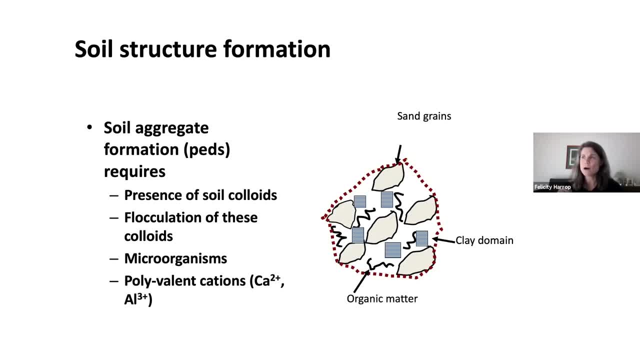 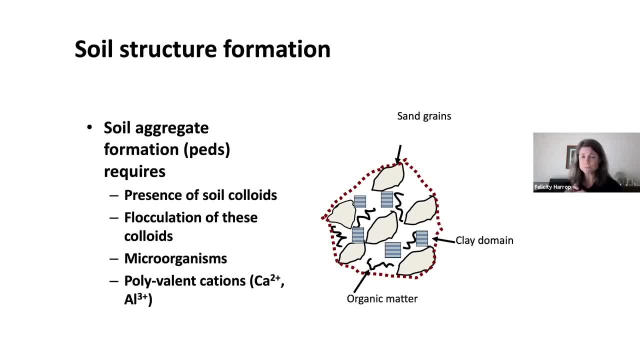 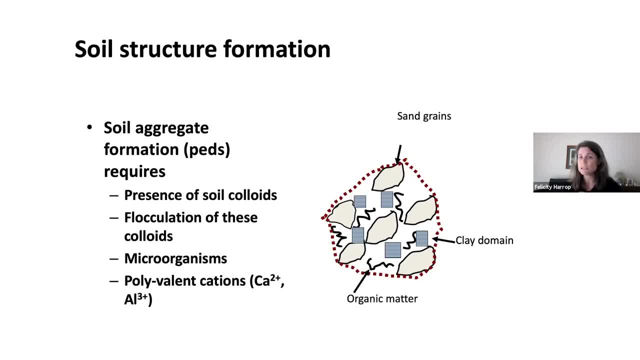 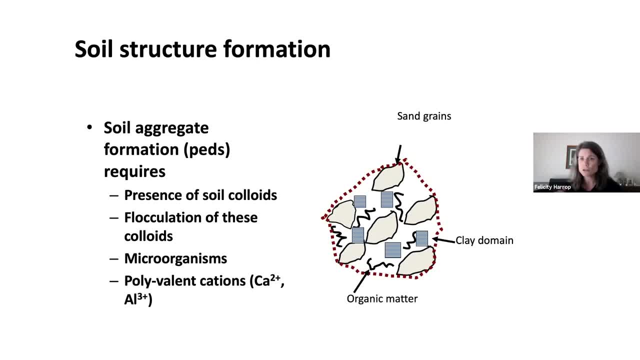 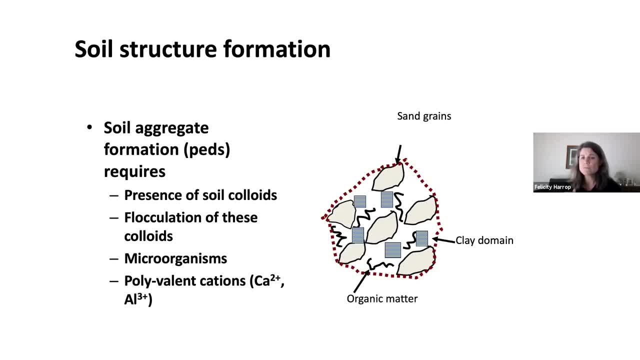 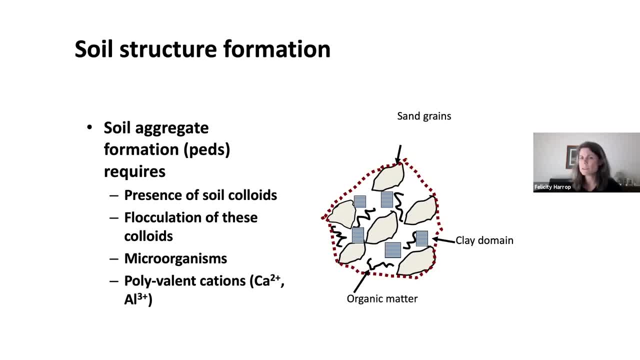 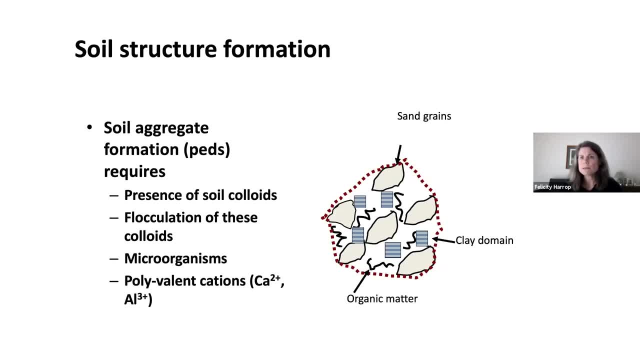 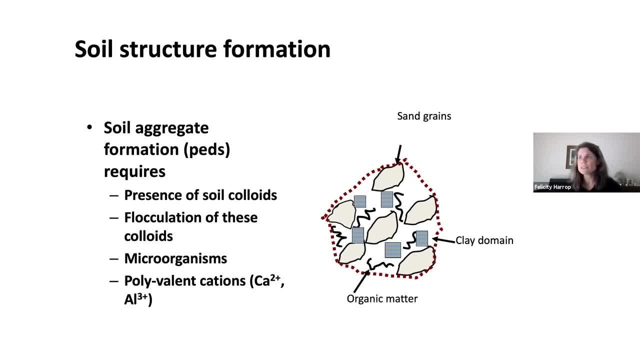 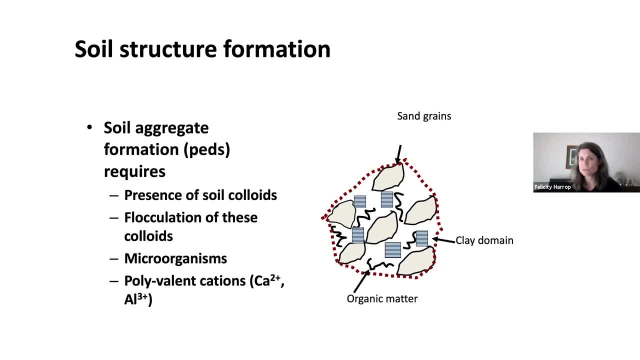 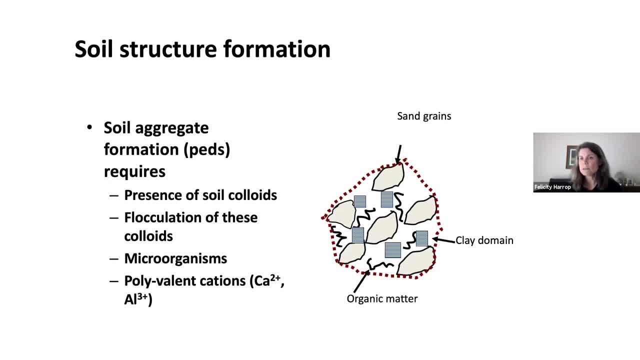 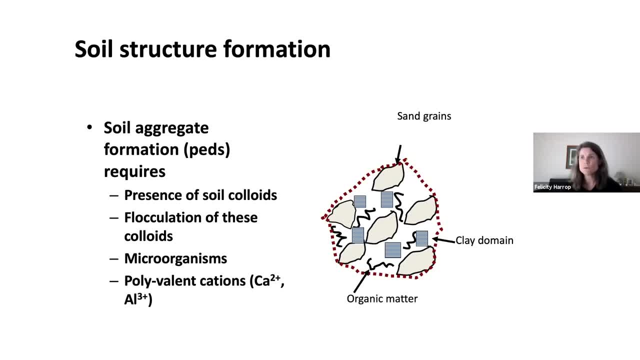 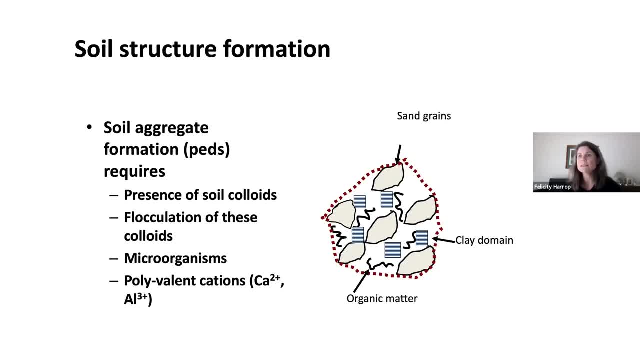 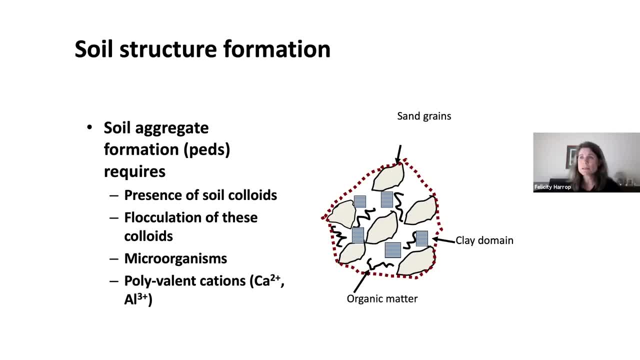 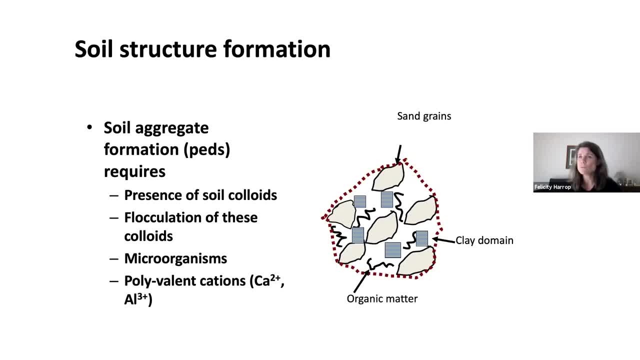 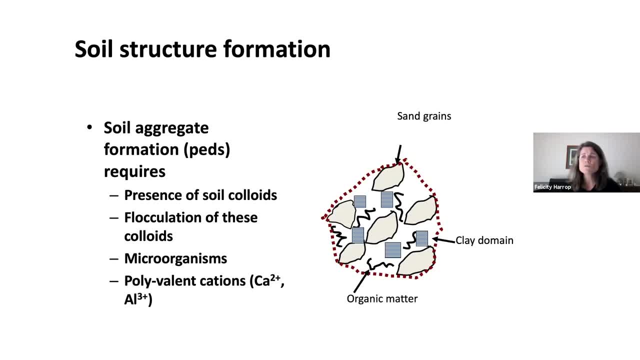 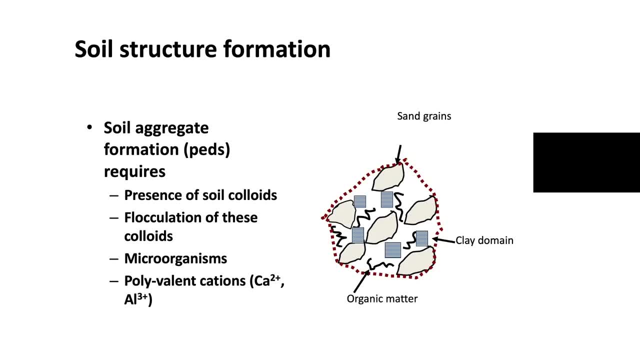 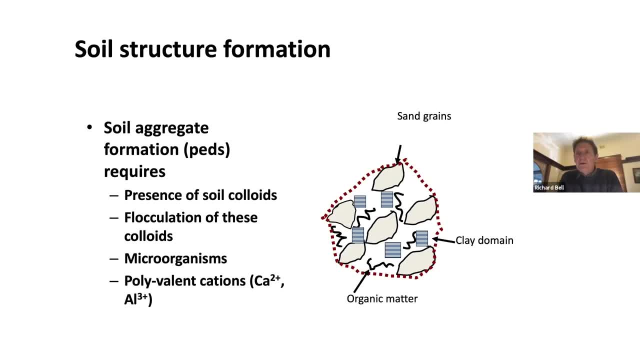 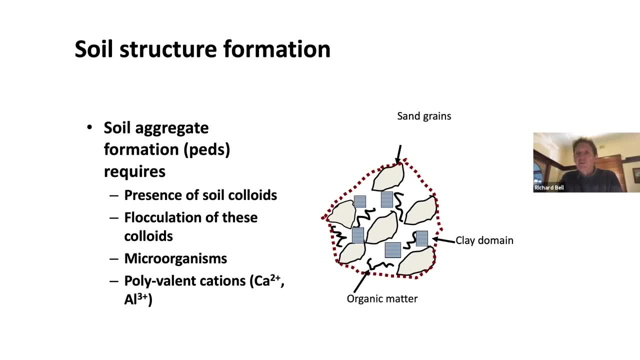 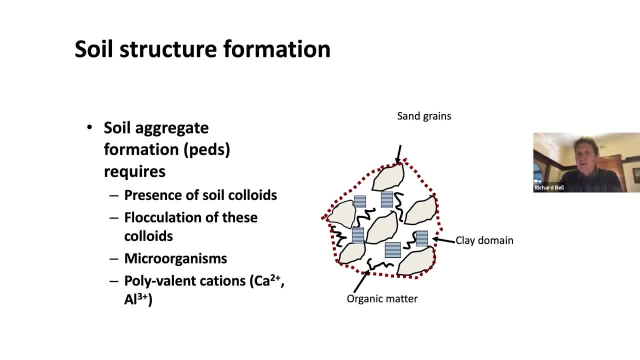 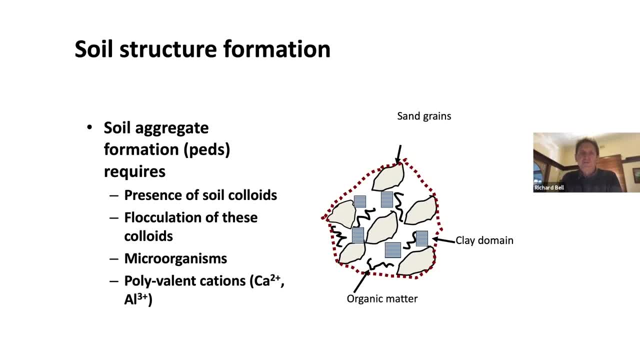 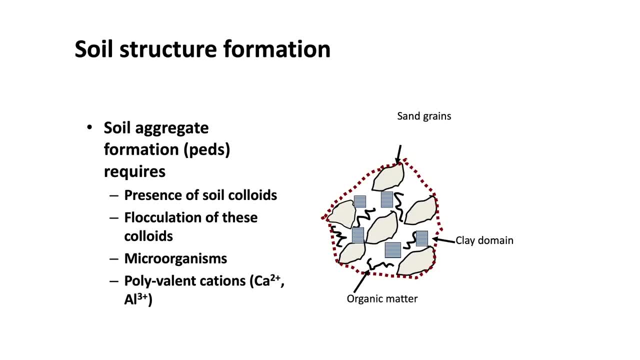 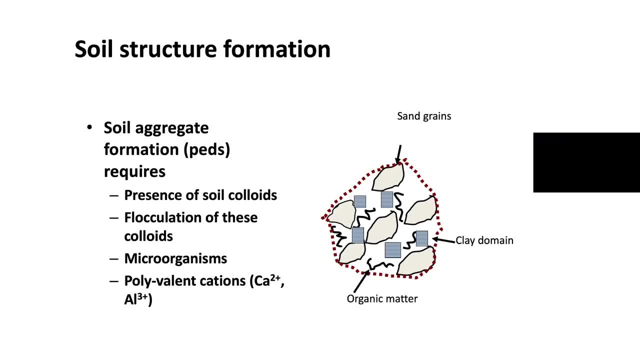 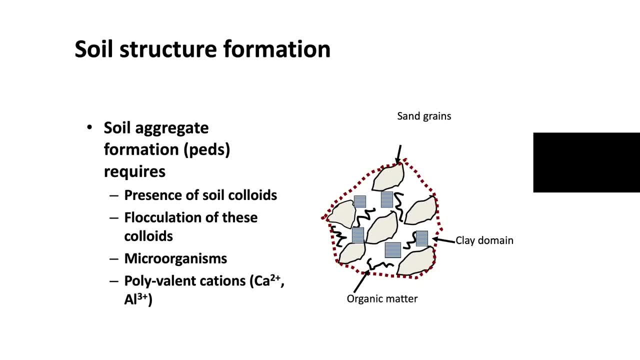 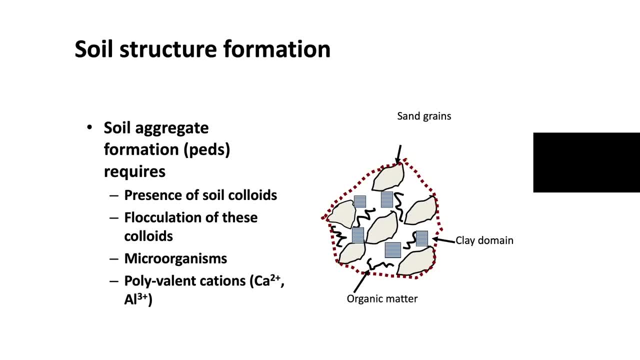 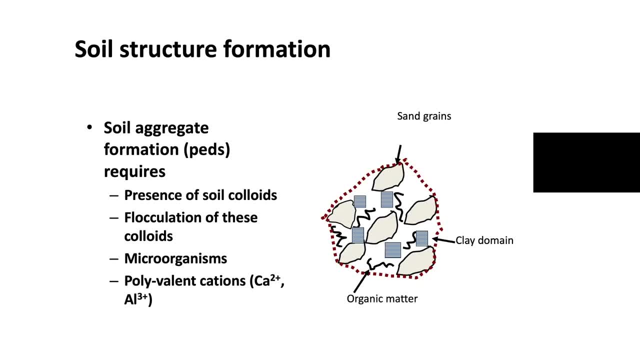 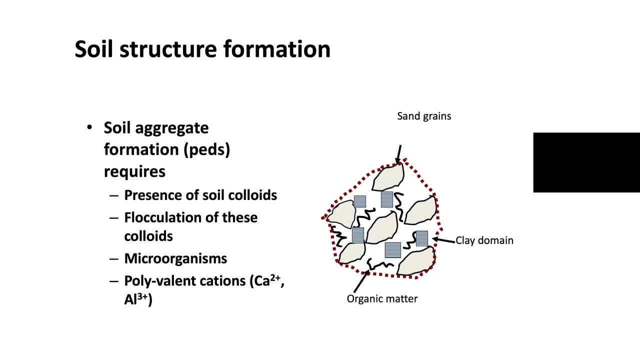 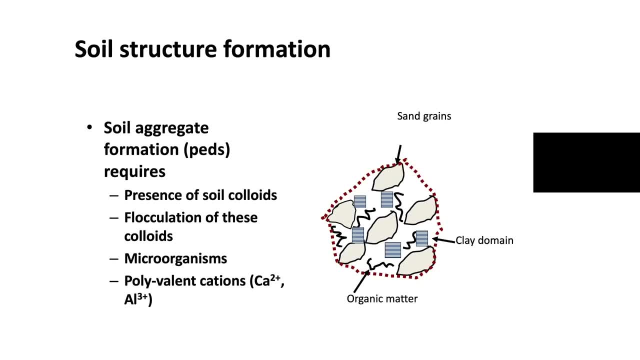 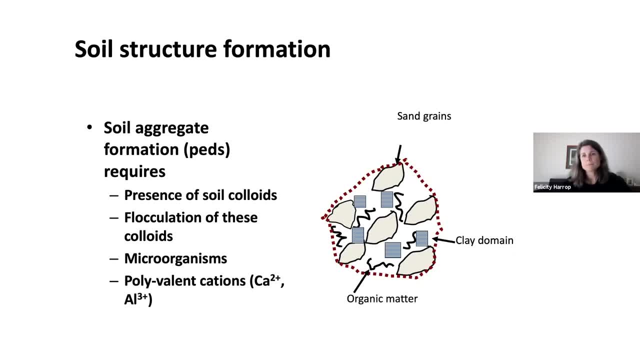 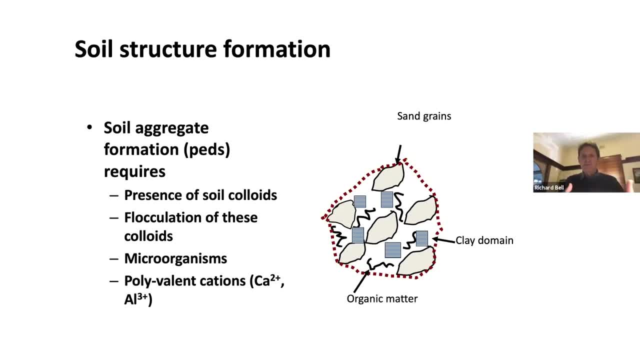 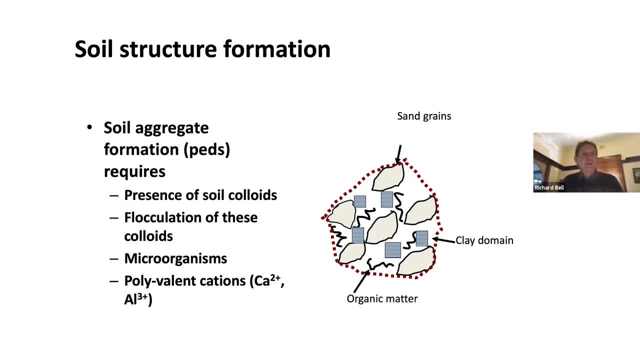 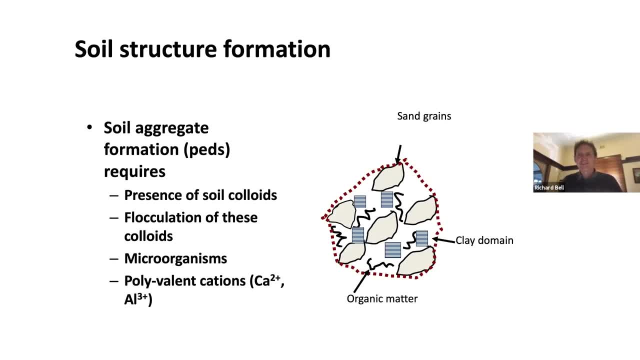 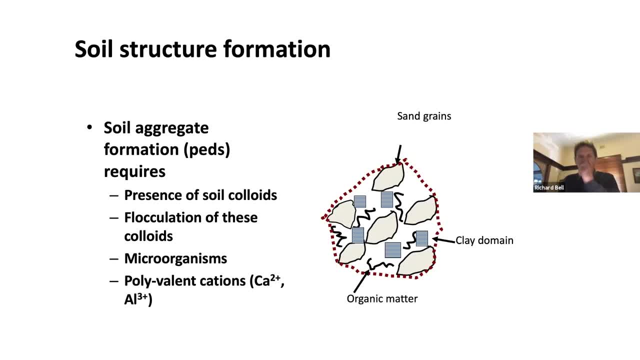 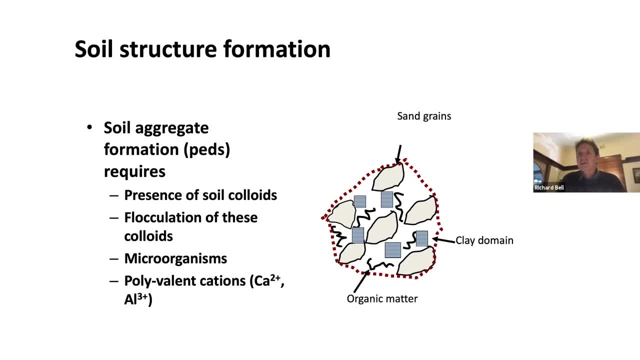 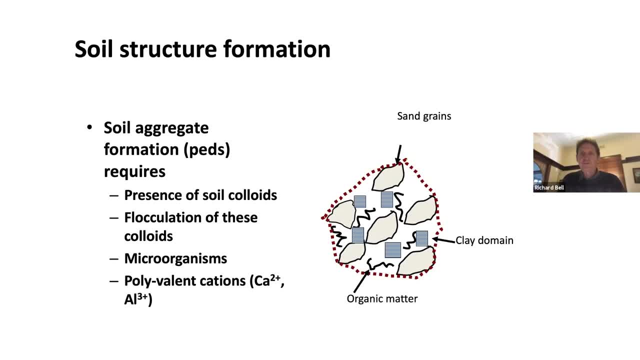 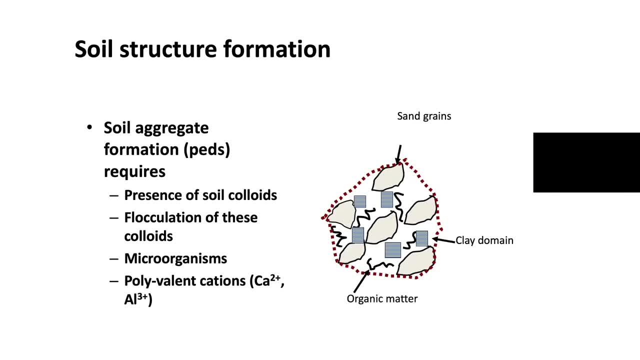 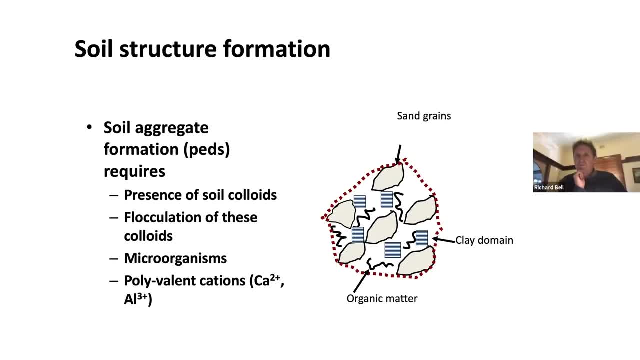 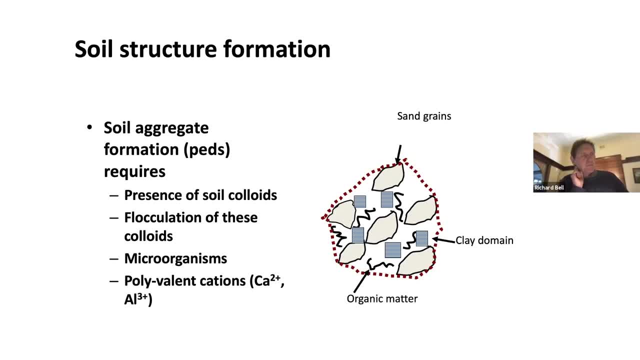 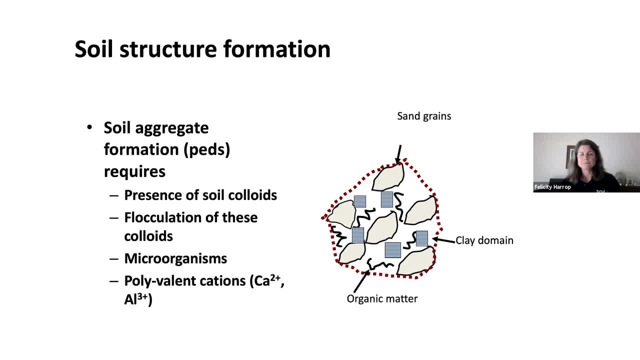 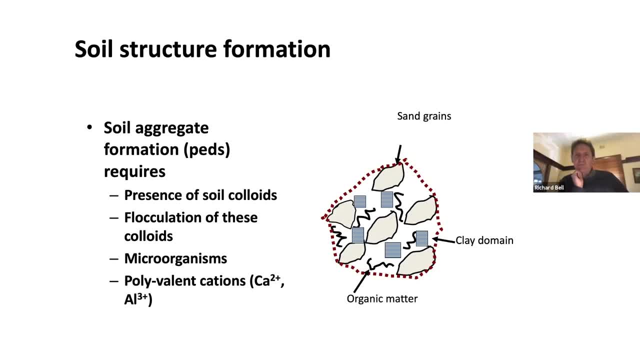 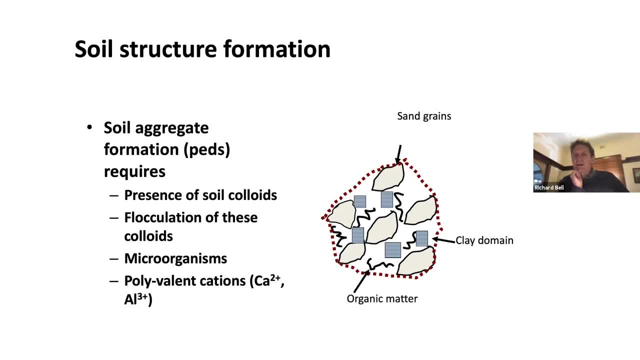 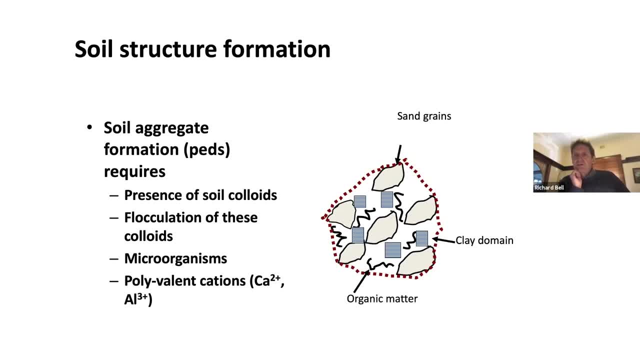 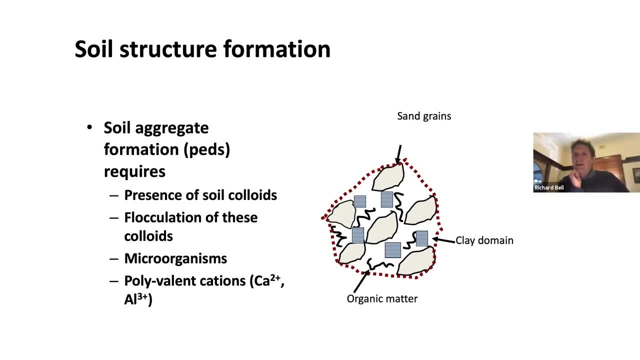 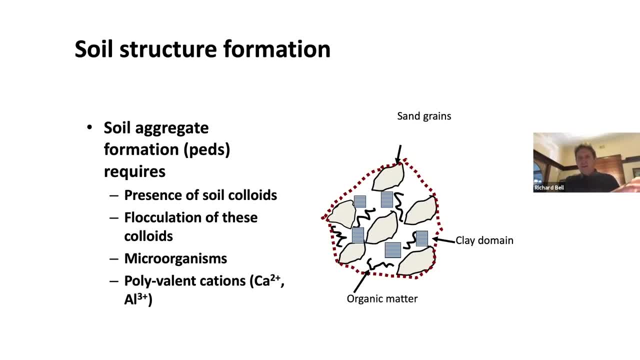 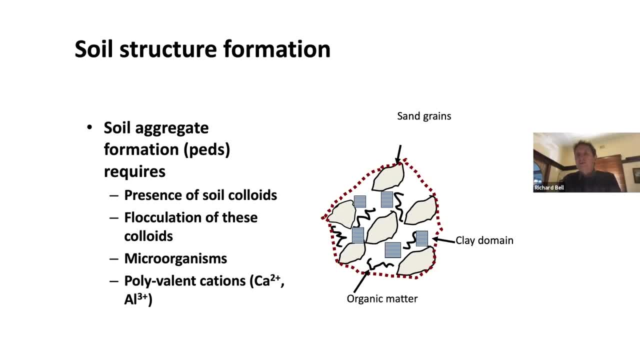 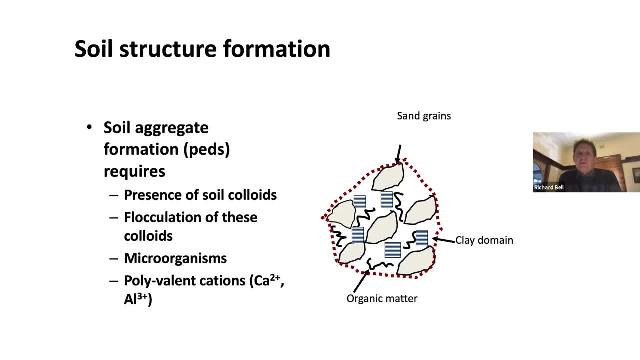 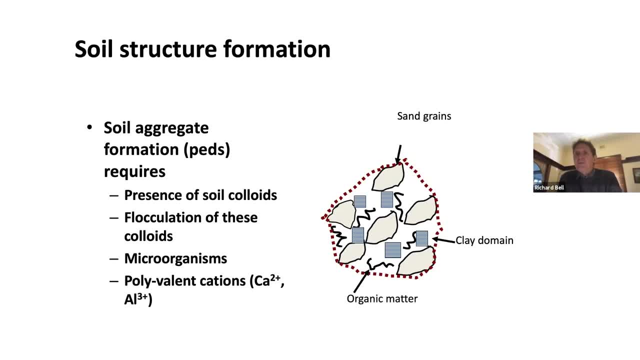 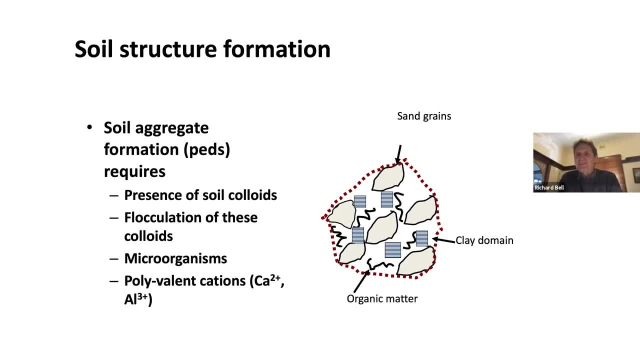 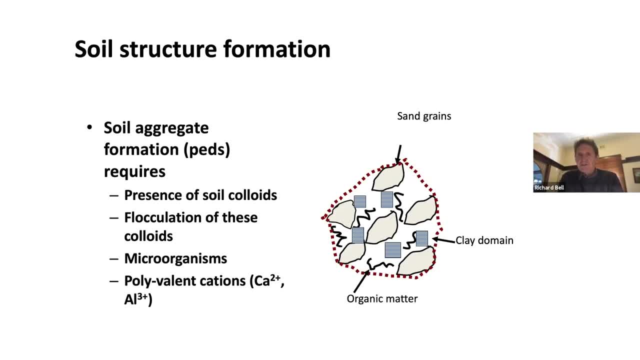 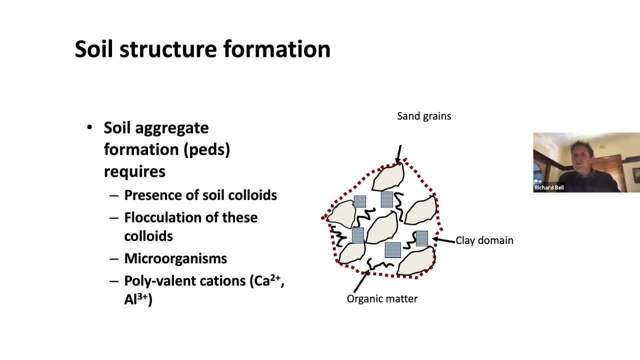 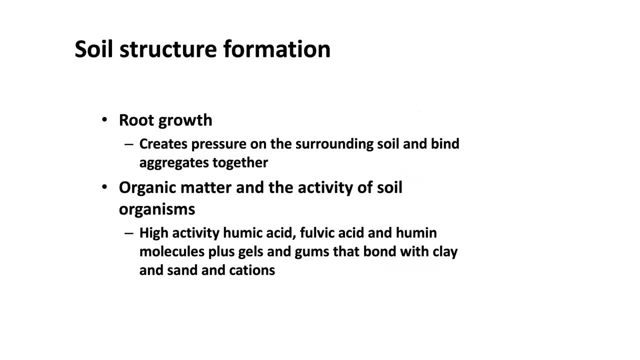 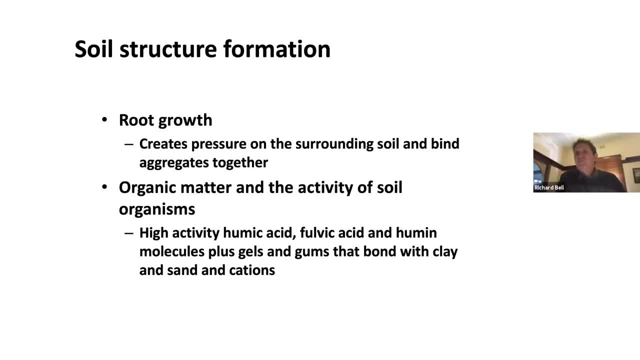 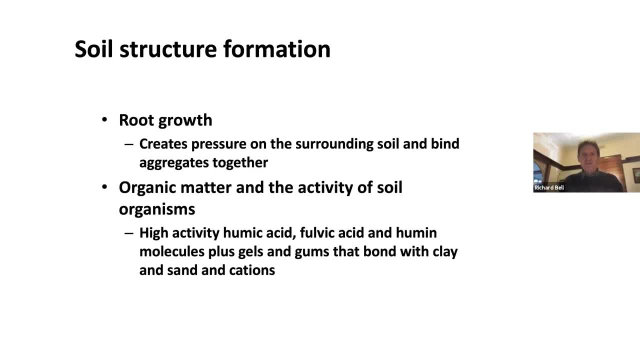 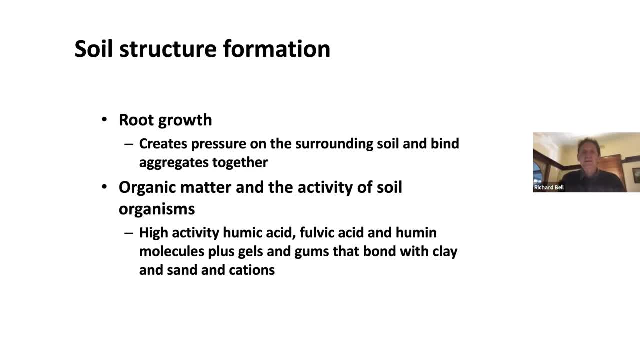 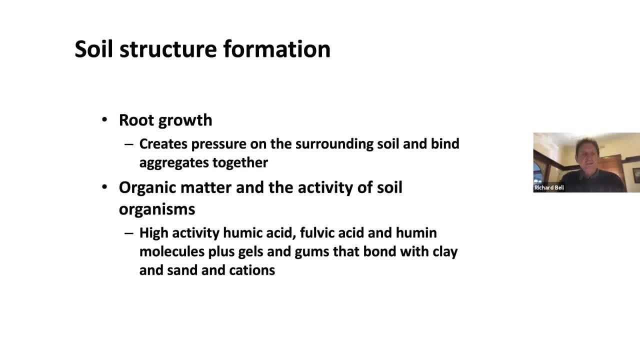 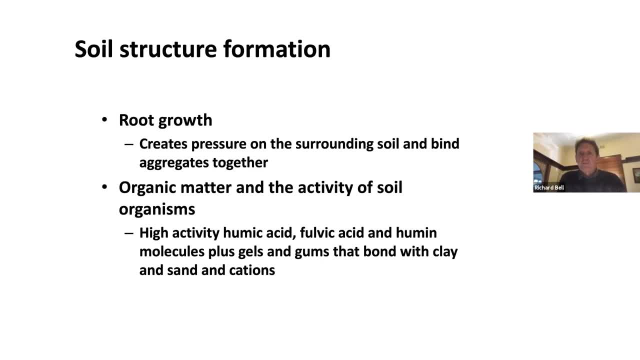 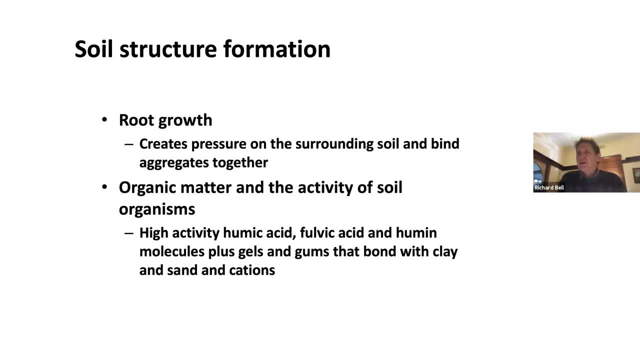 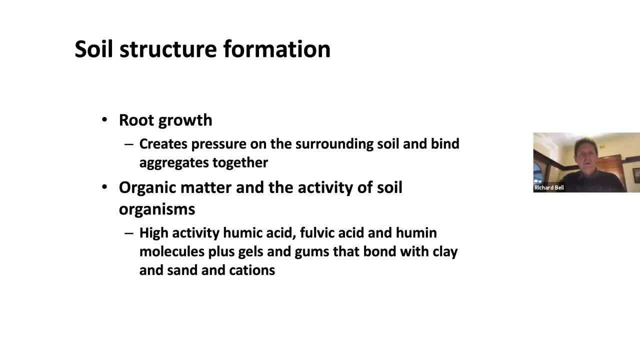 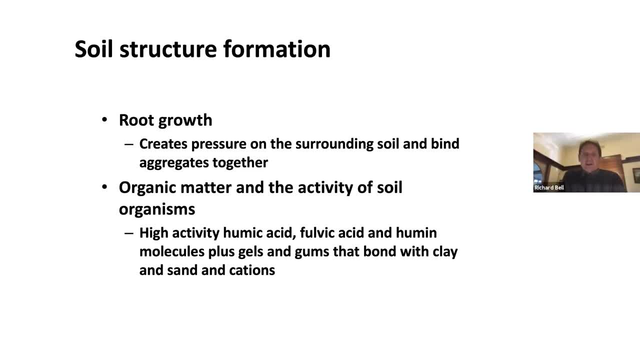 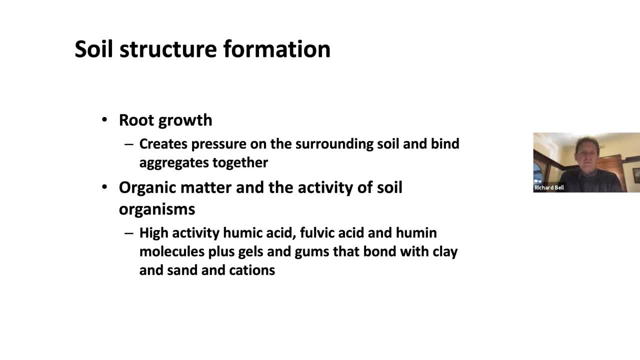 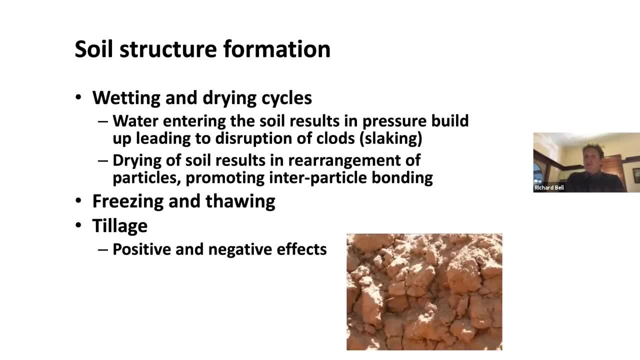 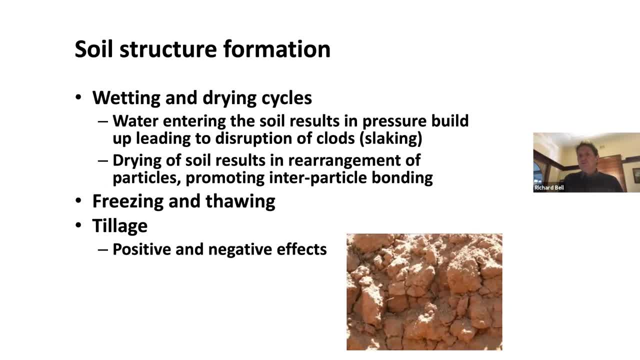 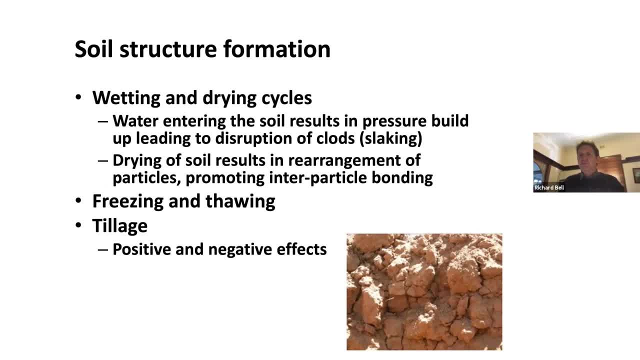 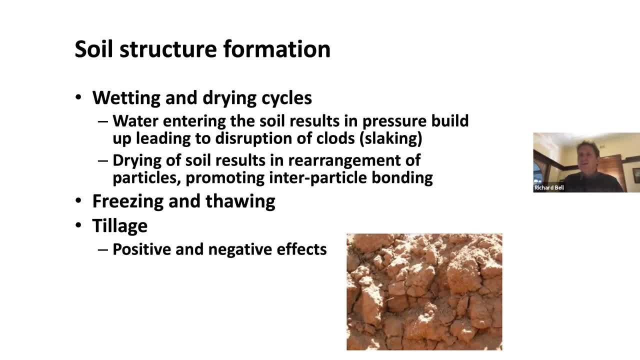 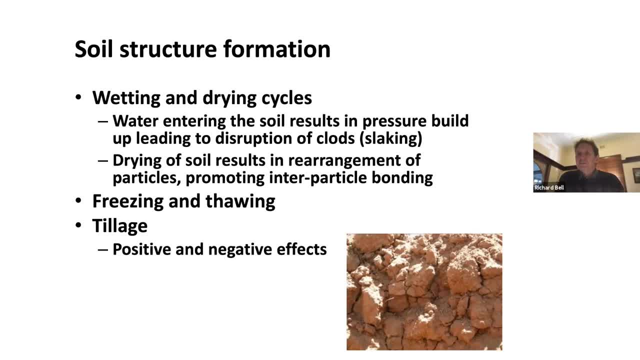 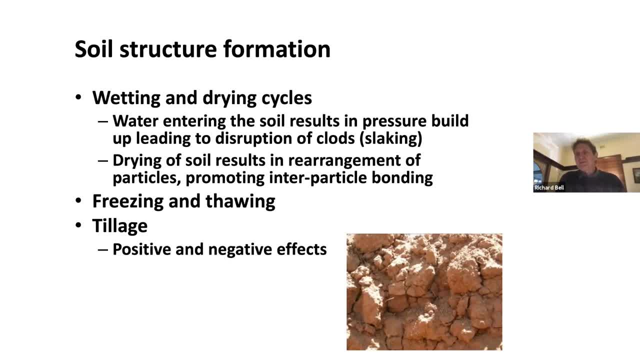 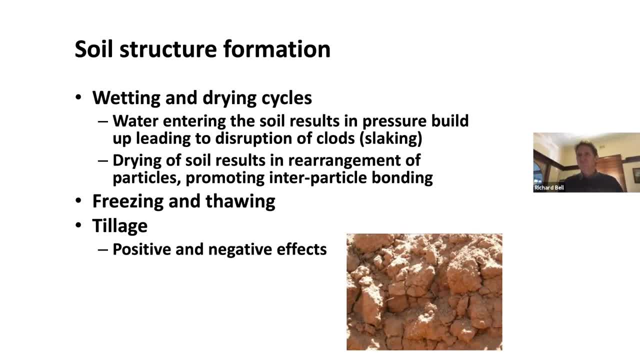 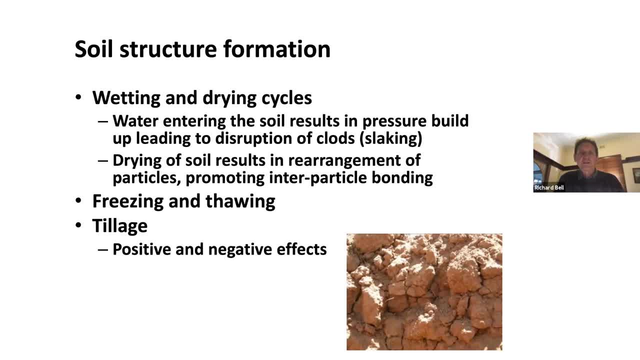 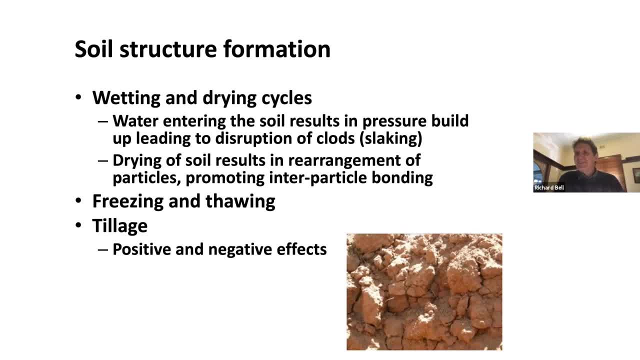 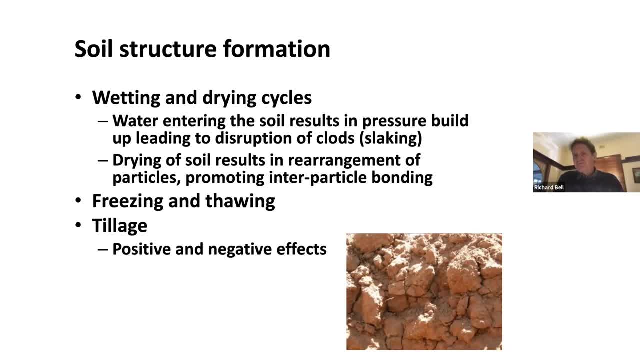 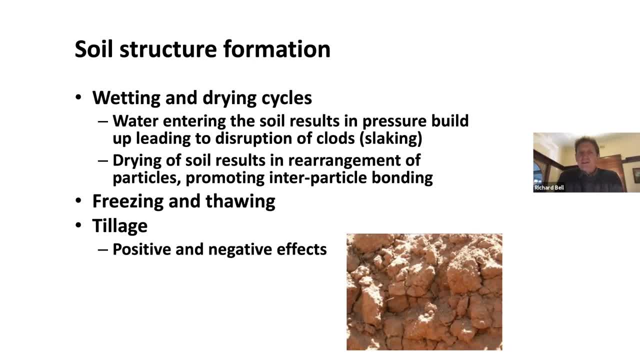 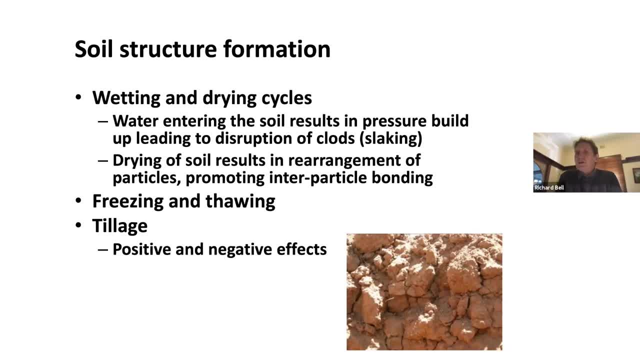 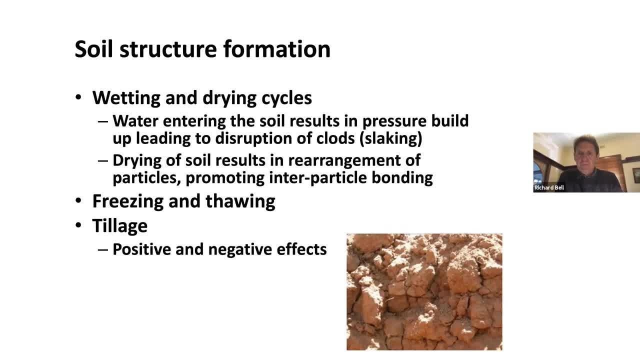 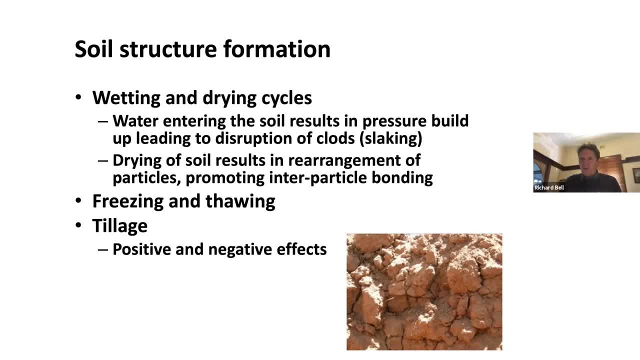 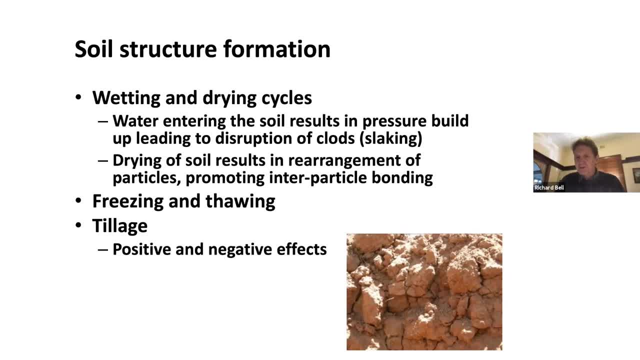 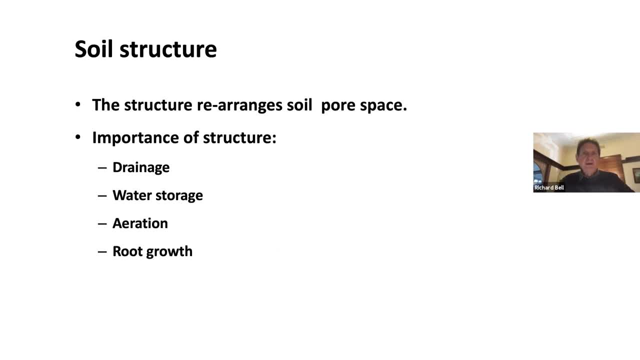 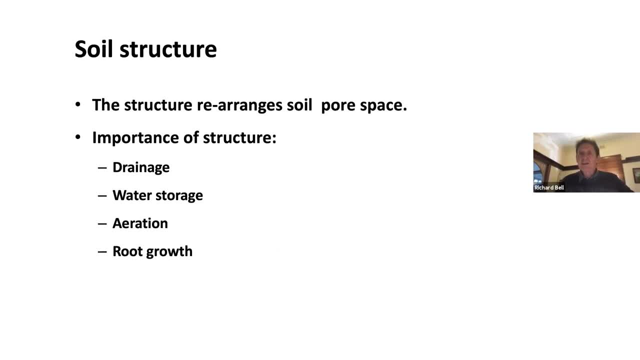 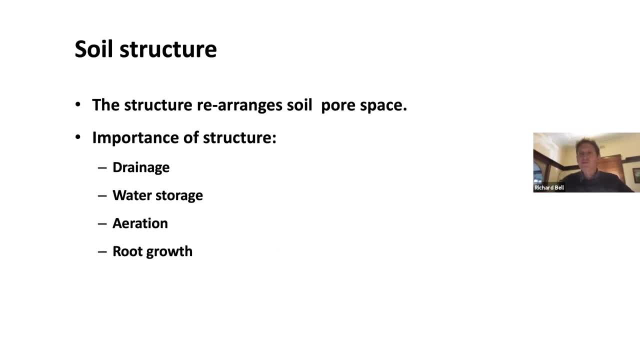 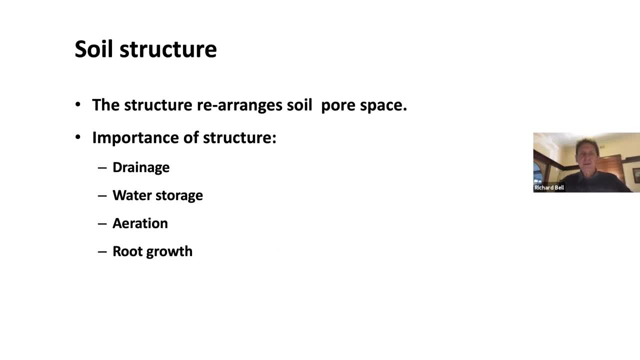 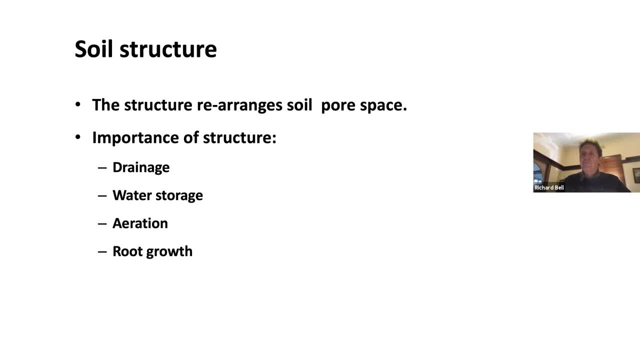 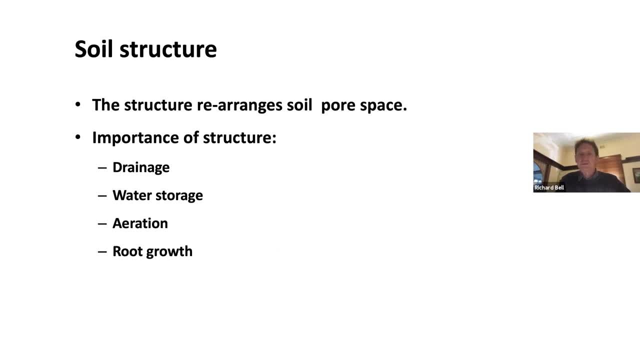 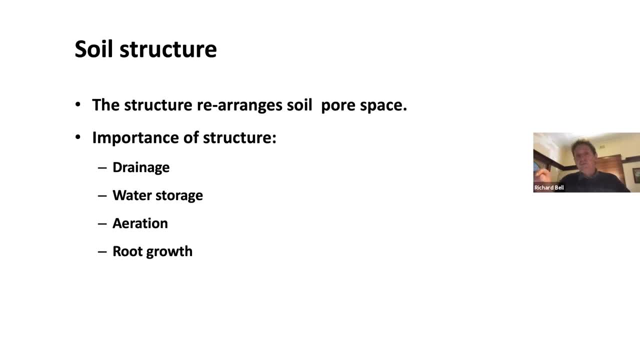 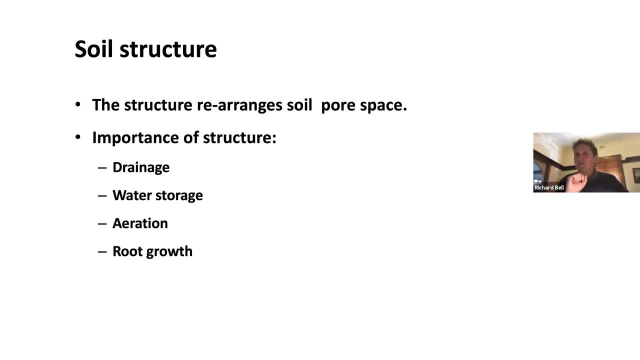 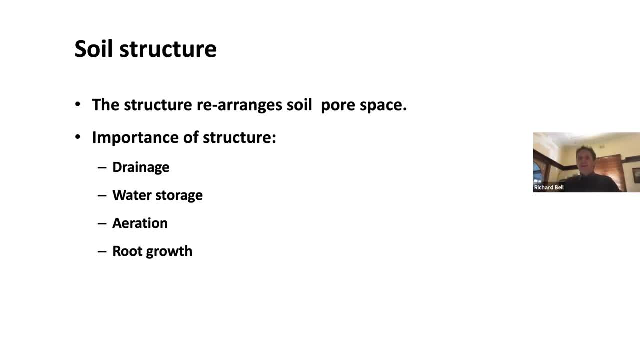 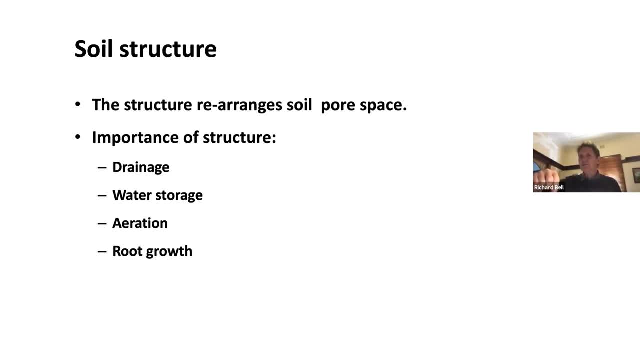 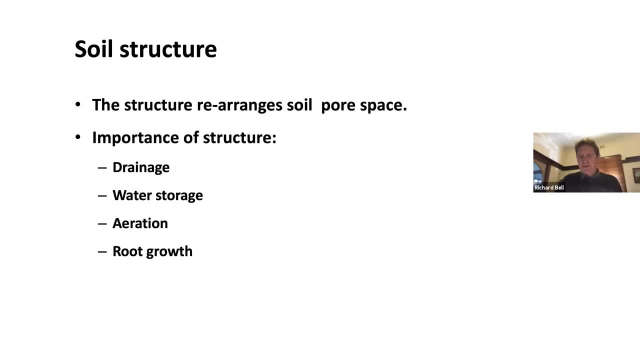 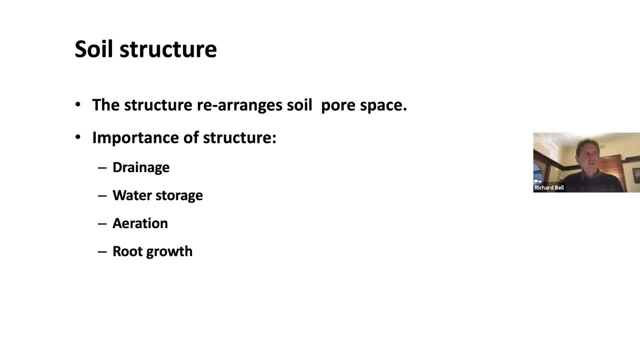 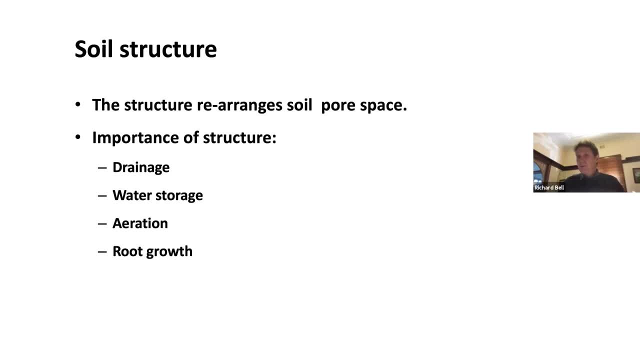 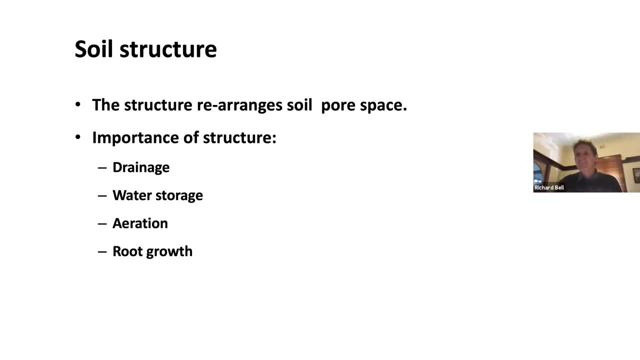 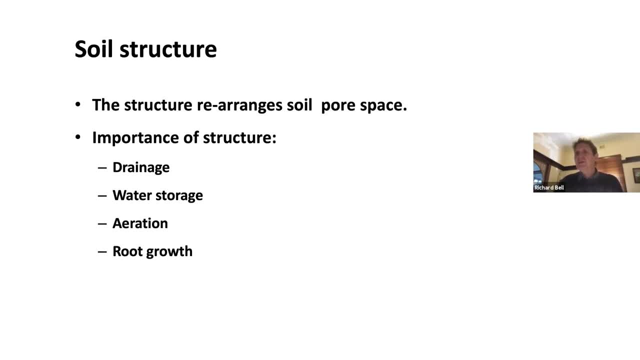 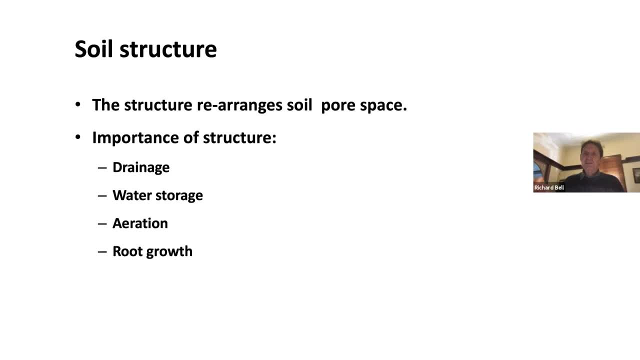 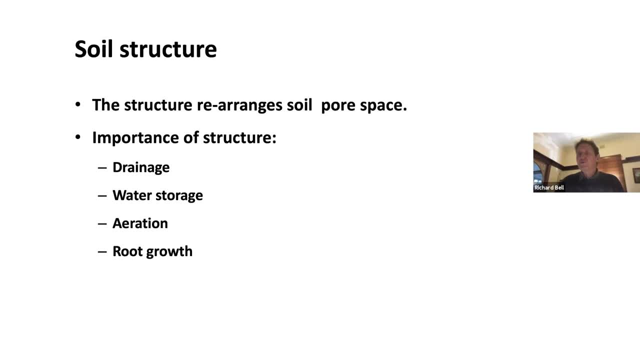 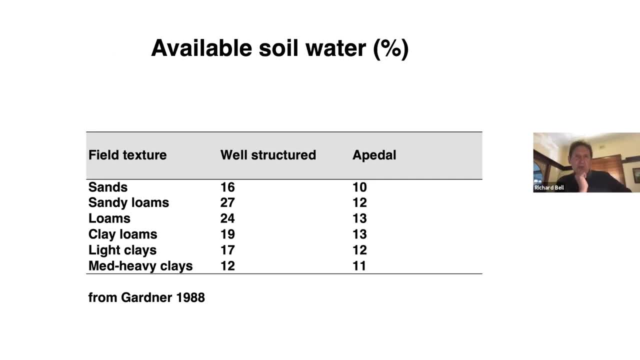 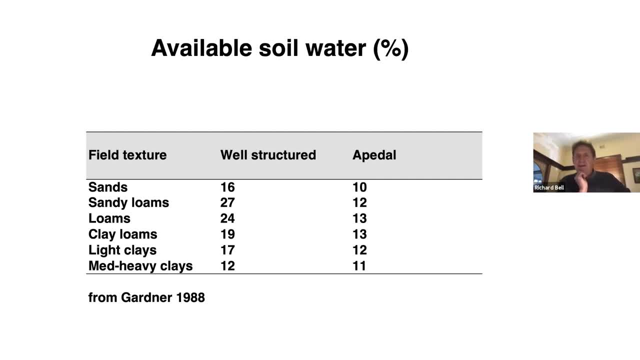 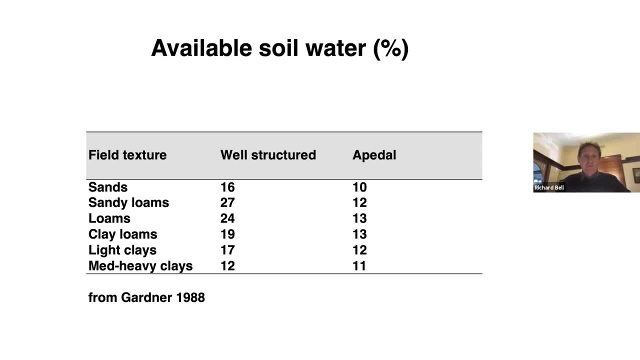 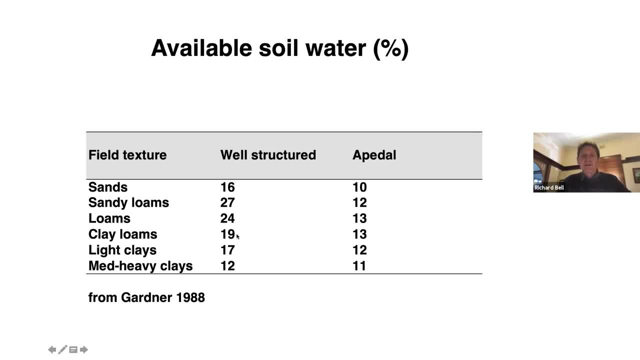 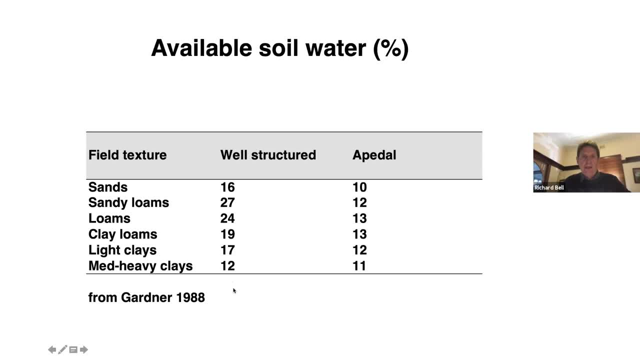 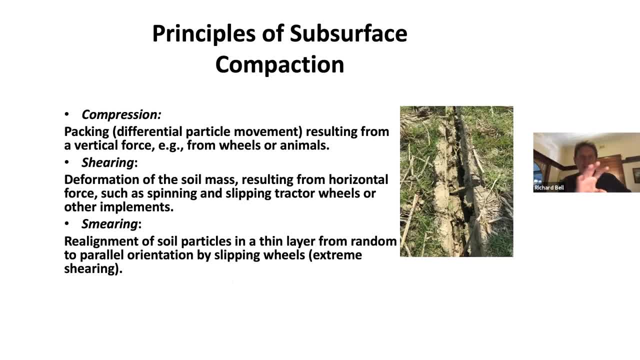 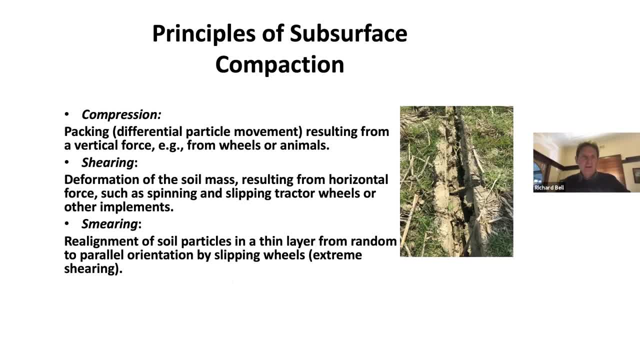 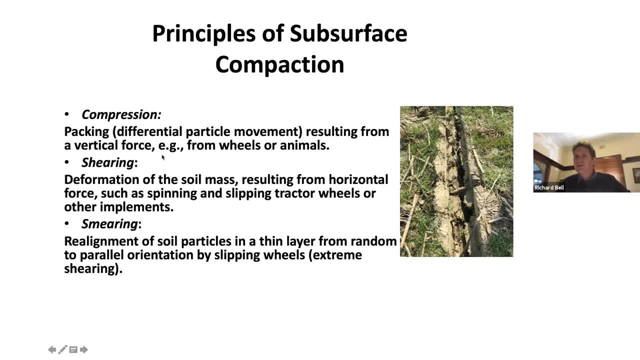 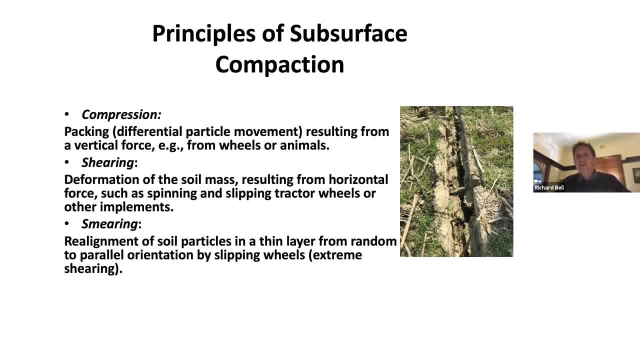 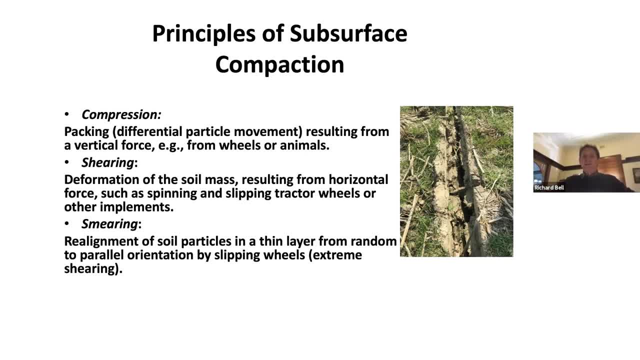 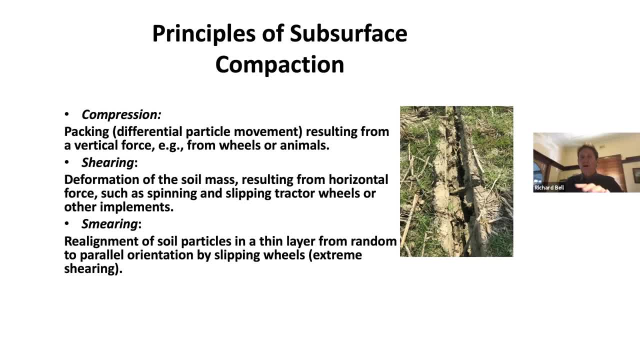 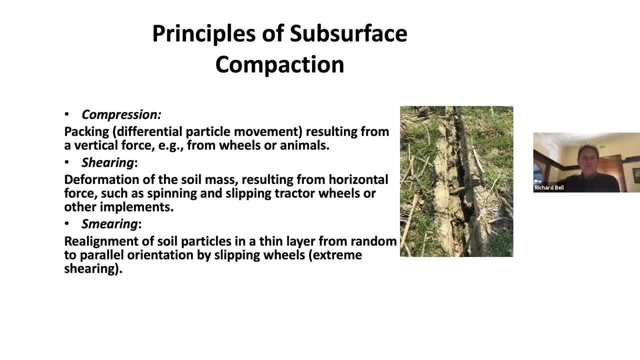 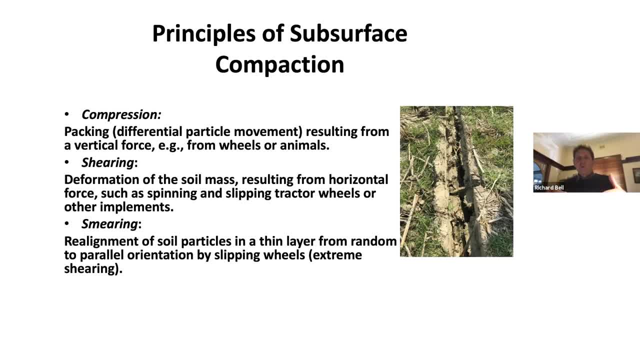 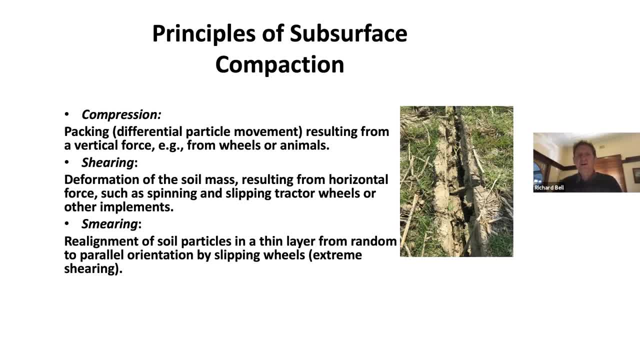 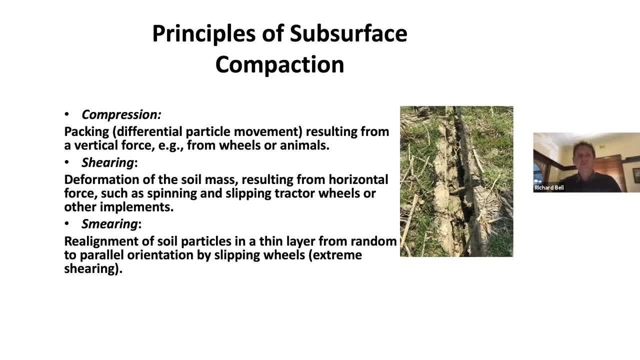 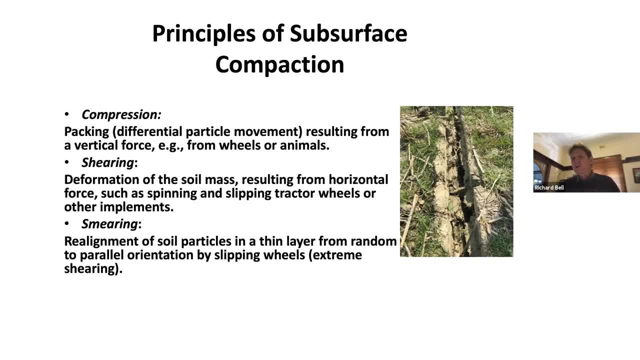 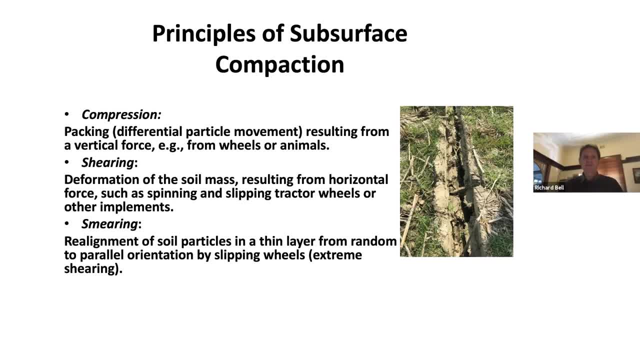 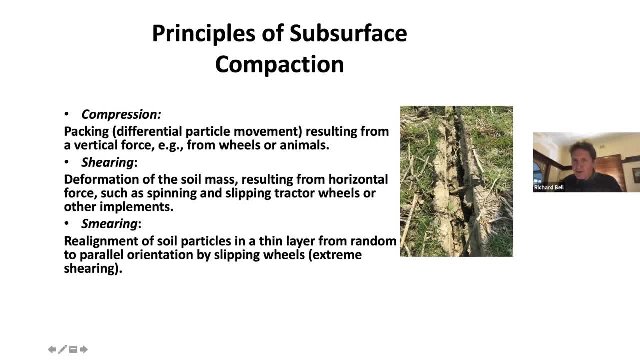 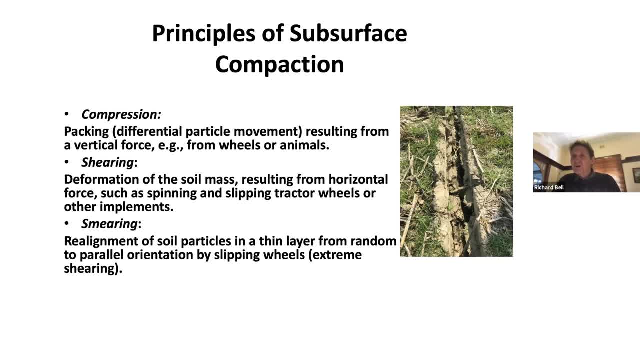 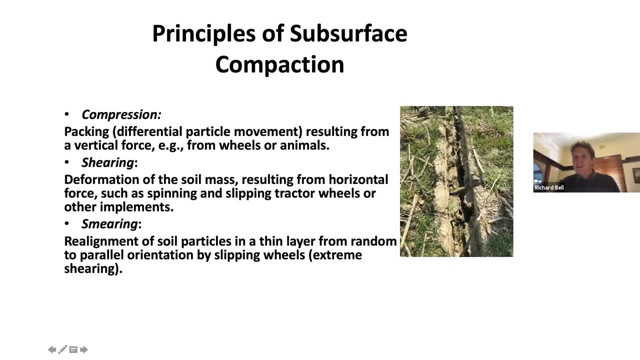 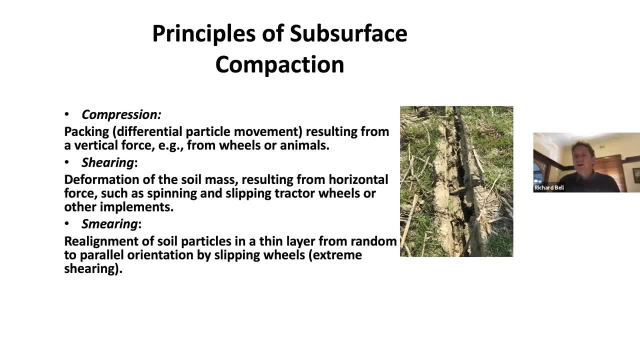 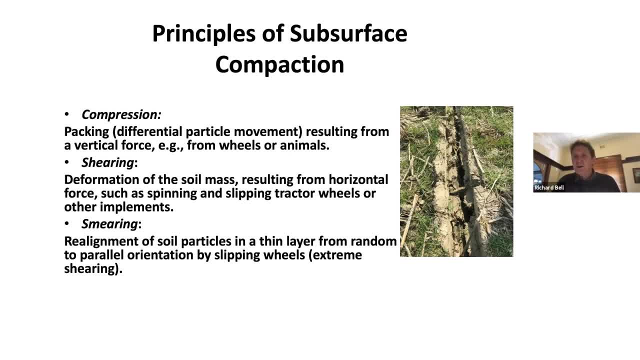 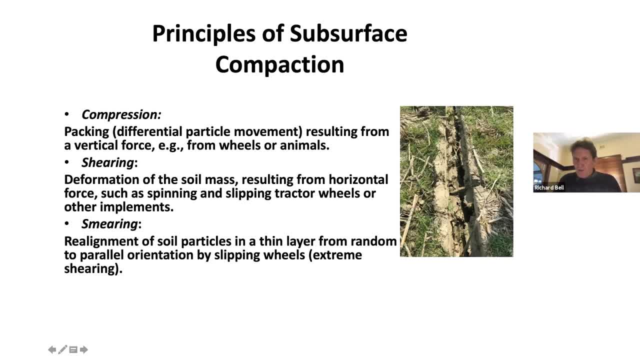 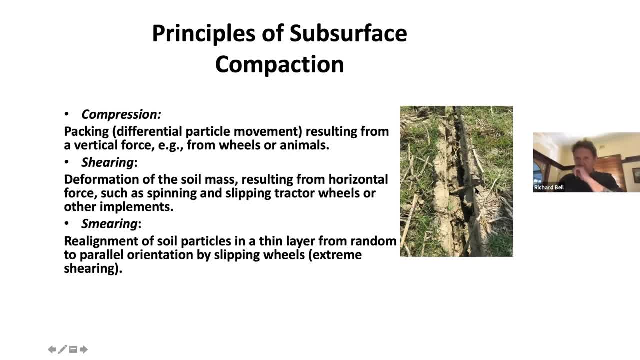 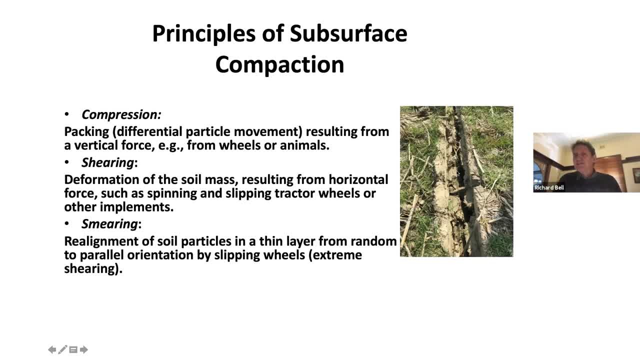 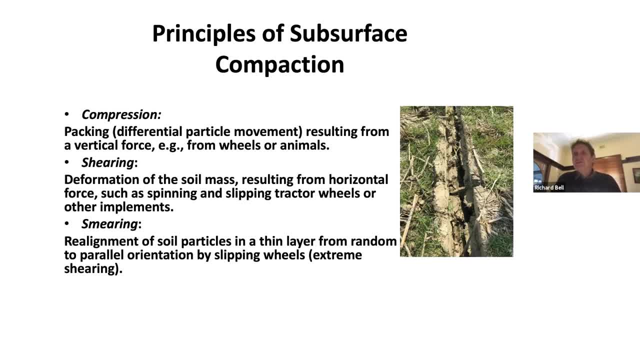 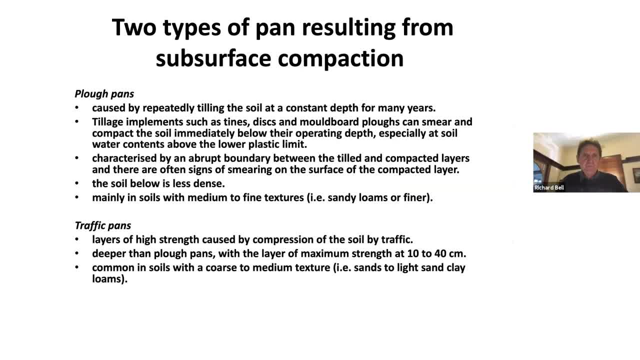 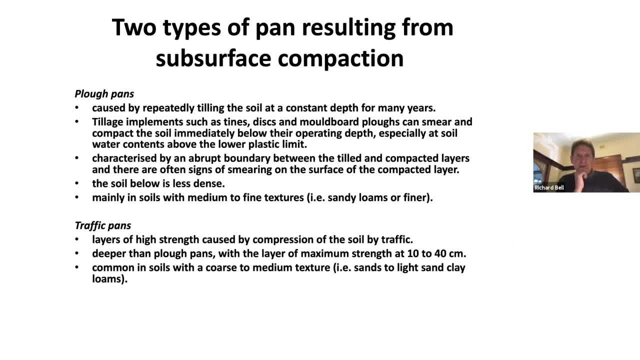 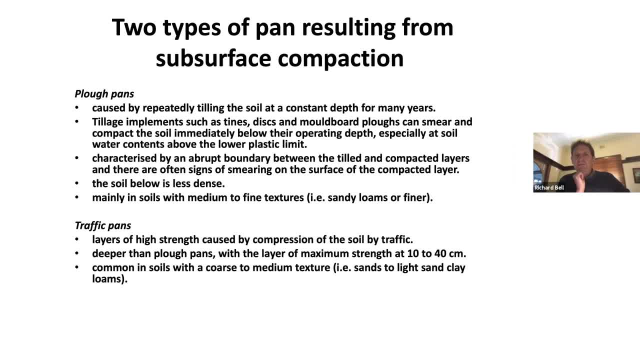 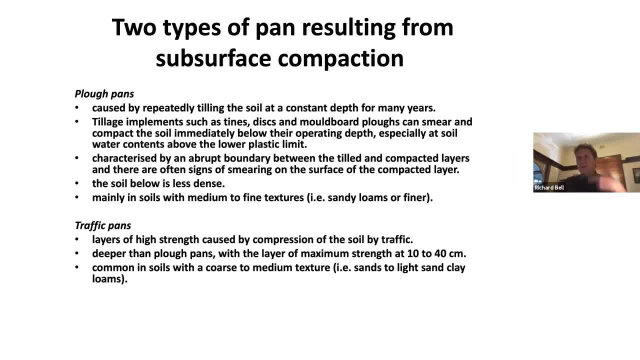 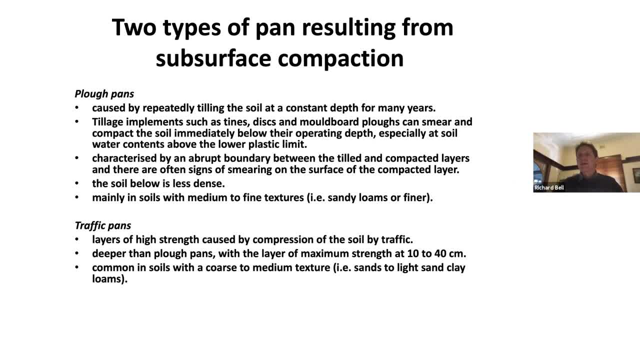 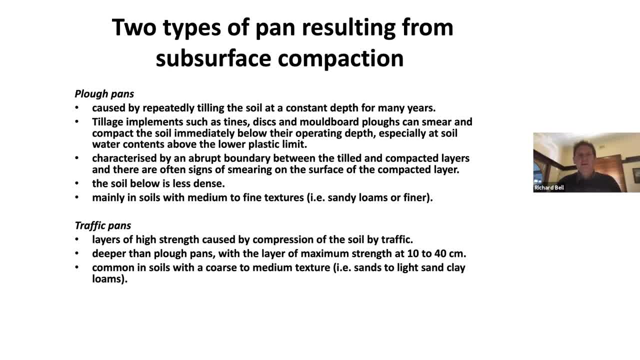 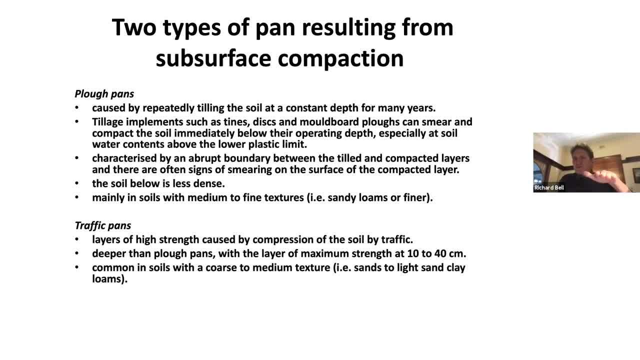 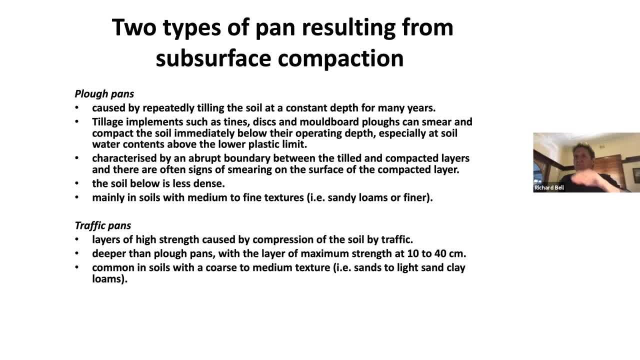 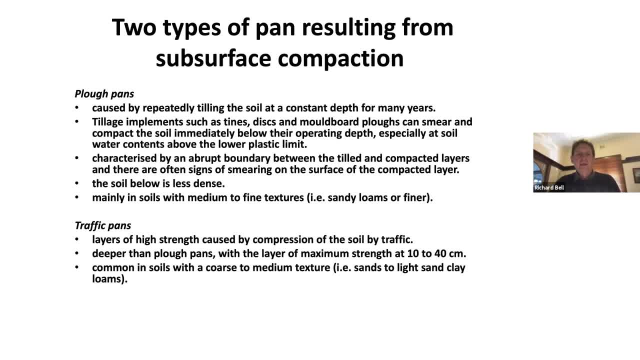 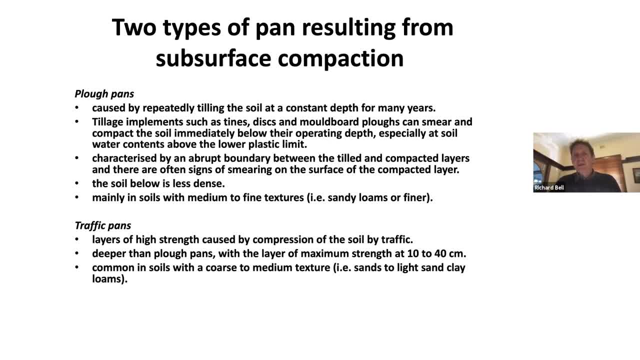 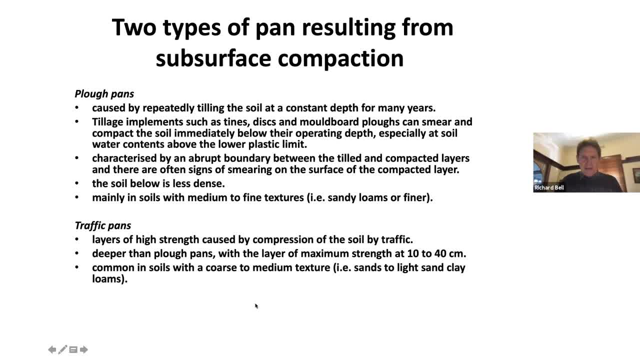 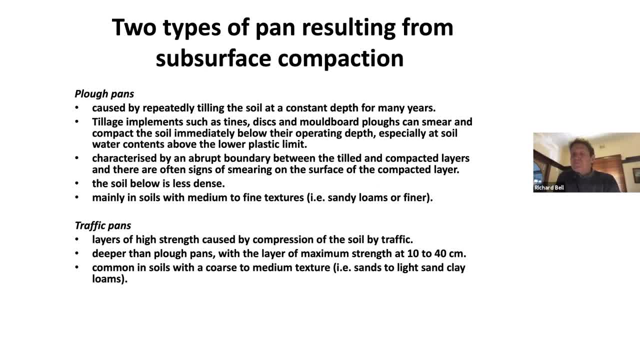 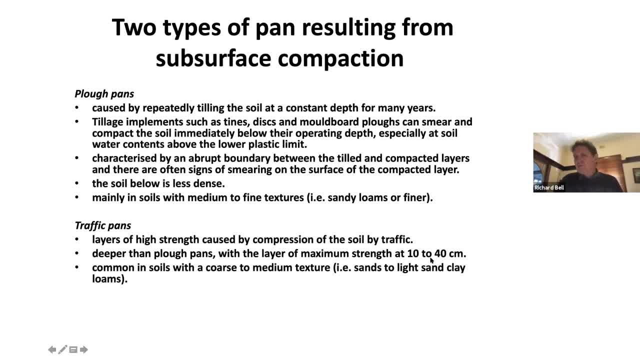 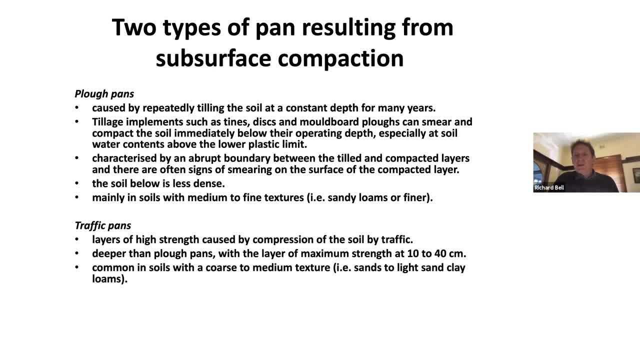 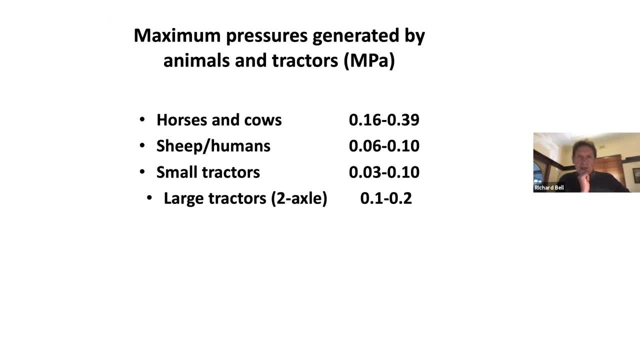 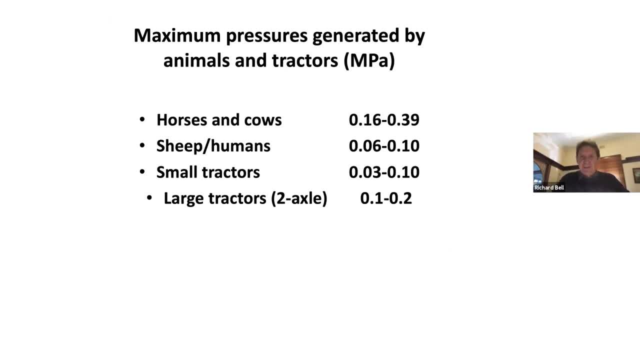 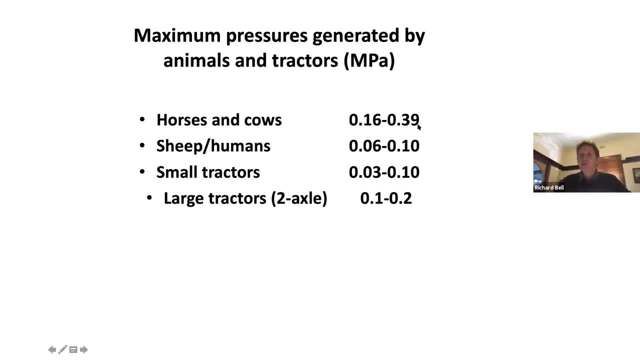 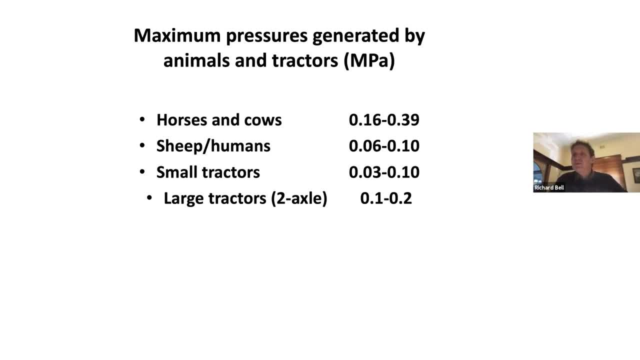 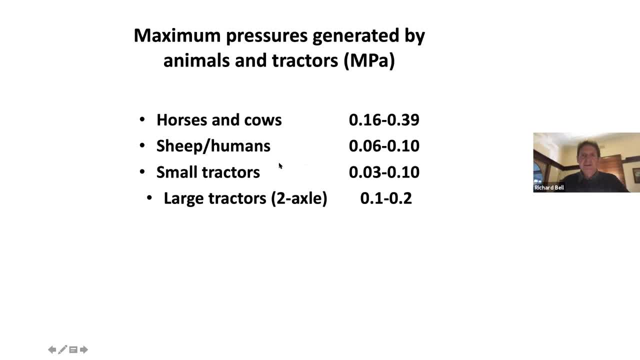 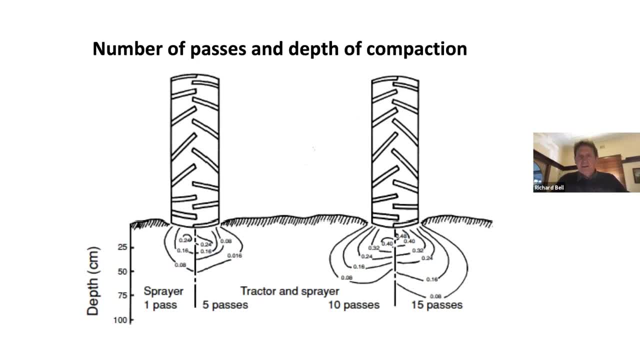 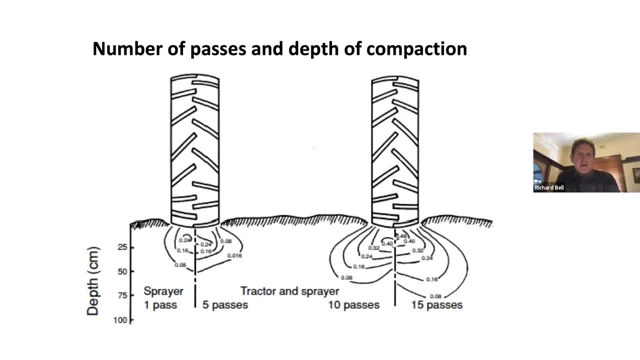 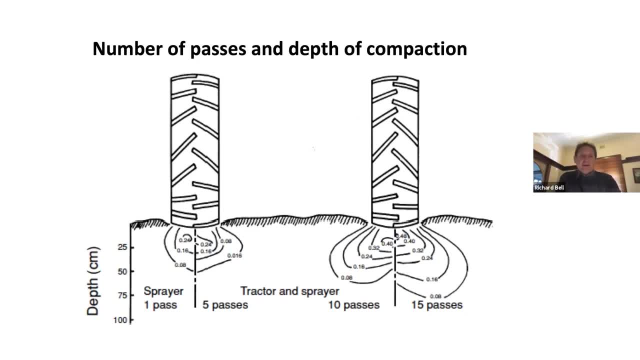 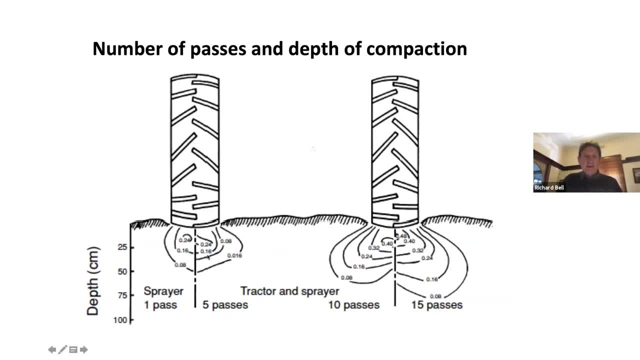 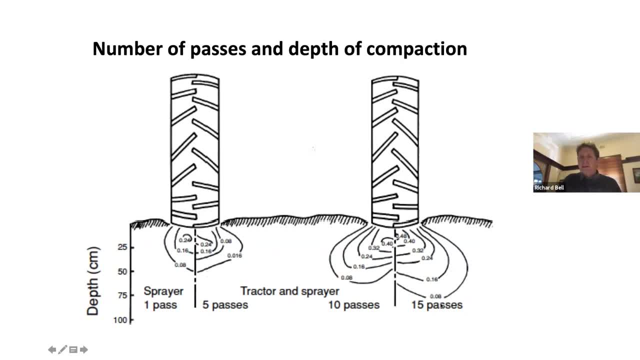 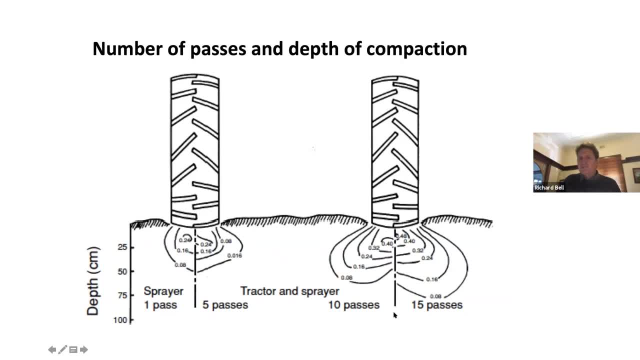 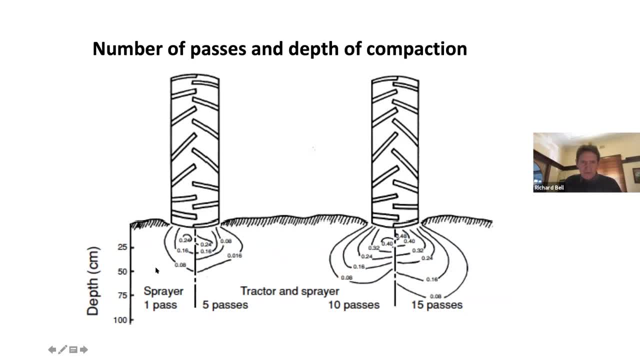 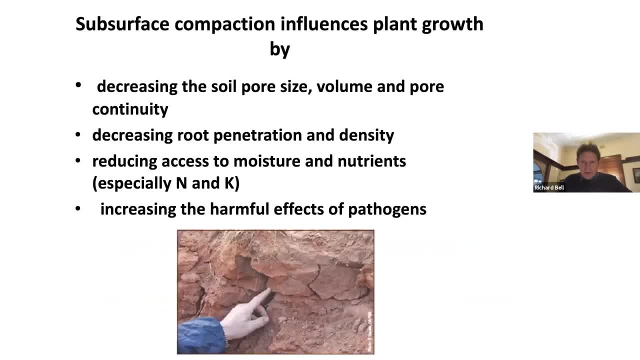 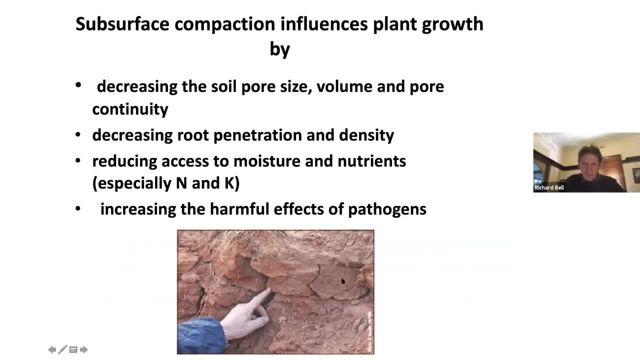 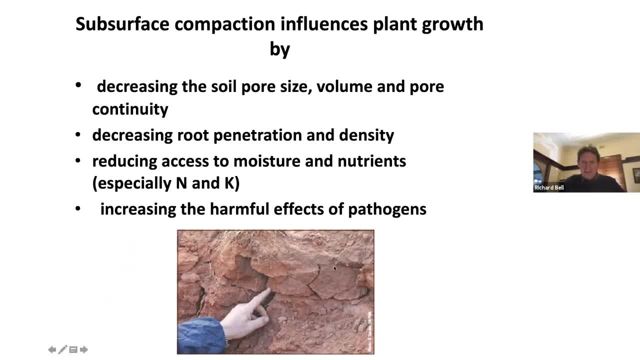 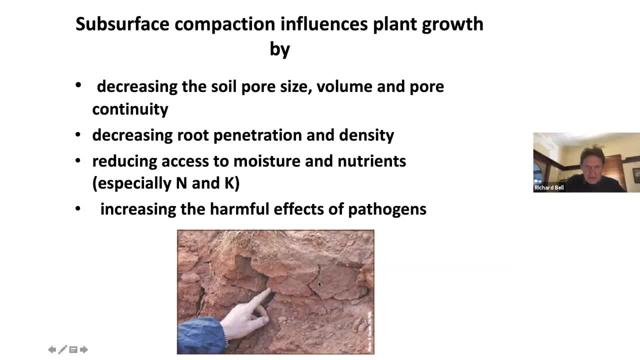 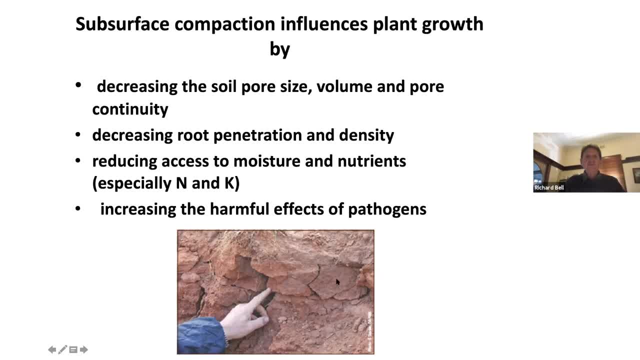 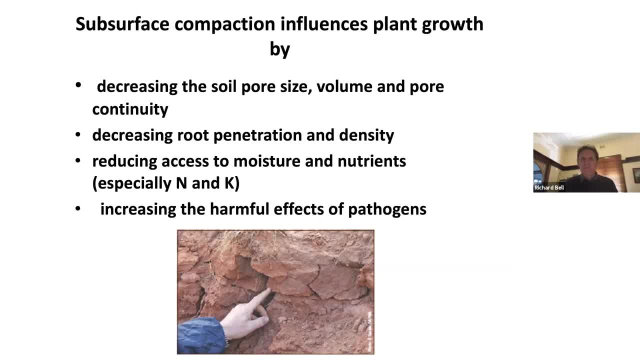 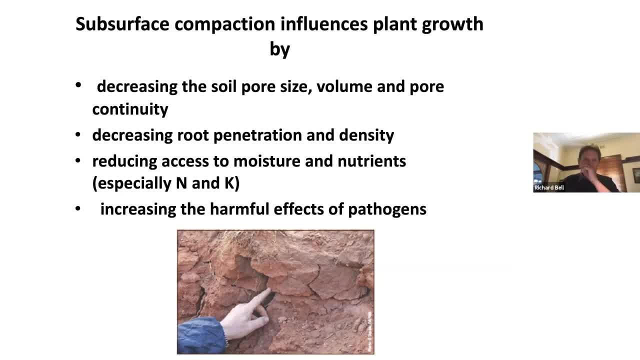 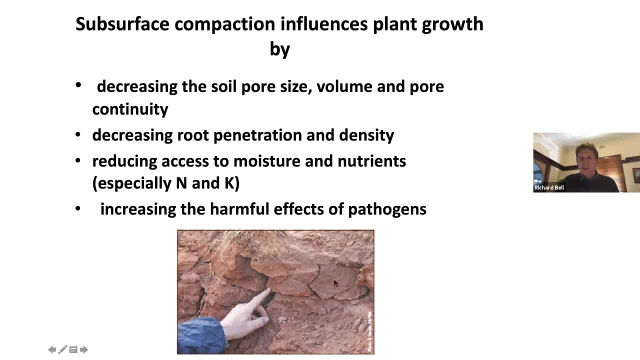 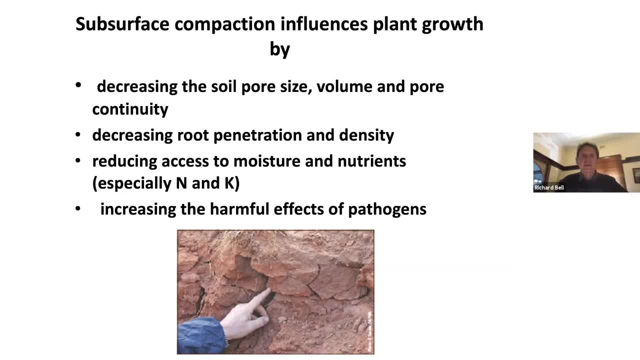 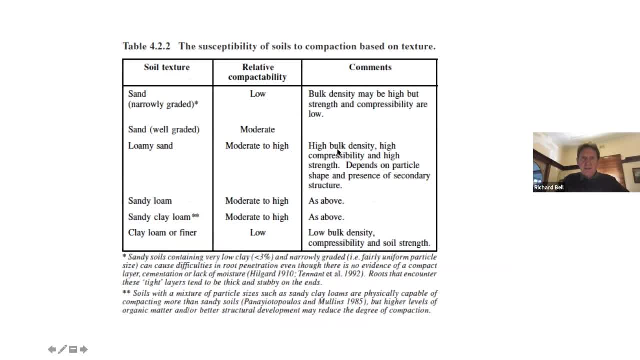 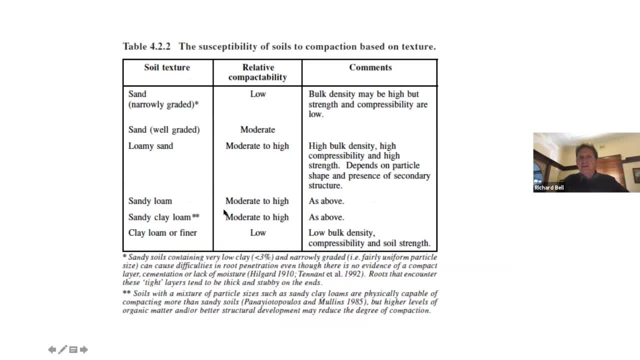 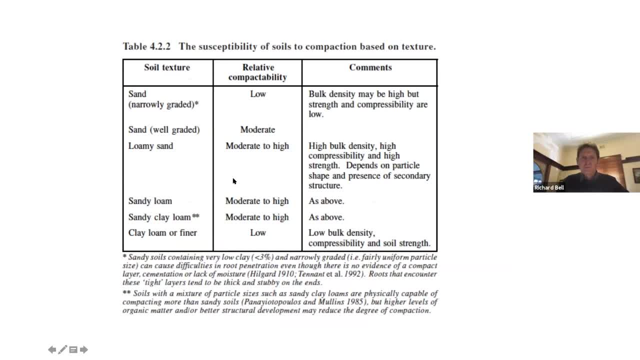 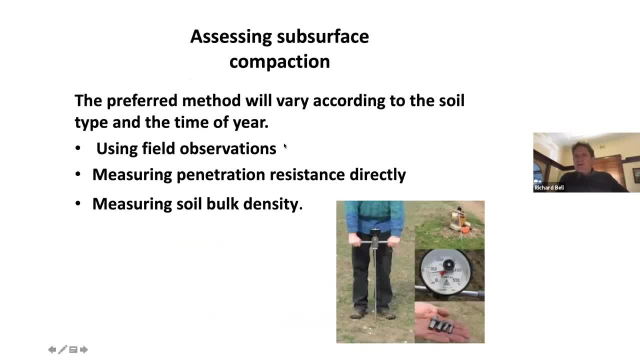 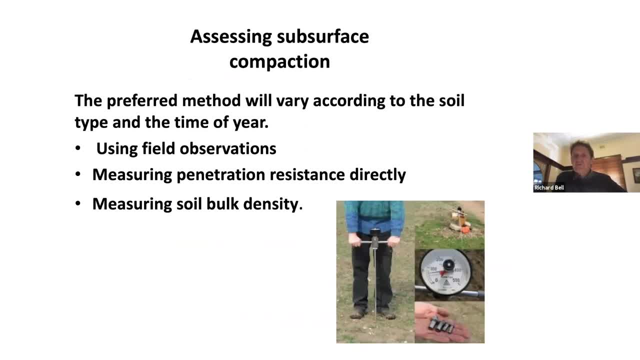 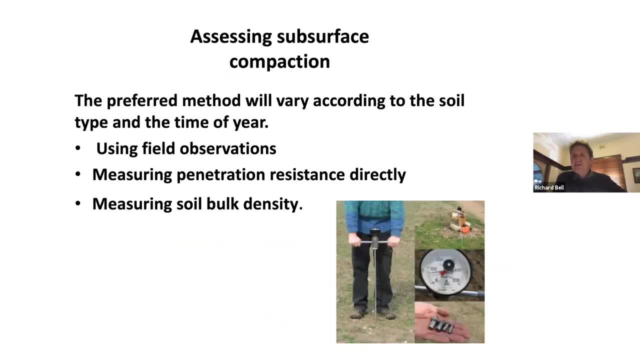 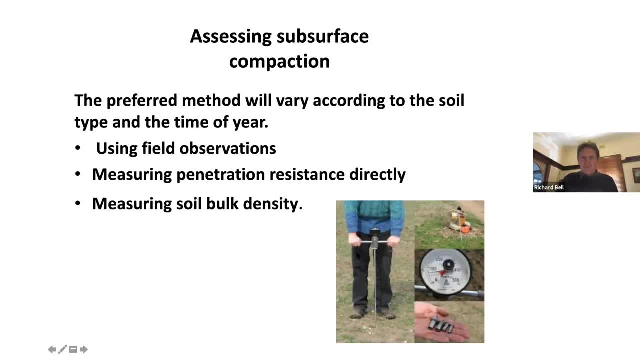 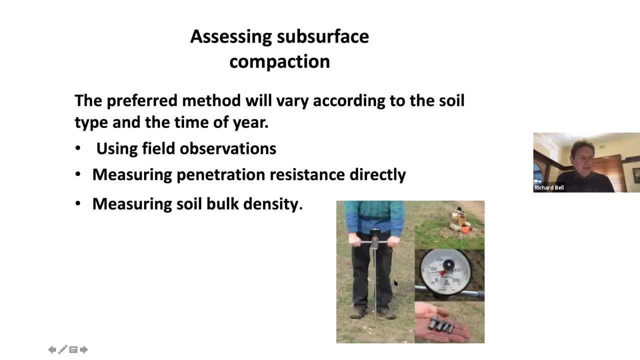 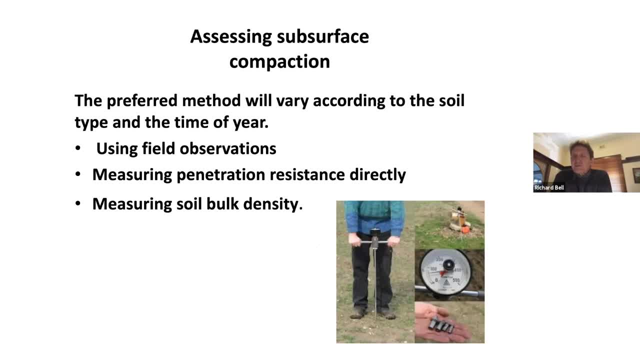 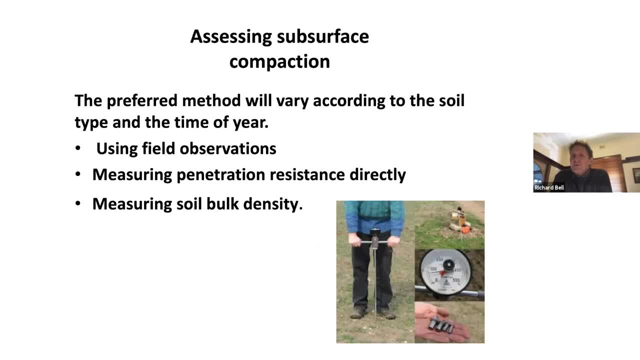 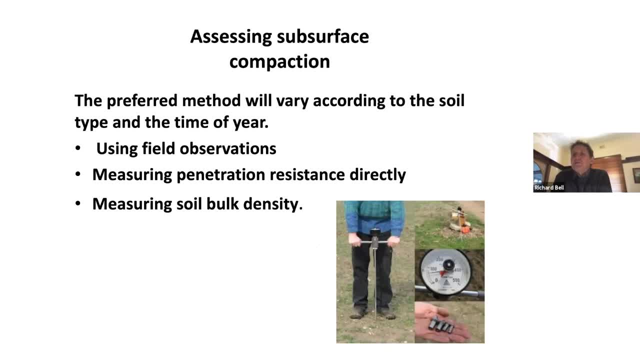 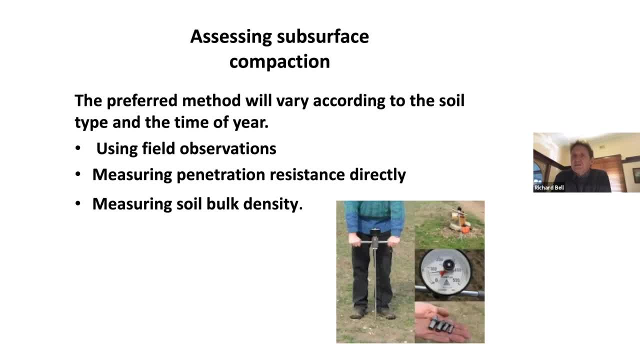 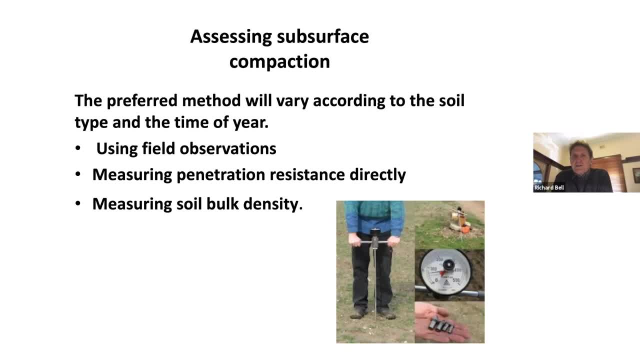 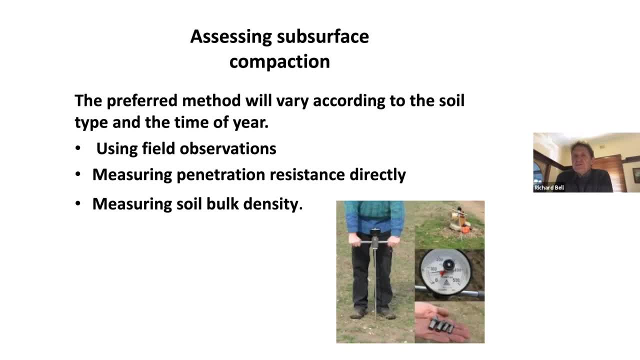 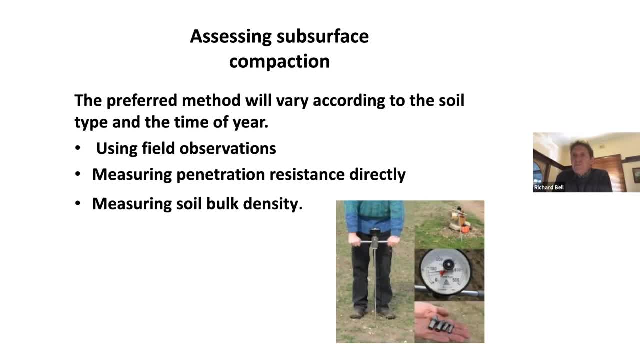 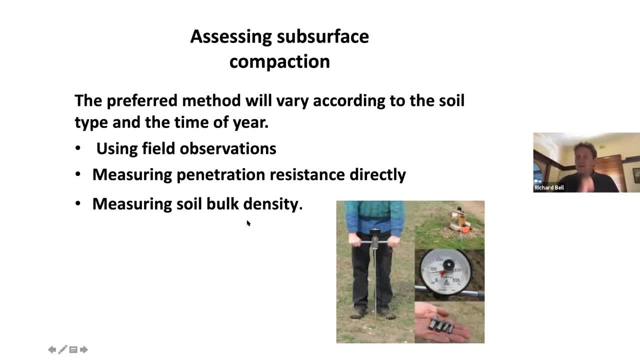 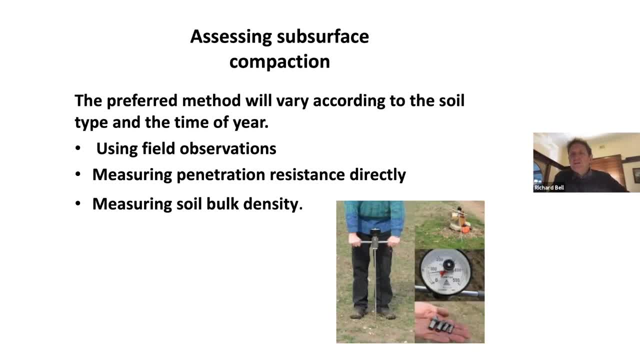 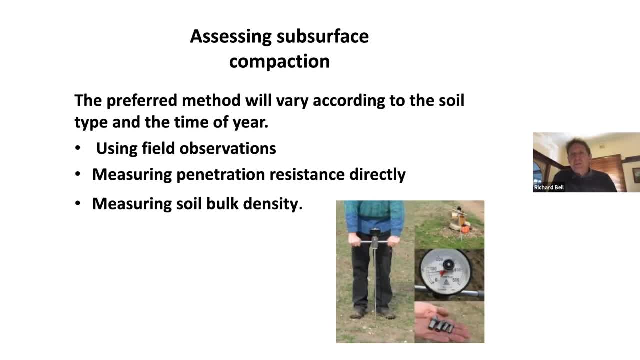 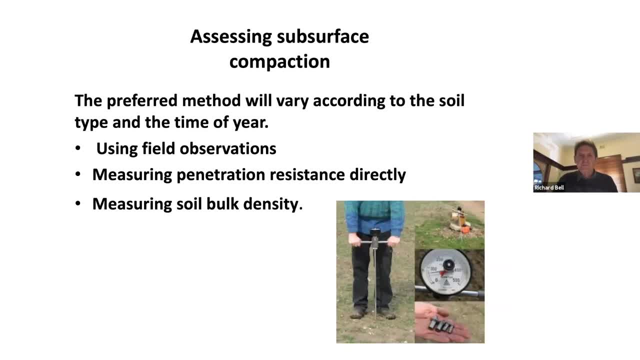 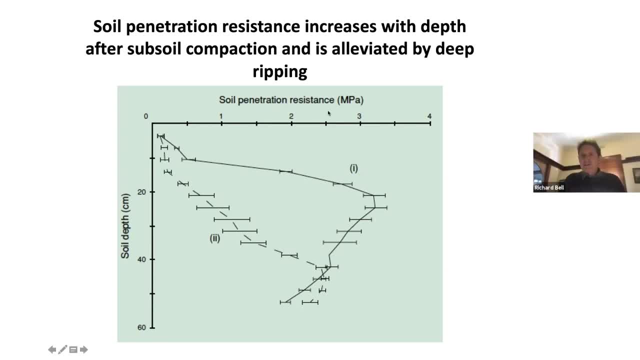 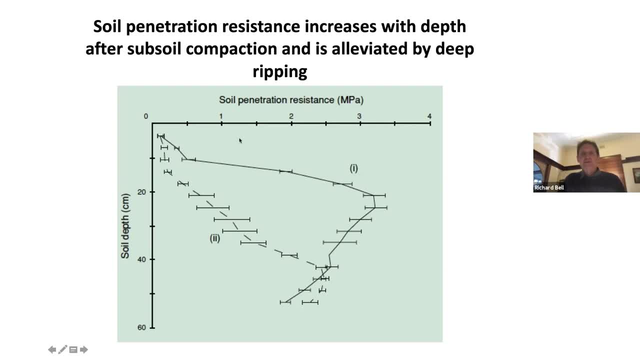 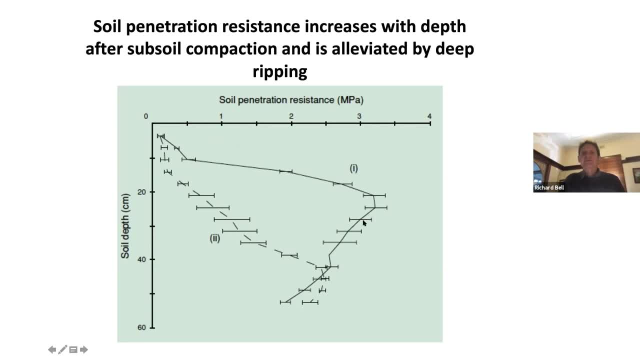 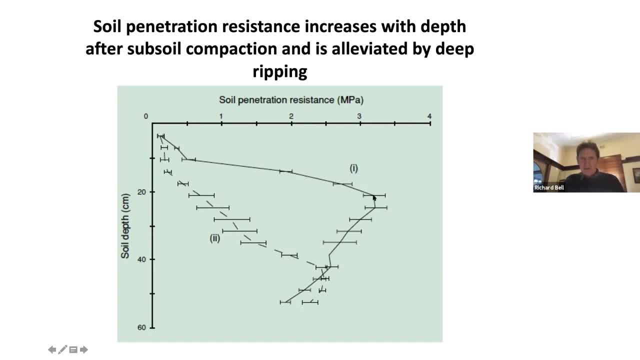 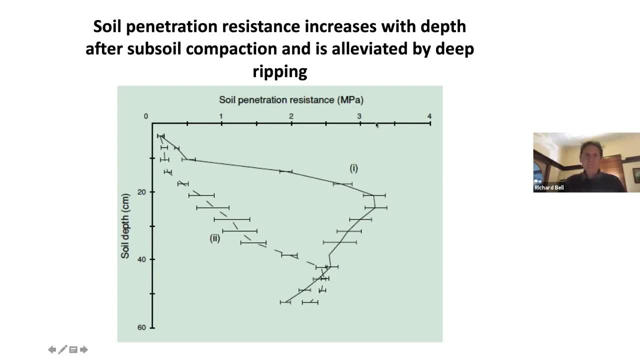 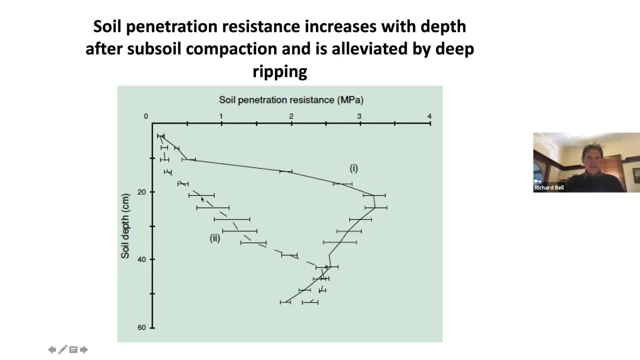 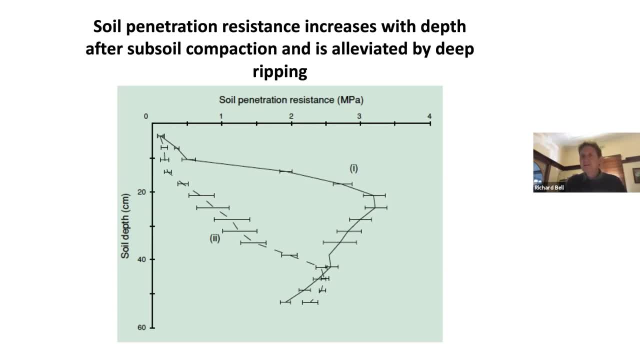 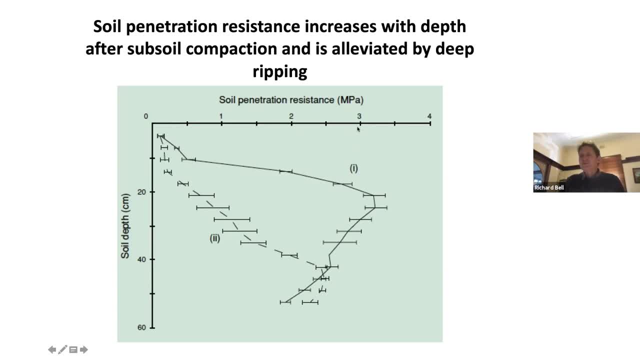 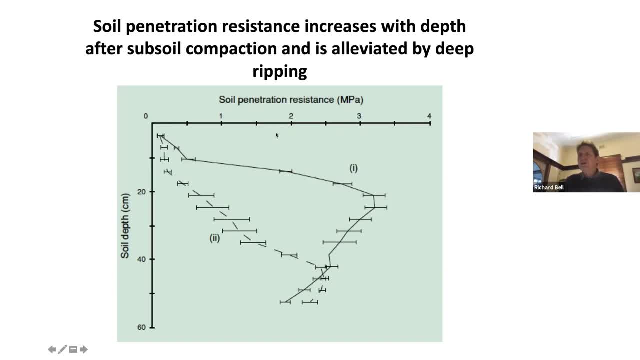 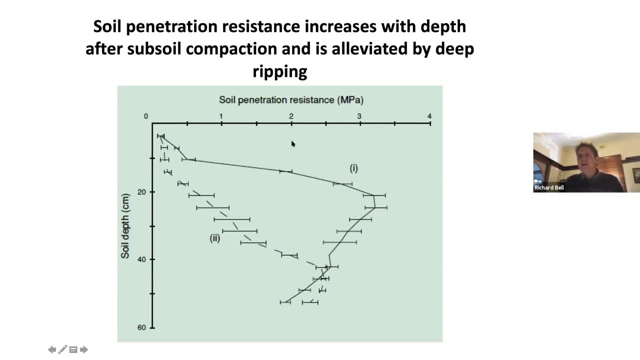 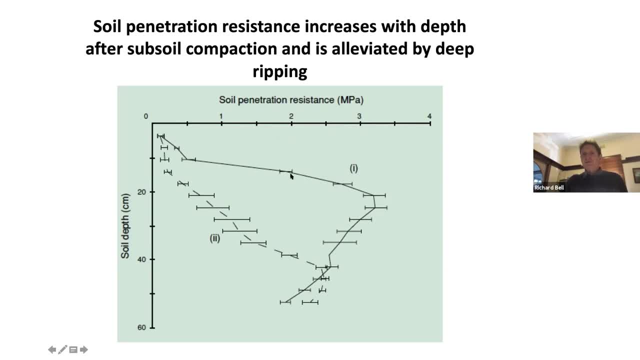 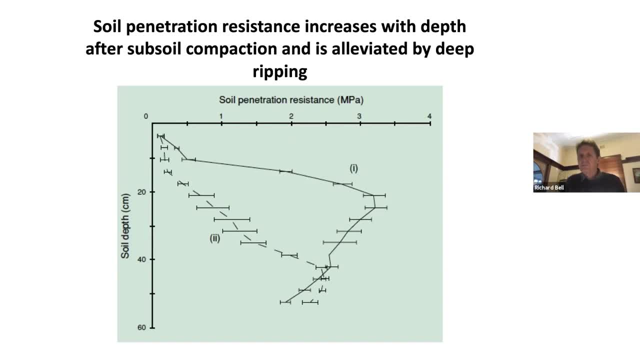 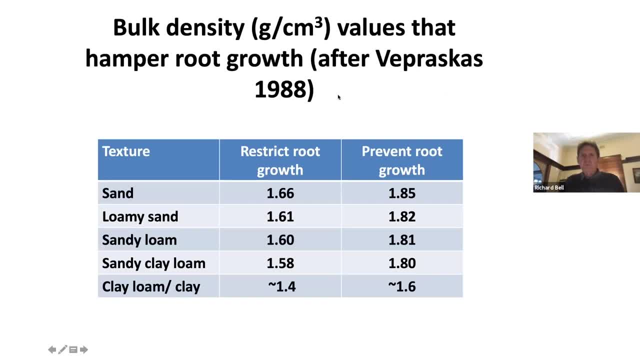 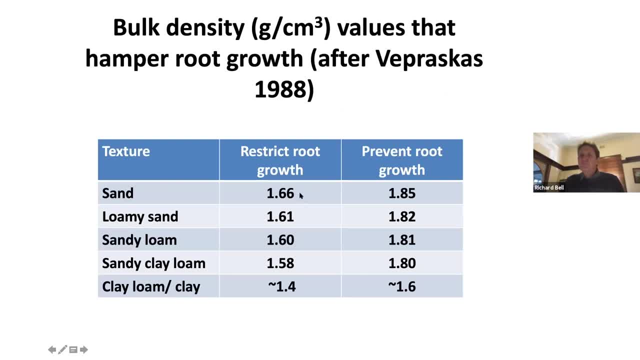 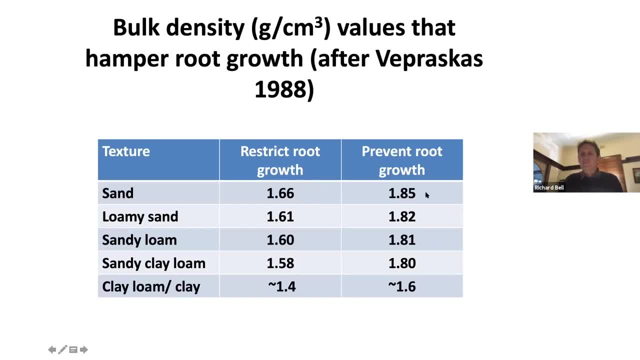 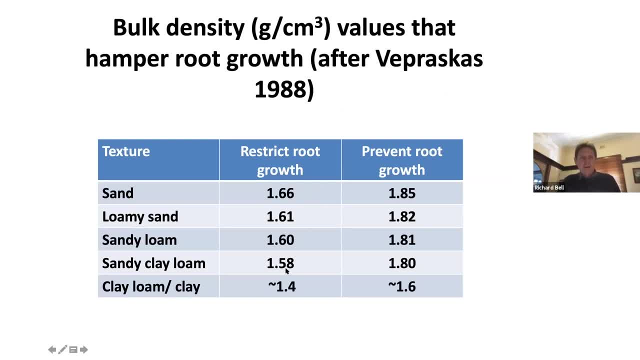 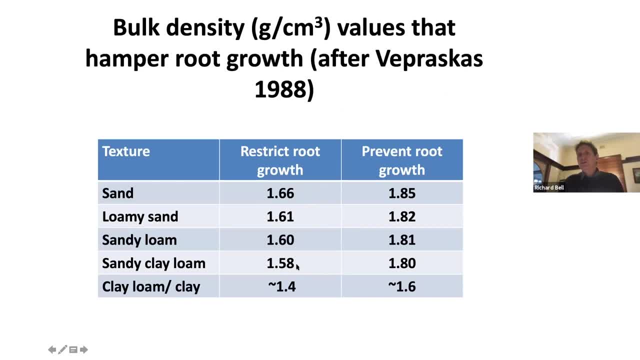 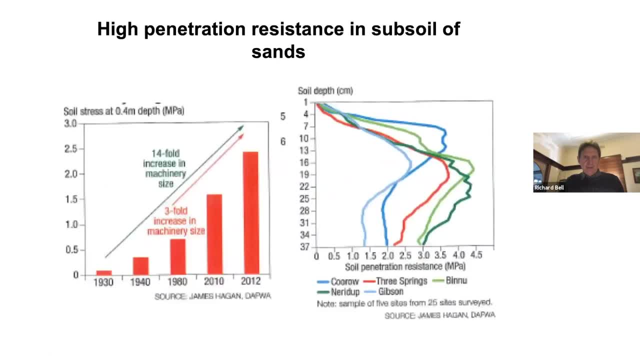 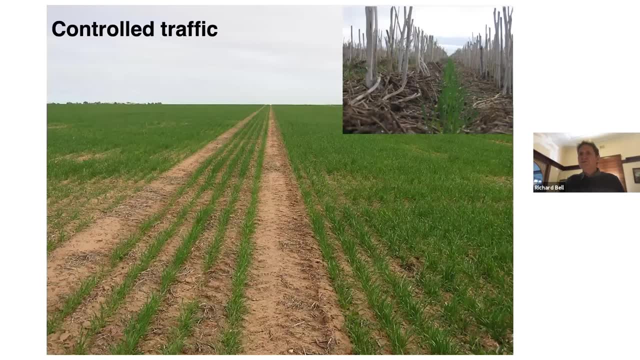 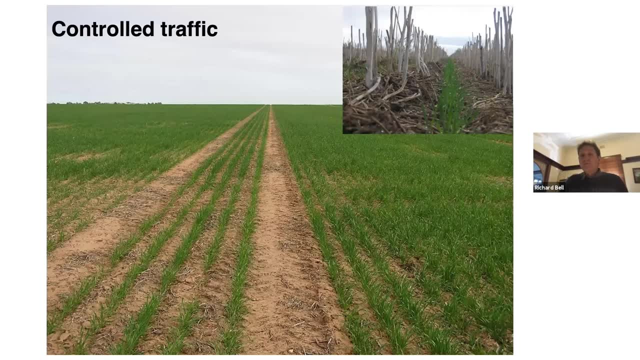 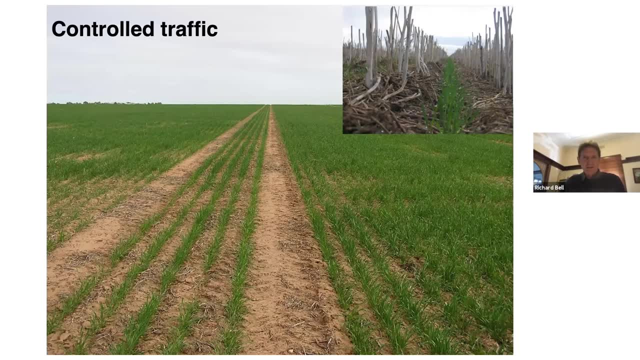 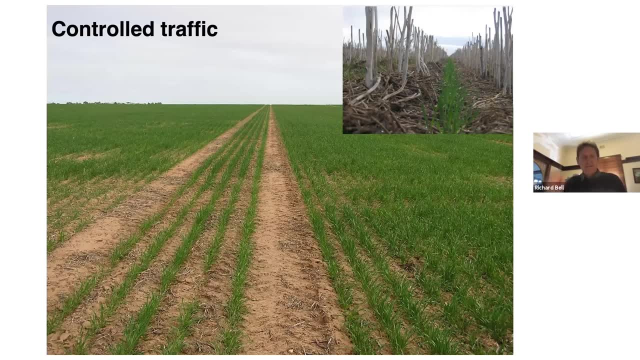 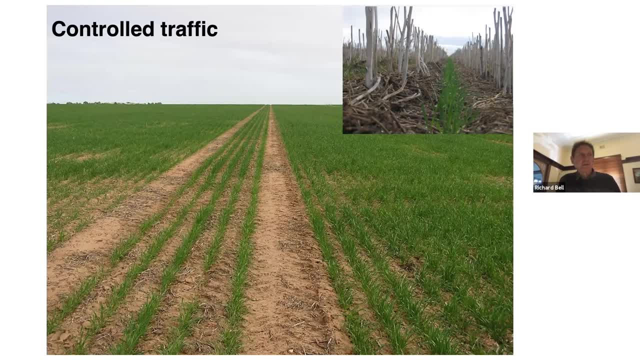 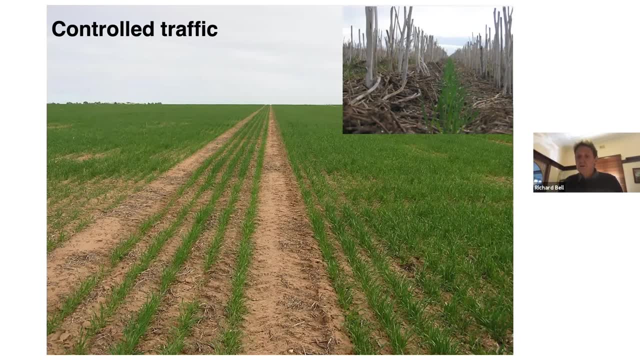 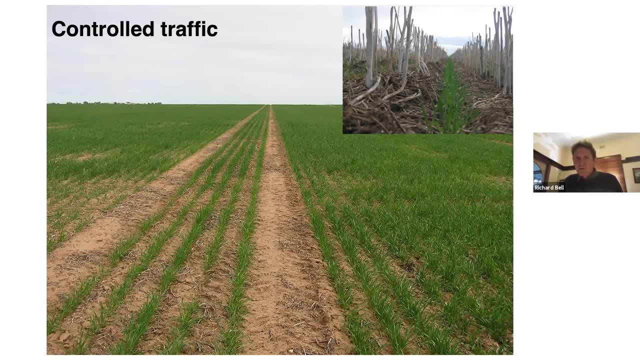 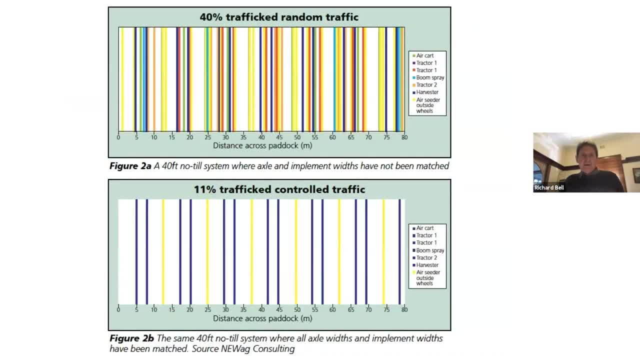 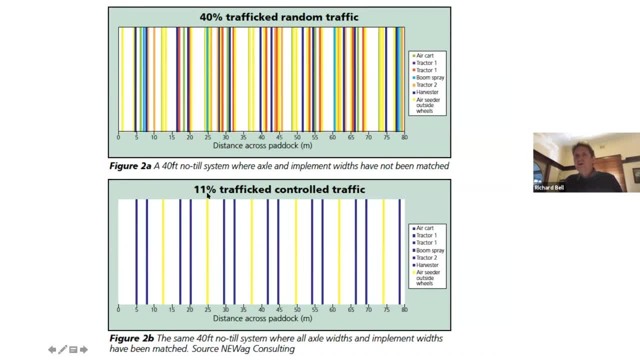 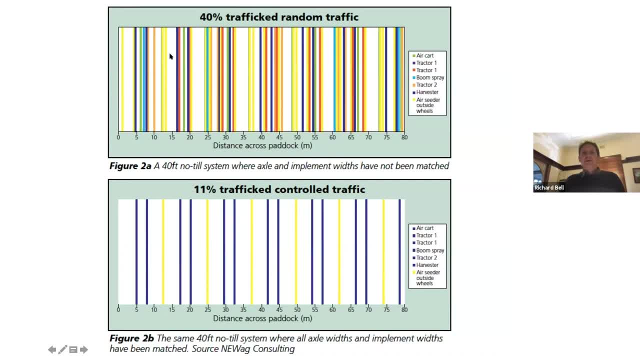 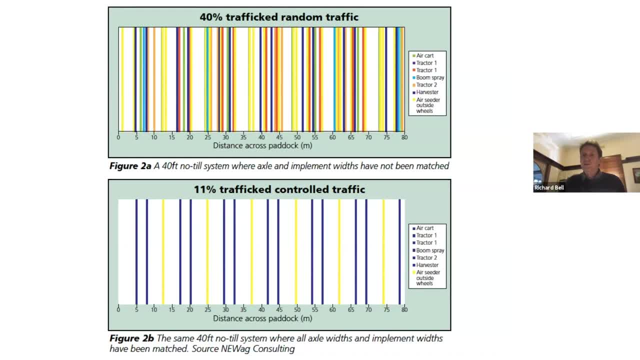 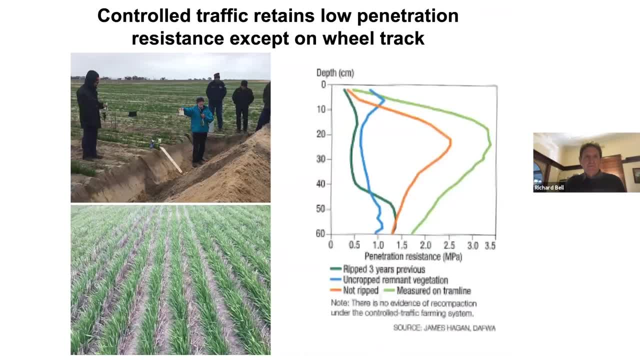 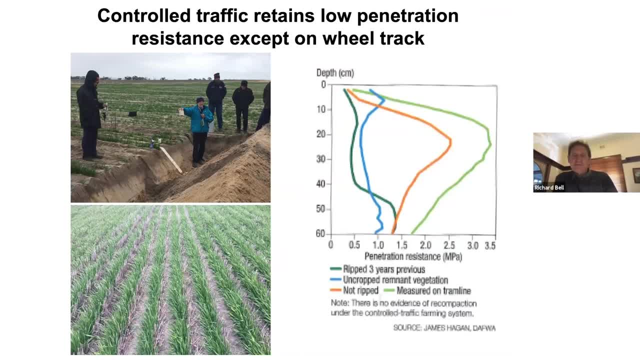 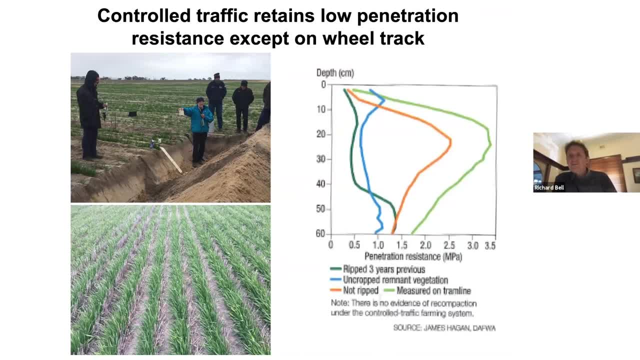 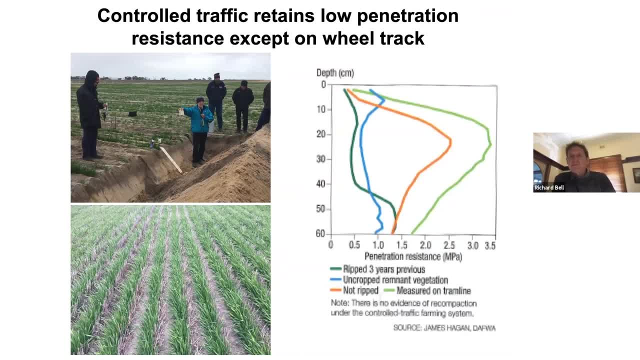 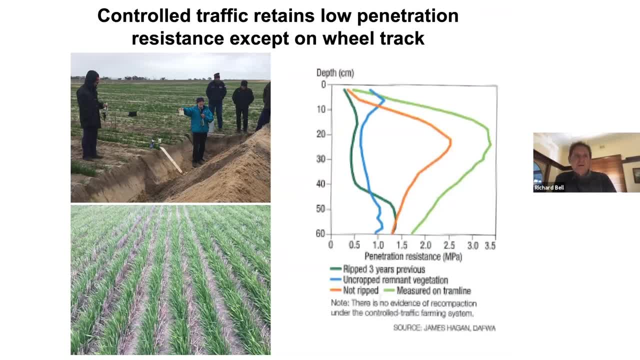 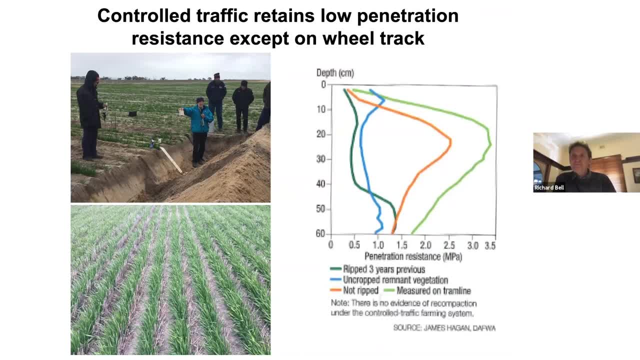 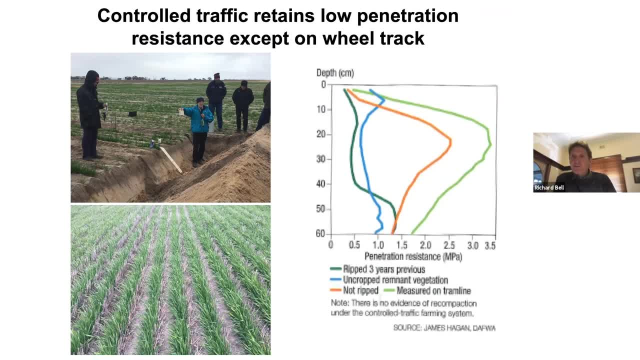 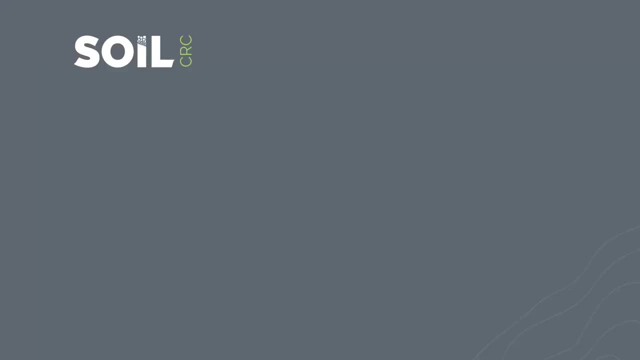 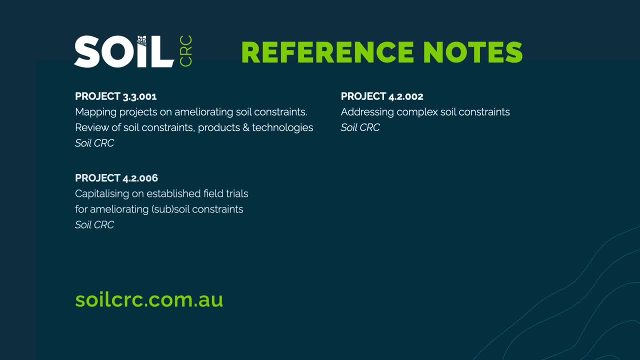 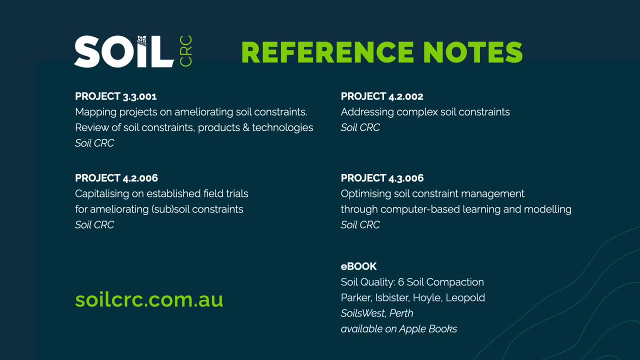 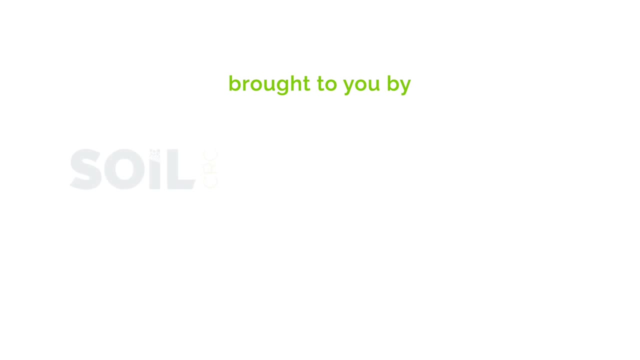 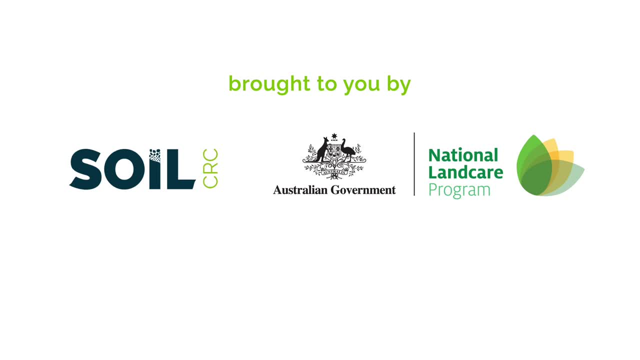 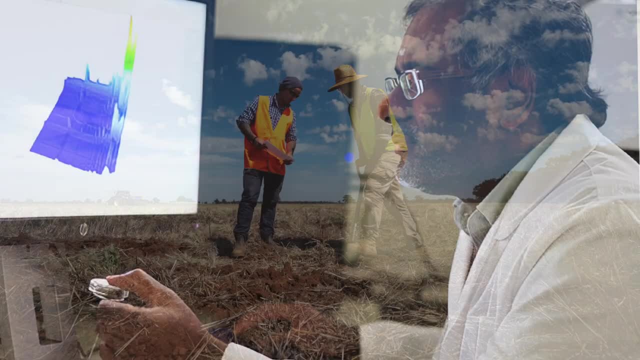